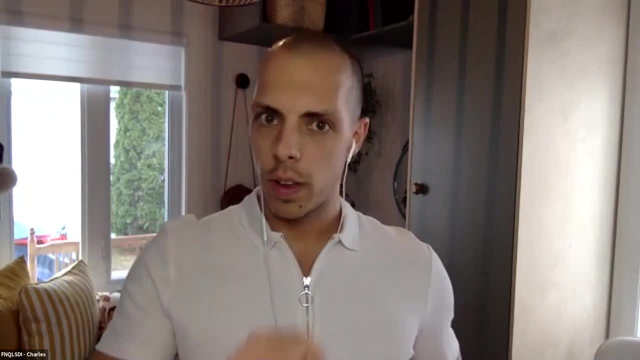 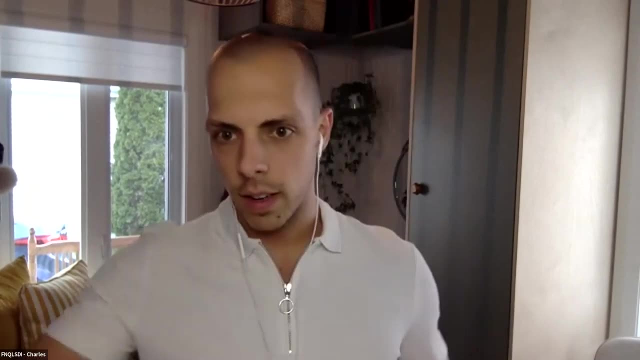 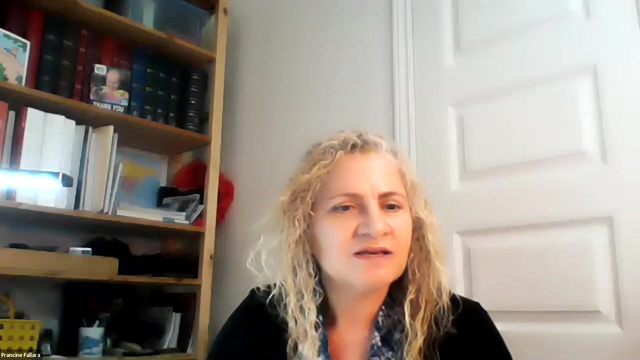 If you are watching the replay. as usual, send all your questions to info at iddpnqlca. Once again, that information goes to Francine and we get them answers right back to you Without further ado. Francine, the floor is yours. Thank you, So welcome to this new block. I'm going to share my screen. 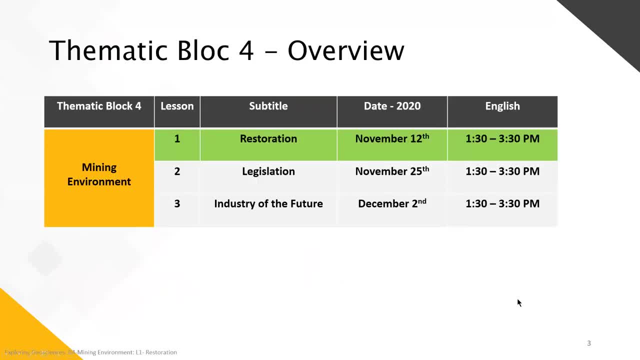 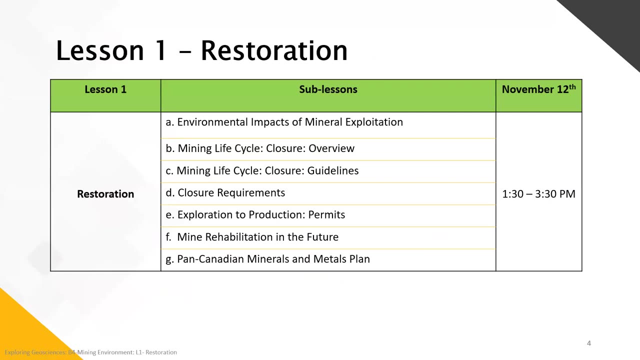 Voilà, We're good to take off, Thanks, Okay. so thematic block four. the true lessons are restoration, legislation and industry of the future. Restoration, separated into seven general subjects. I'll have a bigger part on the environmental impacts of the mineral exploitation. 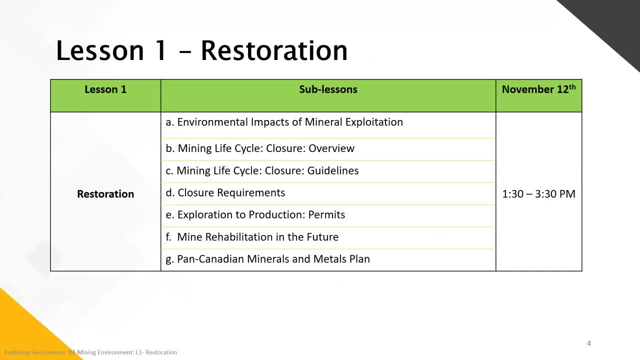 We'll fit that in within the mining cycle, the overview and the updated guidelines, The closure requirements, An example of exploration, two production projects- what kind of permits are needed, the mine realization in the future and the newest planned Canadian minerals and metals plan. 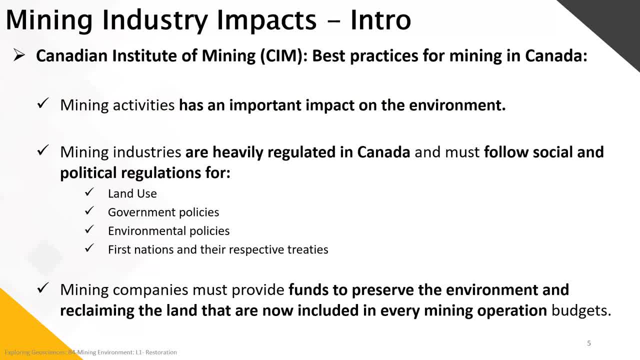 So to start, I went to get the CIM, the Canadian Institute of Mining- best practices for mining in Canada. This is a great guide for you to start and read, Also, for I've included to push out several PDF files. that regroups the official guide that I'm 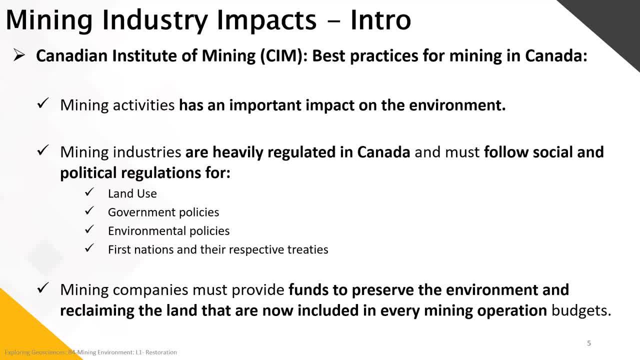 covering here today. So if you have any interest, you can have the PDF files, and I also included in this presentation all the website links if you want to go directly on the website. So mining activities has an important impact on the environment. Mining industries are heavily regulated in Canada and must follow social and political 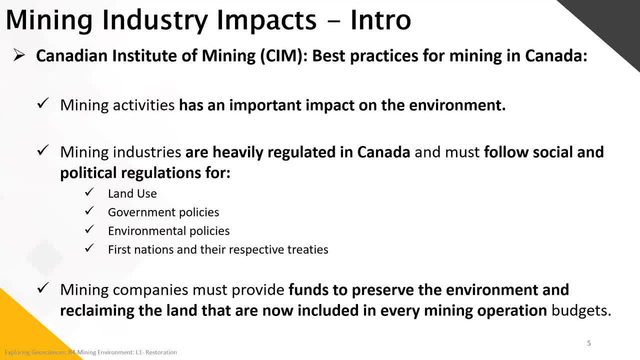 regulations. Contrary to what several people think, these regulations include the land use, many government policies, environment policies and First Nations and their respective treaties. Mining companies Must provide funds to preserve the environment and reclaiming the land that are now included. 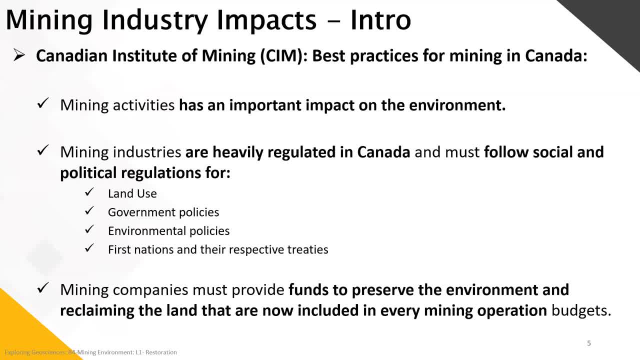 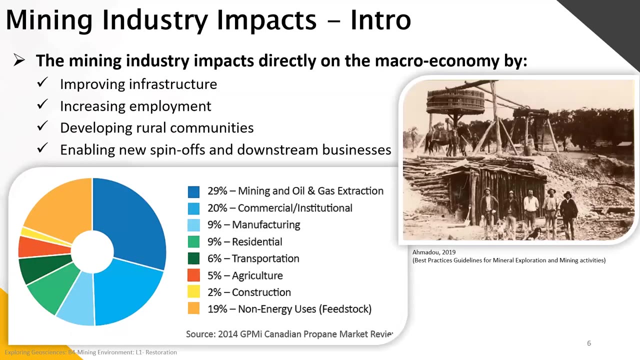 in every mining operation budgets. So many of the environment impacts horror stories we have seen from the past are now within the past because the industry is very heavily regulated to prevent any of these new horror stories. So the mining Industry impacts directly affects the entire micro economy as we know it. 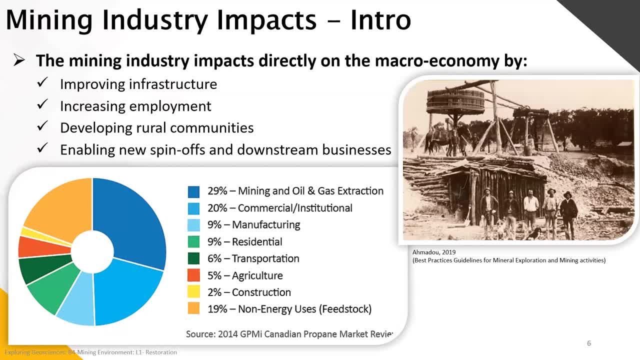 It has also some. we're talking about negative impacts, but we also need to talk about positive impacts. So some of these positive impacts are improving the infrastructure, increasing employment, developing rural communities, because a lot of the rural communities would not exist, or 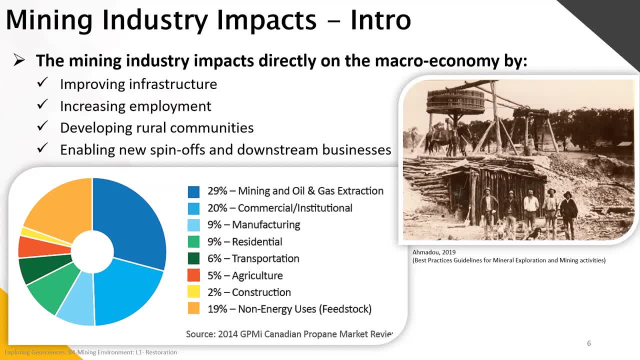 would live with Practically no jobs or any possible possibility to open or enable any new spin offs and downstream business. So mining industry has a lot of what we call direct and indirect impacts, both negative and positive. I've included here down here the main domains that the mining industry impacts, both positive and negative. 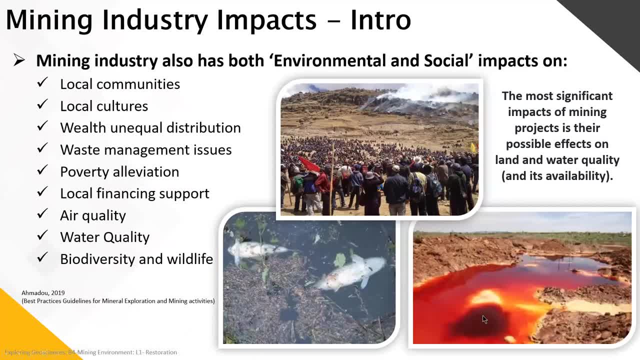 So most of these impacts are in what we call the environmental and social category, and these can include local communities, local cultures, wealth unequal distribution, waste management issues. It has, like I said, positive impacts like poverty alleviation, Local financing support. 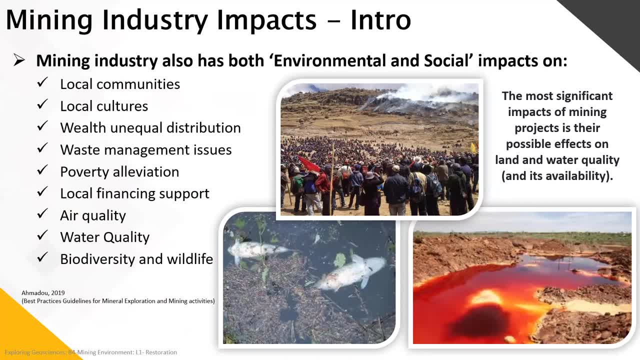 So these are the main ones: Housing, health, land development and natural resources, public support for either businesses, festivals, municipalities, development and so on. Air quality, water quality and biodiversity and wildlife. The most significant impacts of mining projects is they're possible effects on land and water quality. 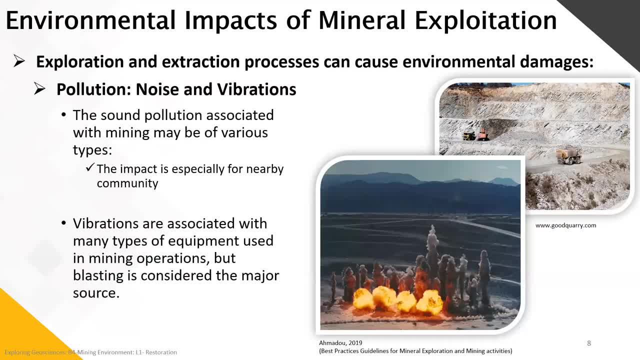 So the first part of my presentation. I've done a total list with examples of every project that I've done- Everybody I've done. So I started with two projects that I've done. So that's really easy. There's a lot going on. 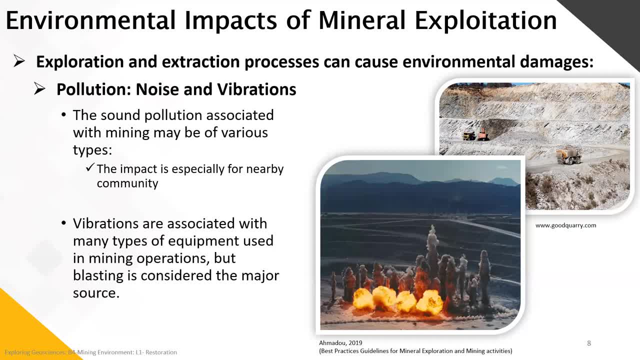 every kind of impact you can have, not just in Quebec, not just in Canada, but in the world. and it will show the processes, the main processes that can cause environmental damages, And I've also included some examples of how these can be controlled. So the first one: noise and vibration. 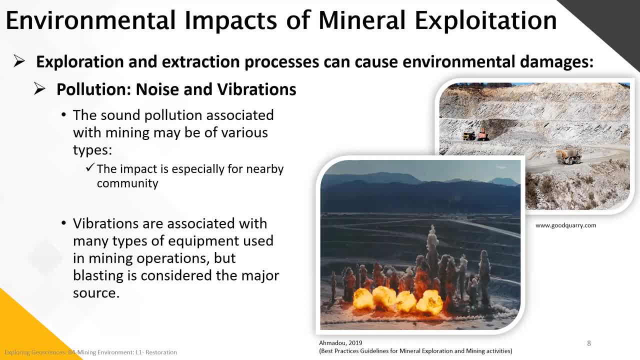 So the sound pollution-associated mining, maybe of various types, For example, the impact is especially for a nearby community. This has been lived by many communities in the Abitibi area, especially one of the later examples in the Malartic town. 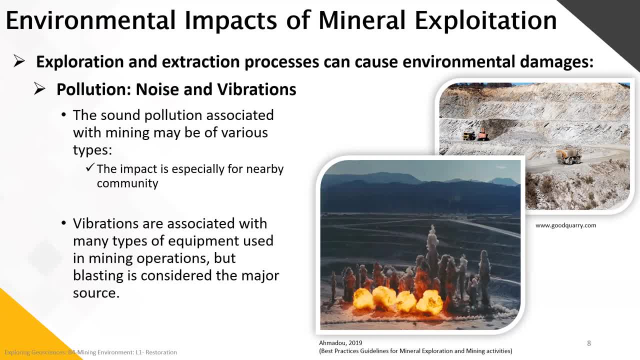 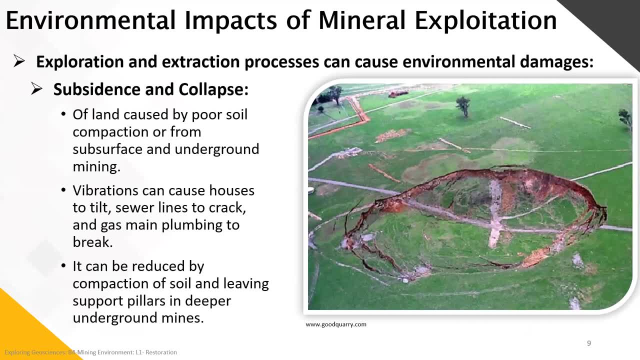 Vibrations are associated with many types of equipment used in mining operations, but blasting is considered the major source, and these impacts can cause what we call subsidence or collapsing. it's basically the land is collapses caused by poor soil compaction or from subsurface, and 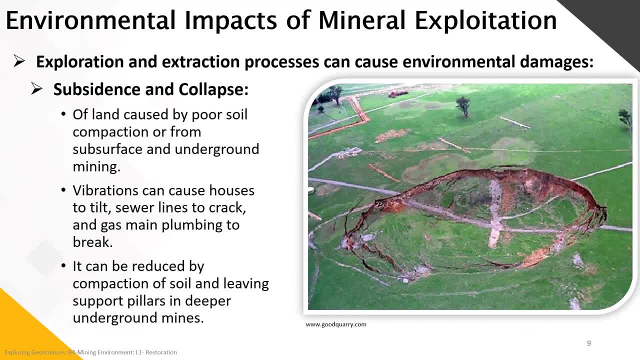 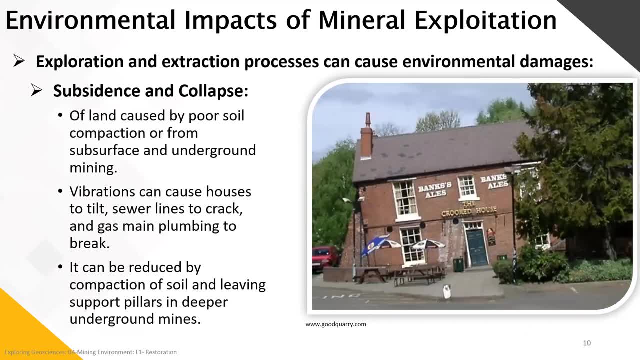 underground mining. the vibration can cause houses to fill, sewer lines to crack gas, main plumbing to break. here is a drastic example. it's not always as this bad um i'd move. i know some examples in the area before uh there, before the change of the open pit um in the town from uh to el dorado, um it was. 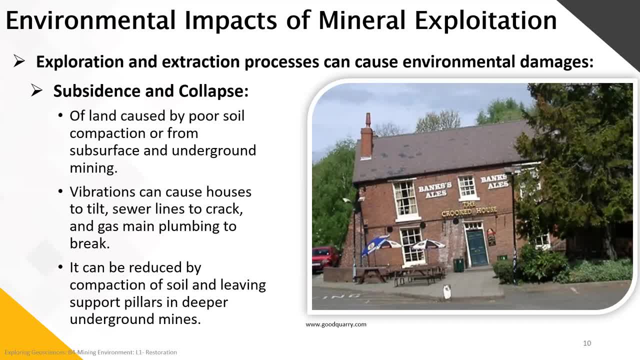 the first, i think it was century mining and many of the houses near uh would complain about uh by caused to vibrations, sewer lines and plumbing and etc. every time the mine would undergo uh blasting. this can be reduced by a good compaction of the soil and leaving support pillars and 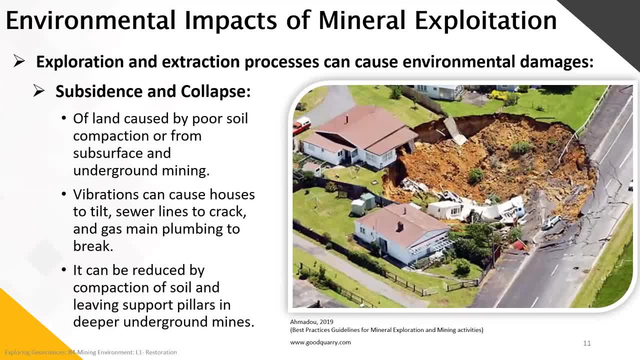 deeper underground mines, but also by planning um some of these blasts, um and making sure now that these buildings are not being destroyed and, for example, they're going to collapse on the way. and i want to say that this will be a big problem in the past, because the cities were not well 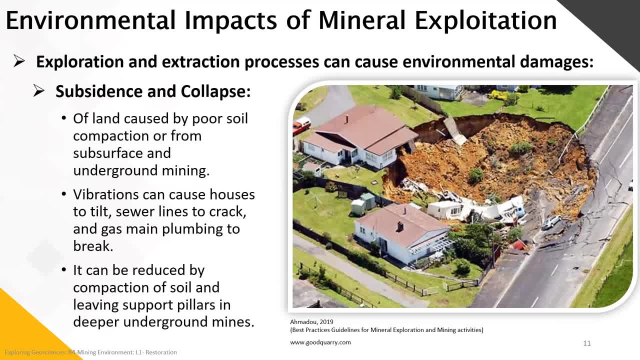 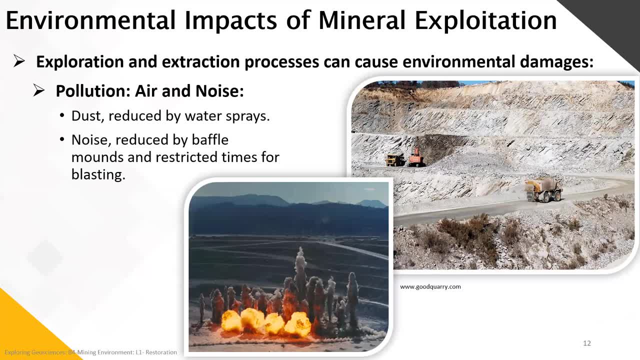 uh developed um. the infrastructures were not well developed so a lot of these houses were built too close to the mining site. this would not happen today. uh, for pollution, we also have air, air and noise pollution. so air, whatever Dust, can be reduced by water sprays. 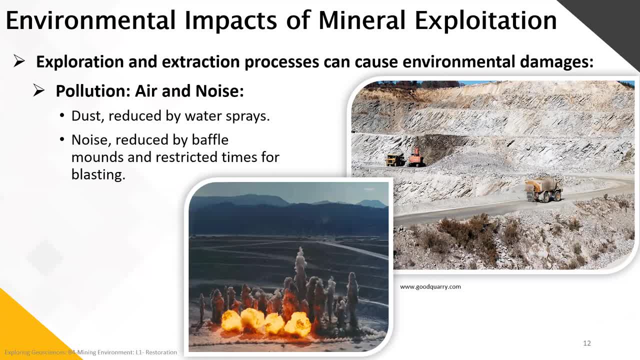 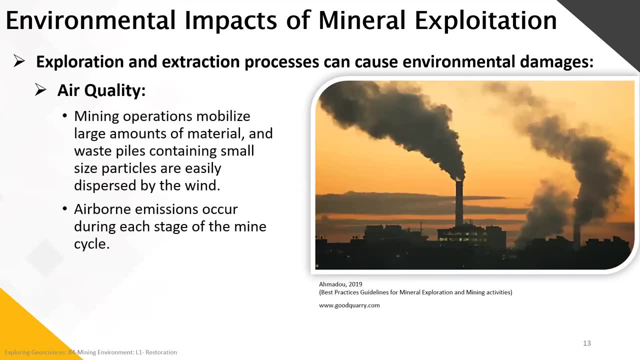 The noise. the noise can be reduced by baffle mounds and restricted times for blasting. A lot of the mines now don't blast all day long. They have restricted schedules to respect The air quality, while the mining operations mobilize large amounts of material and waste files. 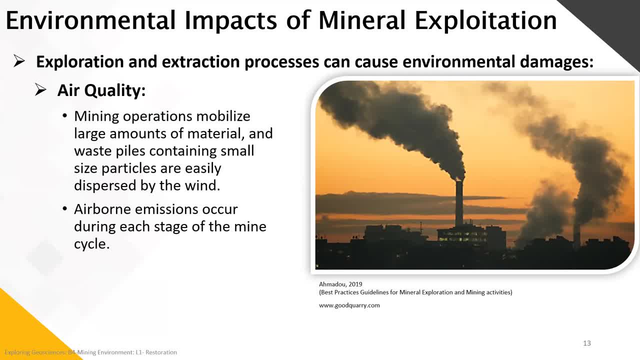 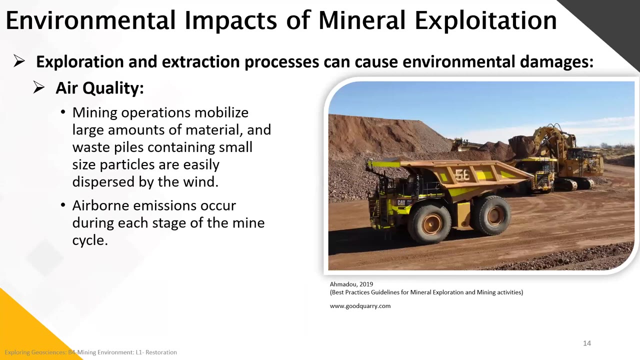 containing small size particles which are easily dispersed by the wind. Same principle as the natural volcano, the ashes would go around the air. same principle: Airborne emissions occur during each stage of the cycle of the mine cycle. The mining operations mobilize large amounts of material. 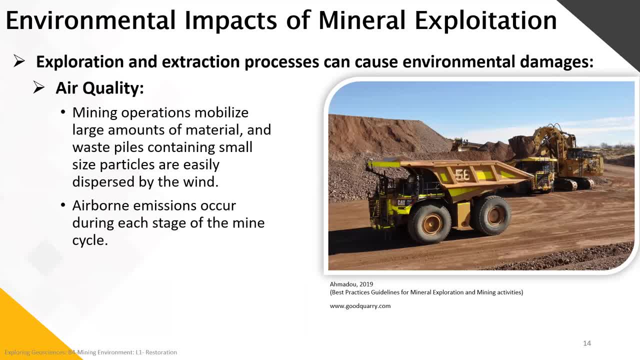 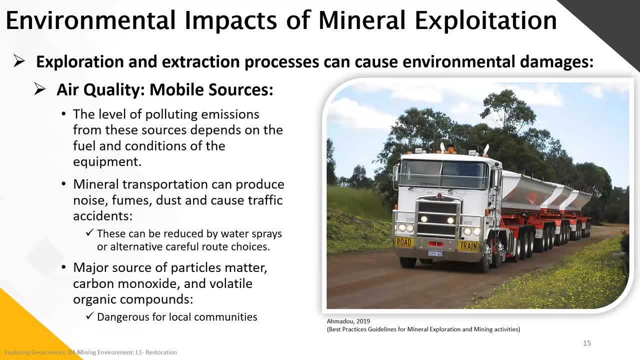 and waste files containing small size particles which are easily dispersed by the wind, And the airborne emissions occur during each stage of the mining cycle. We have two types of air quality that can be damaged by either mobile sources- mobile sources, So the level of cooling emissions from these sources. 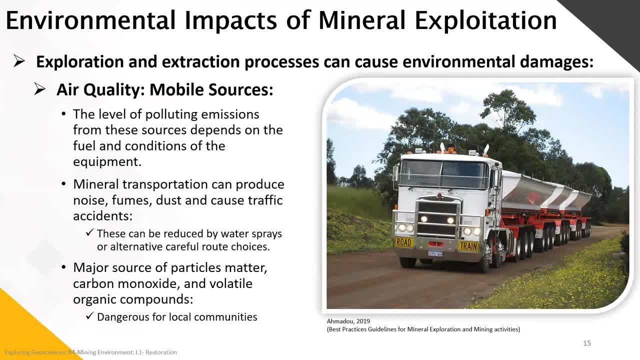 depends on the fuel and the conditions of the equipment. Mineral transportation can produce noise, fumes, dust and cause traffic accidents, can, most of the time, be reduced by either water sprays or by mines or mine projects, creating alternative route choices that they will build for their own product transport. 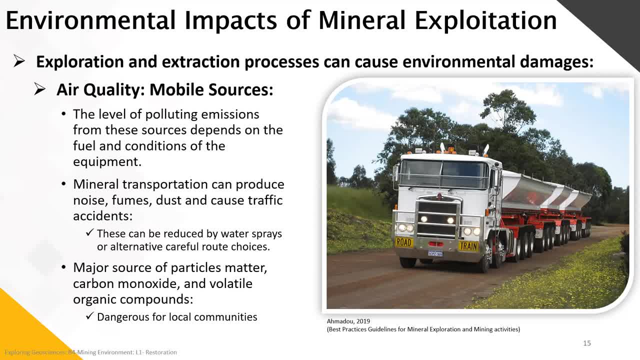 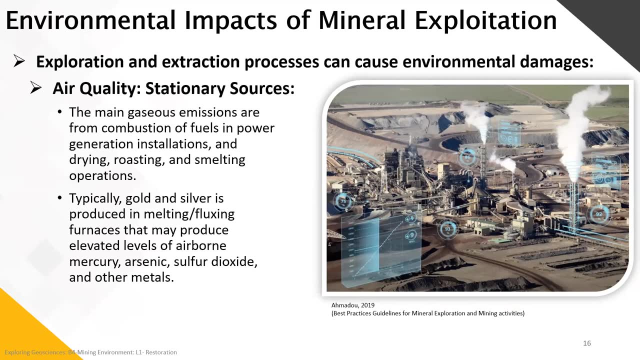 Major source of particles. matter like carbon monoxide and volatile organic compounds can be dangerous for local communities. We have the stationary source. Well, the stationary sources are basically within or on the mine development site. so the main gaseous emissions are from combustion of fuels and power generation installations and drying, roasting and smelting. 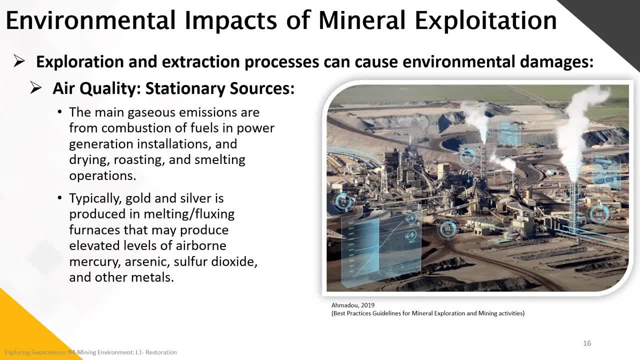 operations like any other manufacturer domain company. Typically for gold and石 it's nine: 00 And gold and zinc: 00 And gold and zinc: 00 And gold and zinc. Silver is produced in melting or fluxing furnaces so that may produce. 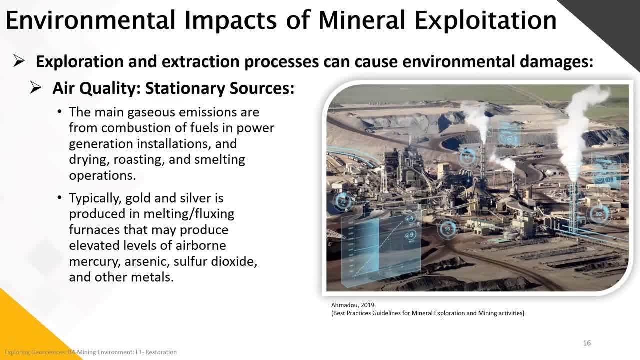 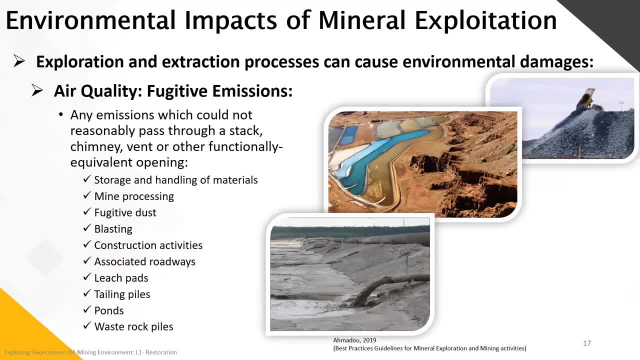 elevated levels of airborne mercury, arsenic, sulfur dioxide and other metals. We also have what we call the fugitive emissions. Fugitive emissions are sporadic, random, and these are the ones we need to watch out for, because sometimes they happen. 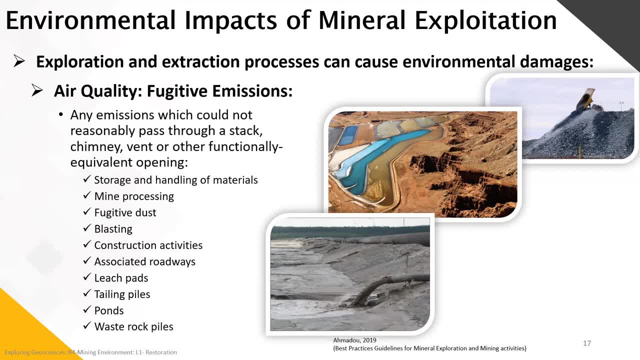 after several months, after several years. so we need ongoing studying of these emissions. So these regroup any emissions which could not reasonably pass through a stacked chimney, vent or other functionally equivalent opening like storage and handling of materials, processing future dust blasting, construction activities, associated roadways, leach pads. 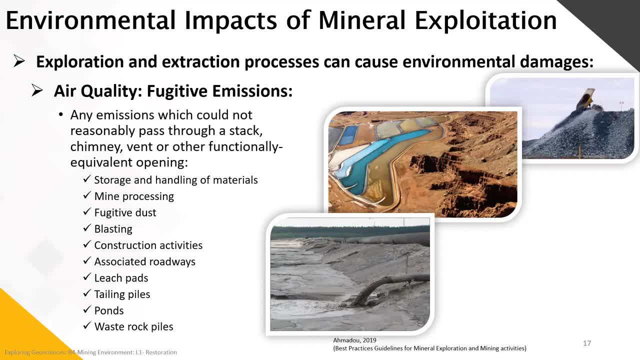 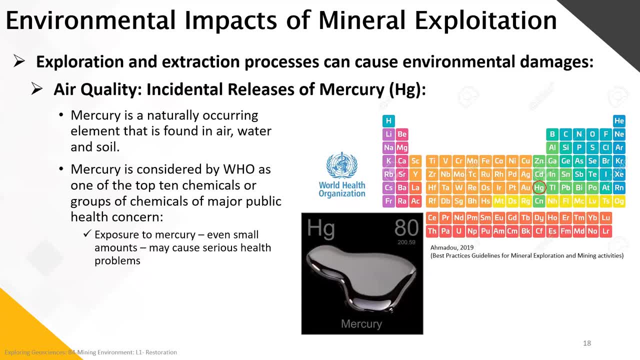 tailing piles, ponds and waste rock piles. The air quality. one of the major incidents is the release of mercury. The mercury is a natural occurring element that is found in air, water and soil, So just opening a bracket here. from now on in my presentation you'll see that a lot. 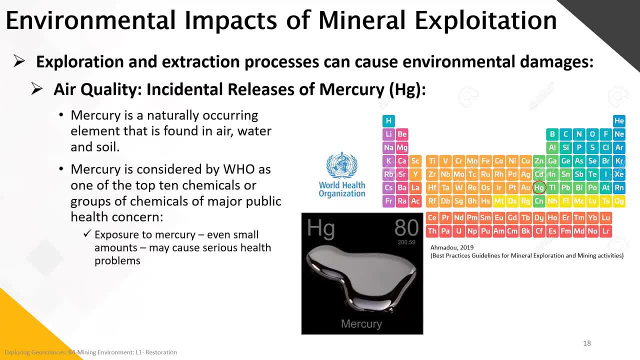 of the environmental damages are caused, ironically, by natural elements. So most of the mining pollution is caused by the mix of natural elements which react chemically with the environmental elements where it is stored, And this, unfortunately, is a chemical process that, if it is not well monitored, will develop. 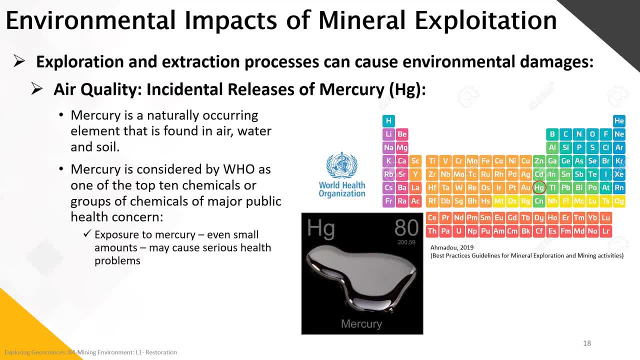 So the companies always have their own environmental department now to do the follow-ups, before a wild mine is ongoing and at the closure. So coming back to mercury, mercury is considered by the World Health Organization as one of the top 10 chemicals or groups of chemicals of major public concern. 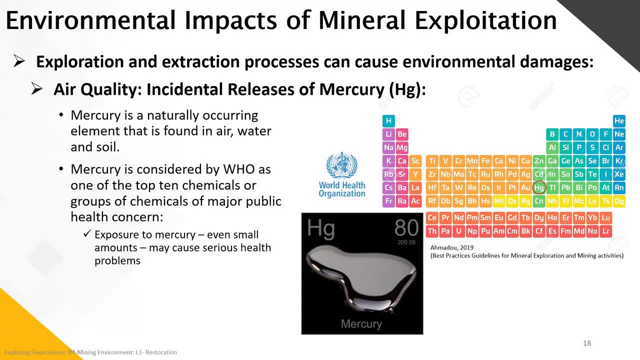 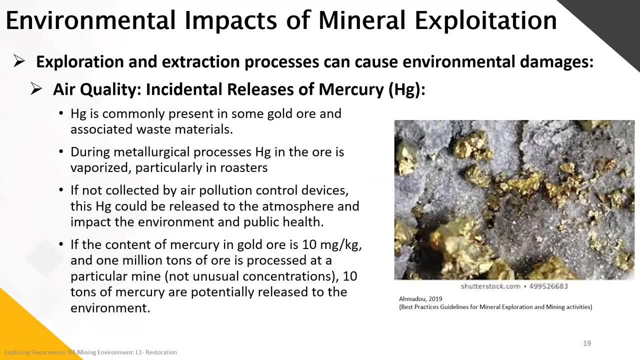 Too long exposure to mercury, even small amounts, may cause serious health problems. Mercury is commonly present in some gold ore and is associated, and therefore is associated in waste materials. Ironically, mercury is one of the trace indicators for when researching gold. During metallurgical processes, mercury in the ore is vaporized, particularly in roasters. 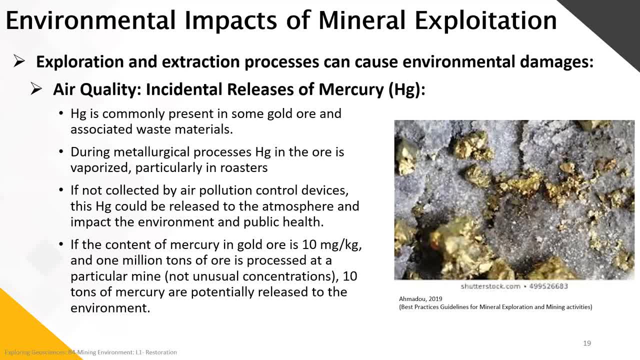 If not collected by air pollution control devices, this mercury could be released to the atmosphere and impact the environment in public health. An example is for mercury in gold ore for 10 milligrams per kilogram and 1 million tons of ore processed in. 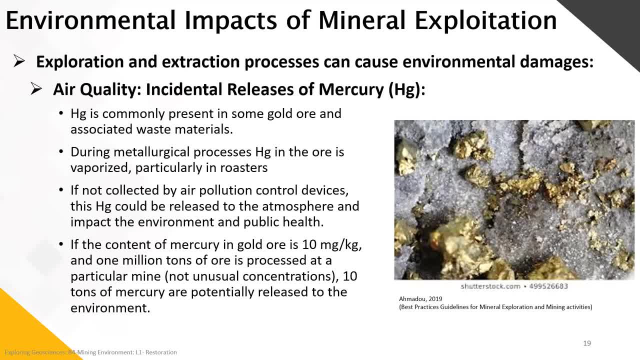 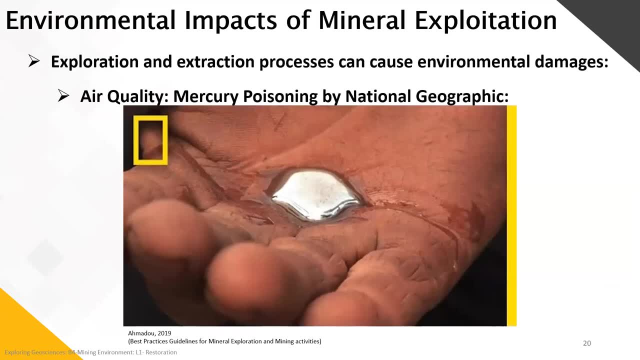 a particular mine, which is a usual concentration, we would create 10 tons of mercury which it would potentially be released to the environment if it was not well monitored. I have included the National Geographic video showing mercury production, Mercury poisoning. I'll let you look at it at your own time. 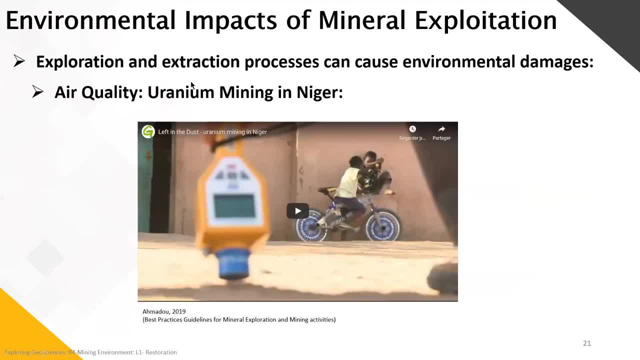 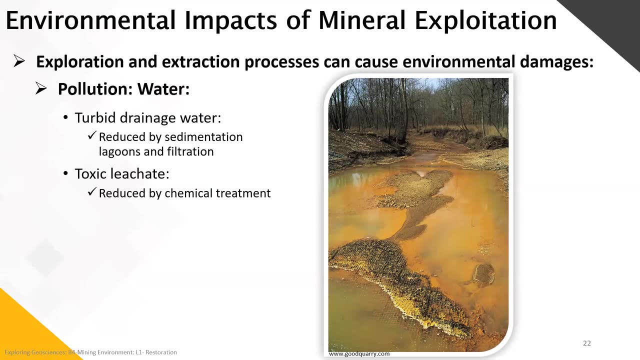 And I also included another video- for the Iranian uranium mining in Niger and the air quality it has caused. So, moving on other type of pollution, moving on from air and noise, we're moving on to the next important one, which would be wine. 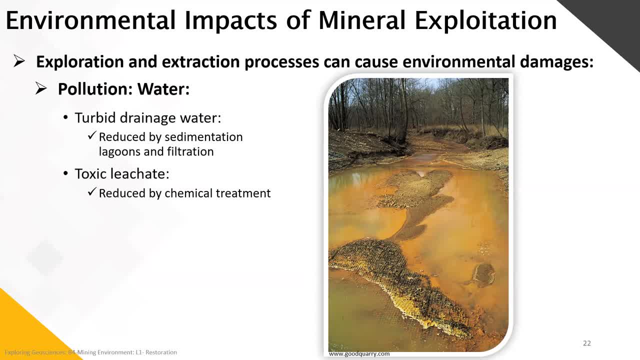 And this is a very important one- which would be water, and mainly it is like a turbid drainage water. so this can be reduced by sedimentation lagons and filtration. Most of the water pollution again is caused by the mix of a chemical reaction between 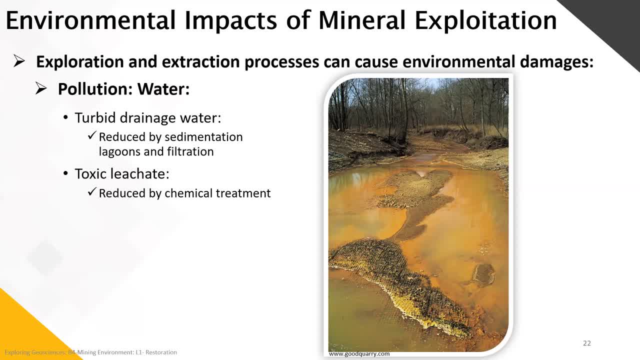 two groups of natural elements combined together will create this pollution by their chemical process. Unfortunately, toxic leachate can be reduced by chemical treatment. So that is why now all mining projects and sites have their environmental department to do all these follow ups and checkups before they occur and, if they occur, to get them right at the start. 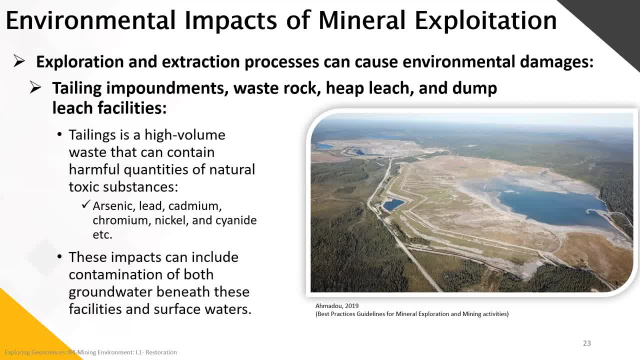 Tailings and impoundments, waste rocks, heat leachate and dump. dump leach facilities are also a big checkup. Tallings is a high volume waste that can contain harmful quantities of natural toxic substances. Again, these are all natural, coming out of the 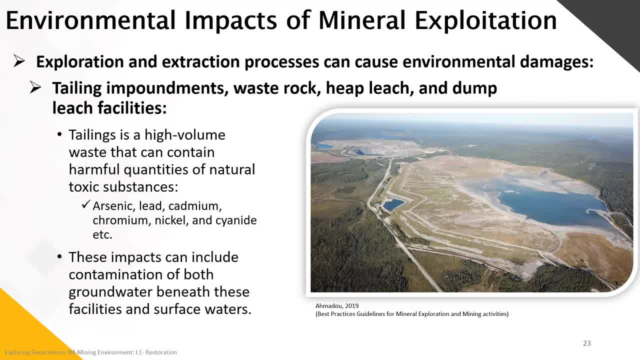 rocks, arsenic, lead, cadmium, chromium, nickel, cyanide, etc. These have to be watched out in the tallings sitting there and not chemically reacting with the environment, So material to make sure that these impacts can include both contamination of the prevent, contamination of groundwater. 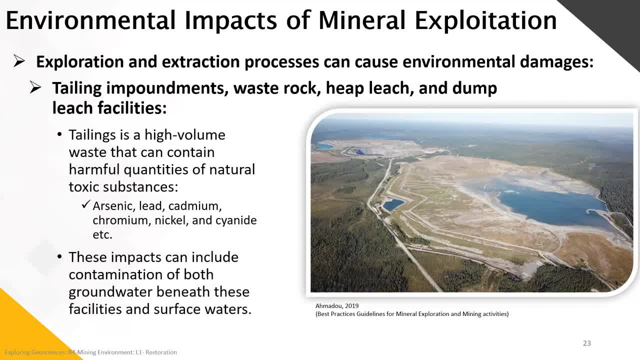 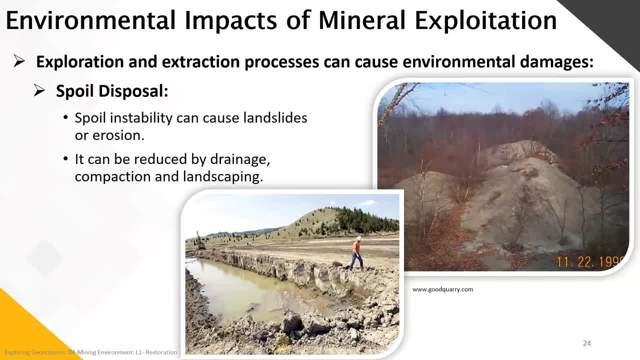 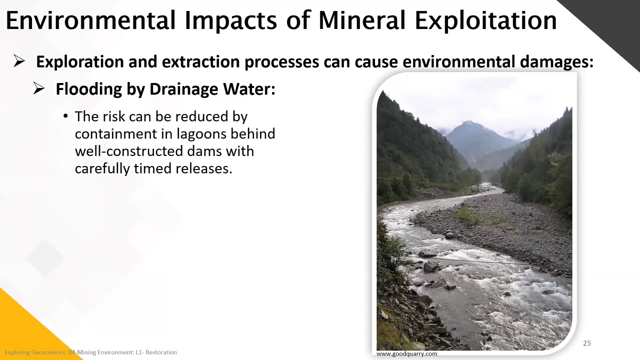 beneath these facilities and also surface waters. Spoil disposal is another of the goals. This can be reduced by drainage compaction and landscaping Flooding by drainage water. the risk can be reduced again by containment in lagoons behind well-constructed dams with carefully timed 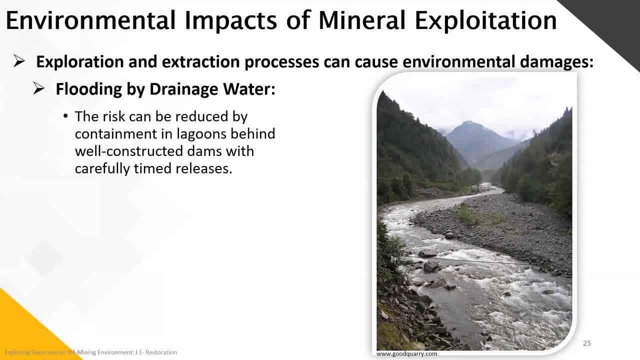 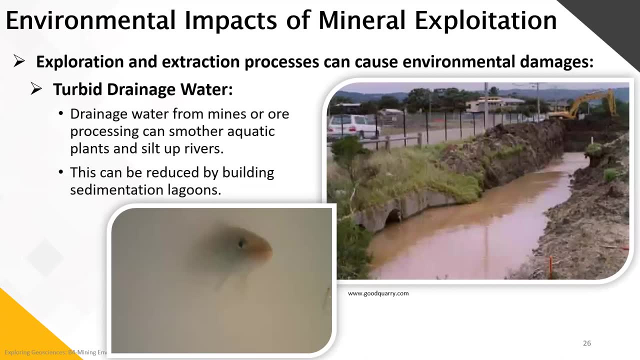 releases To make sure that it doesn't make any natural water to flood. Turbid drainage water from mines or ore processing can smother aquatic plants and silt up rivers. So to prevent again here. this is a natural process. It is the silt coming out of the water, very fine grain that will, if not filtered out. 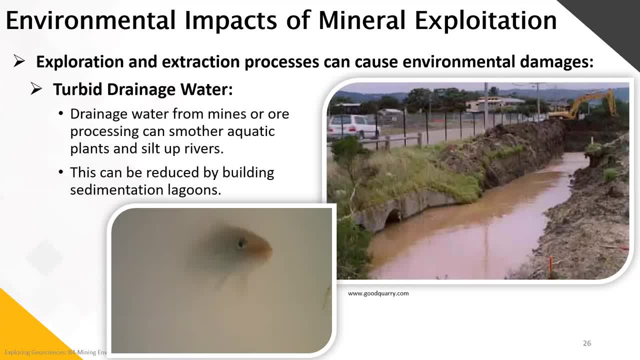 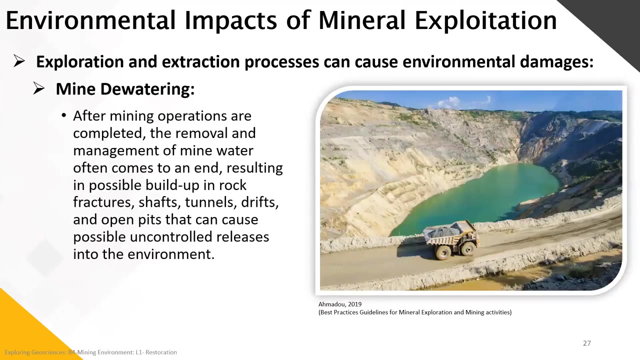 that will cause turbid waters. This turbid water can be dangerous for the living fauna. This can be reduced beforehand by building sedimentation lagoons for the silt to sediment and let the rest of the water out of the system Mine dewatering. So if an open pit or underground mines are closed or temporarily closed, 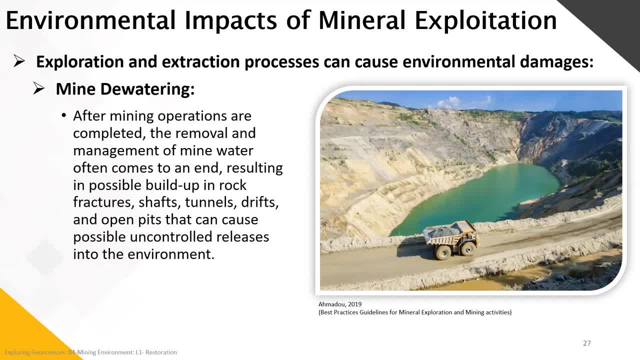 or put on standby, like we've seen in the previous lessons. for many causes, like a lack of money, the metal we are mining the commodity, the price is going down, so the company is putting it on standby. If it is not well guarded and looked upon well, the water will pile up either in the open pit, 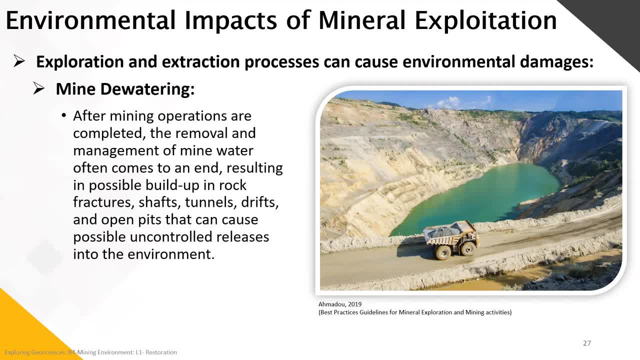 or the underground drifts and so on. So this water, once the mine is going back into production, needs to be taken out. So, after mining operations are completed, the removal and management of mine water often comes to an end, and this can cause big environmental damages, resulting in possible 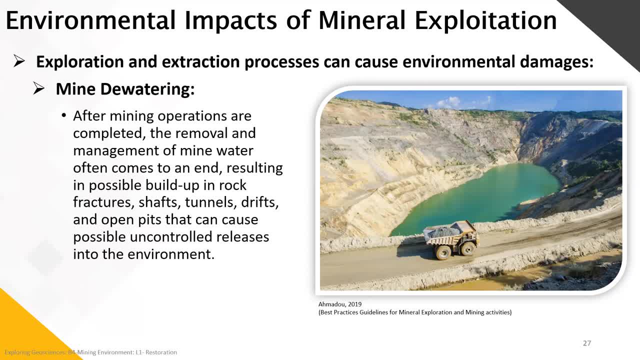 buildup in rock tractors, shafts, tunnels, drifts. We also have toxic leachate through wind and water, So the wind carries by erosion toxic mining waste which can go in food webs and watersheds. Water draining from spoiled heaps may contain toxic metals. 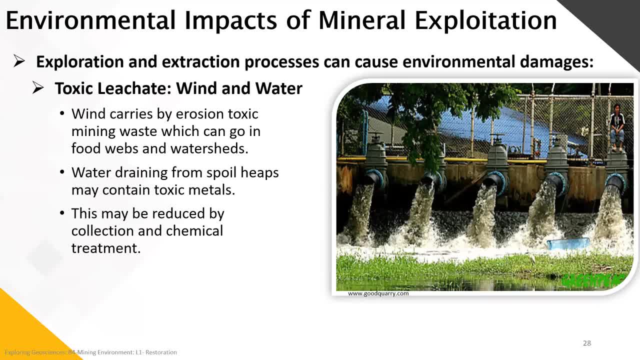 This may be reduced by collection and chemical treatment. So this is an example of an open pit and this is an example of an open pit, and this is an example of an open pit and that can cause possible uncontrolled releases into the environment. 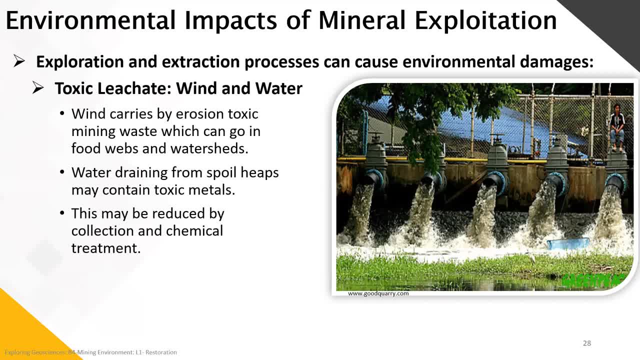 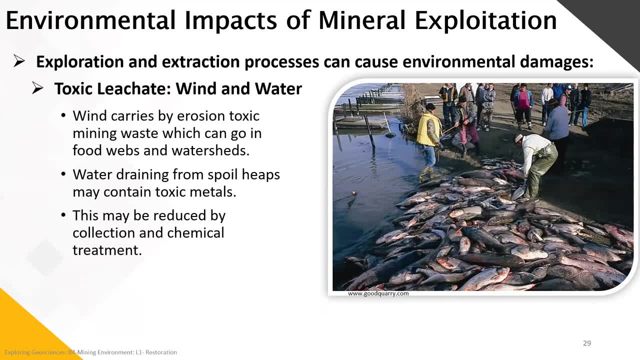 We also have toxic leachate through wind and water: Wind carries, by erosion, toxic mining waste which can go in food and watersheds, as I said before. Example here is within the water and we've seen that sometimes we have like the actual fauna being. 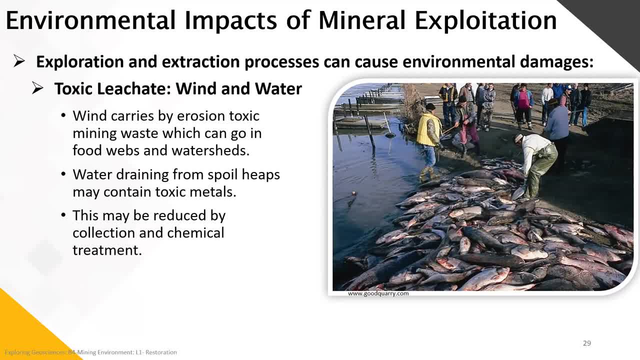 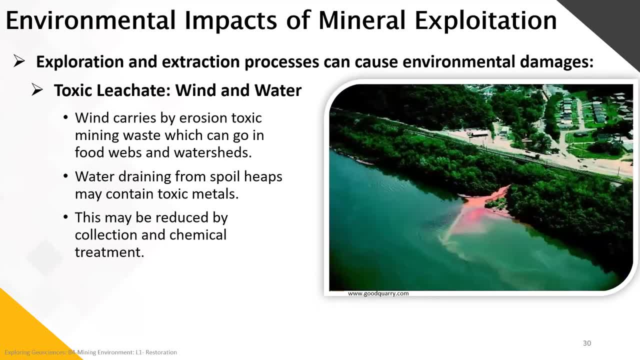 intoxicated by these toxic leaches. So these are not toxic leachates, but these are toxic leaches and they are found in the water Sample here. toxiflecia of water and, again, natural phenomena, with the chemical process of oxidations of iron rich, either soil or water just being oxidized by the air and the 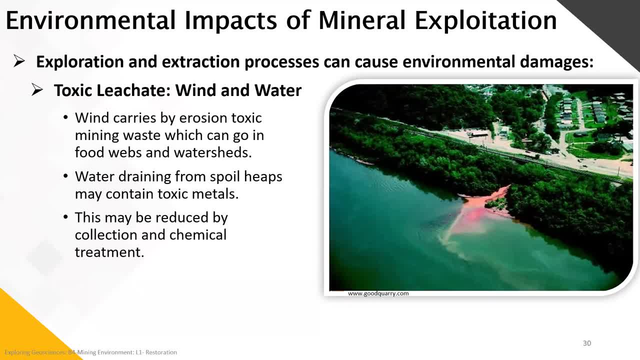 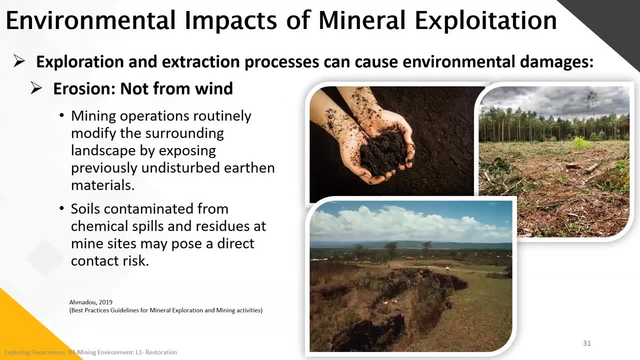 reaction causing the red waters. We have another environmental damage classified under erosion, but not a natural erosion, not from wind, but man-made erosion, and this happens often within mining operations, which are which are literally modify the surrounding landscape by exposing previously undisturbed urgent materials. 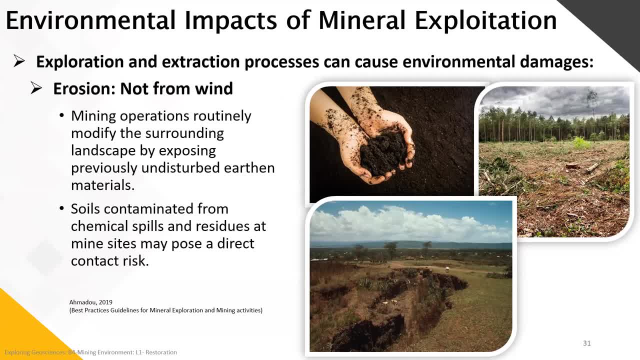 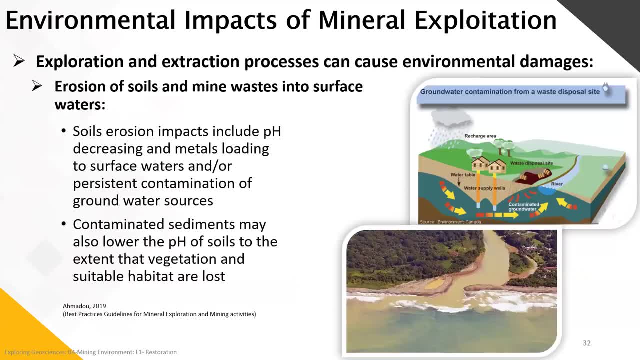 The soils contaminated from chemical spills and residues at mine sites may cause a direct contact risk, The erosion of the soil and the mine waste into surface waters. The soil erosion impacts include the pH decreasing, which means going into the acidic environment, and metals loading to surface waters, and or persistent contamination of groundwater sources. 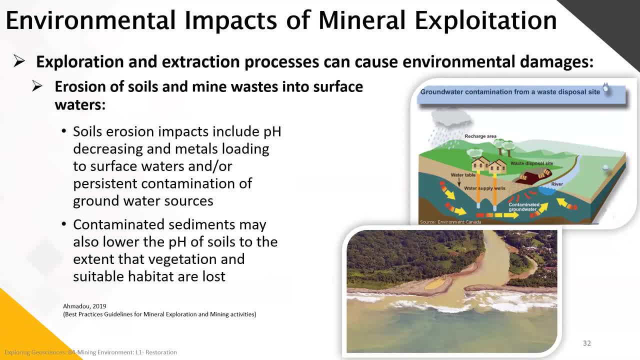 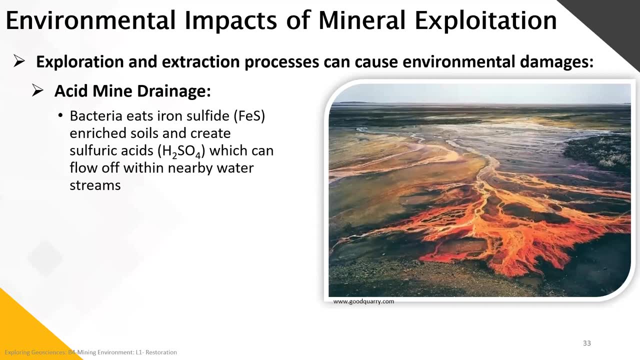 Contaminated sediments may also lower the pH of soils to the extent that they can cause a direct contact risk. Residues from polluted soil, vegetation and suitable habitat are lost because the environments are becoming more and more acidic. So we have what we call the acid mine drainage, the AMD. 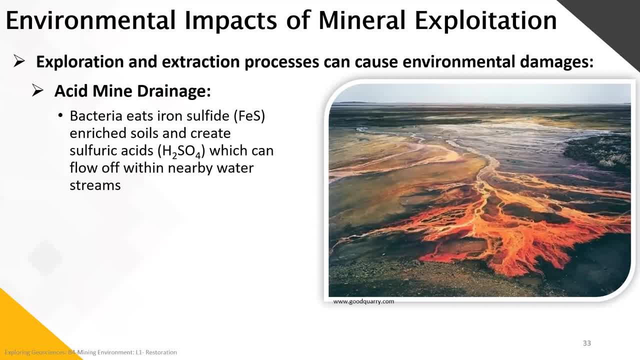 Because then we'll see a little bit later on- but mainly from bacteria which is carbon sulfide, yes, which in the rich soils- and we'll create the sulfuric acid- grabs Any moisture, do its job. And this is an example: the SME. 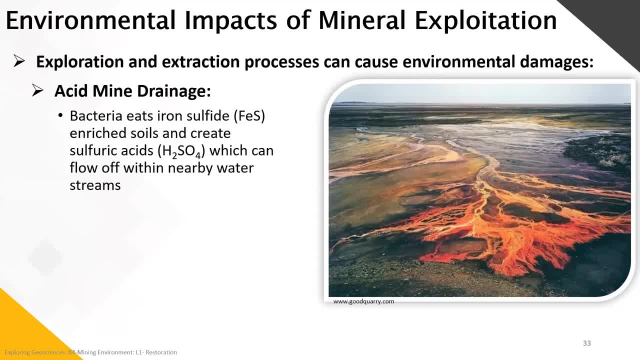 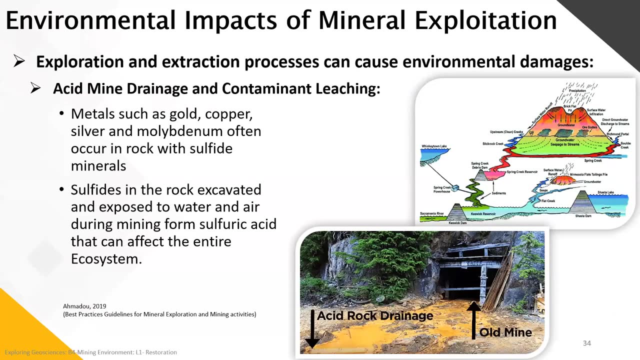 H2SO4,, which can flow up within nearby water streams if not contained, if not well contained, and that was one of the major problems from mines of the past: The acidic mine drainage and contaminant leaching metals such as gold, copper, silver and molybdenum. 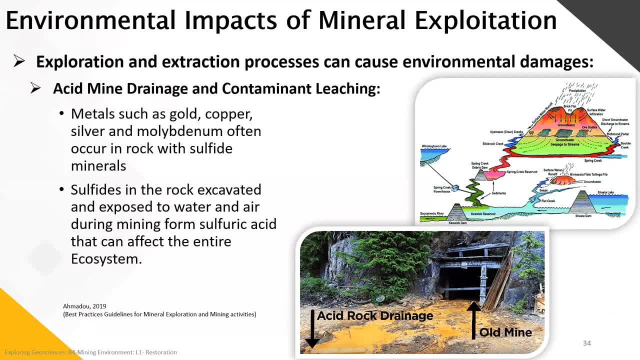 often occur in the rock with sulfide minerals. These sulfides in the rock excavated and exposed to water and air during mining form sulfuric acid. that can affect the entire ecosystem and that was one of the major, major impacts of our unfortunately, historical overmines. 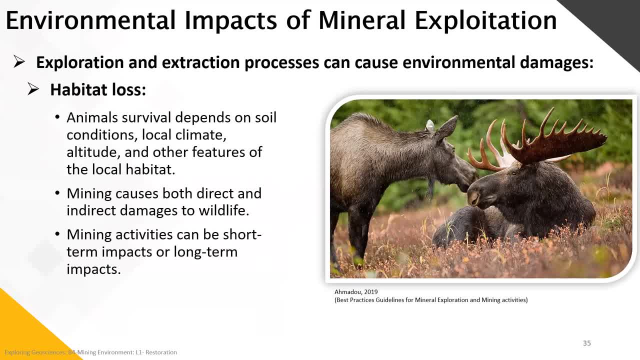 If we move on within the habitat loss category for environmental damages, we have animals' survival That depends on the soil conditions, the local climate, the altitude and other features of the local habitat. Mining causes both direct and indirect damages to wildlife. 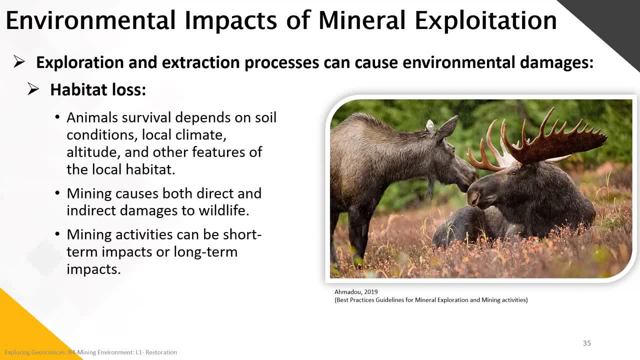 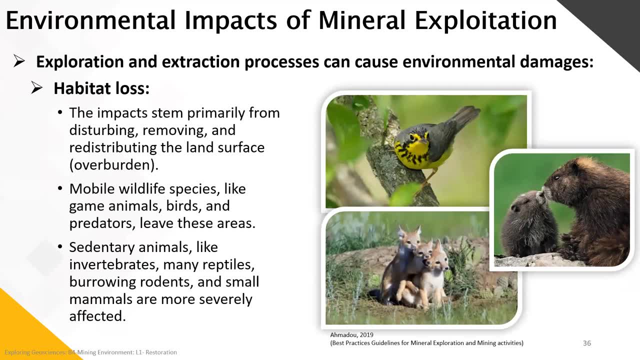 Mining activities can be short-term impacts or long-term impacts, depending on how these are taken care of. from the beginning, The habitat loss. the impacts stem primarily from disturbing, removing and redistributing the land surface. It can be called the overburden. 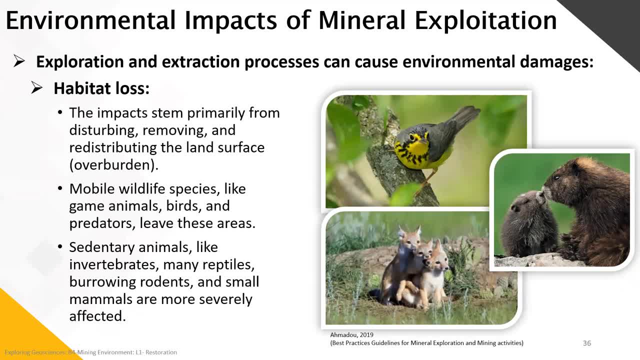 The overburden can be called the overburden, As we saw, while that will affect both mobile and sedentary animals, but the mobile and wildlife species. they have the advantage, like game animals, birds and predators, to leave the areas. 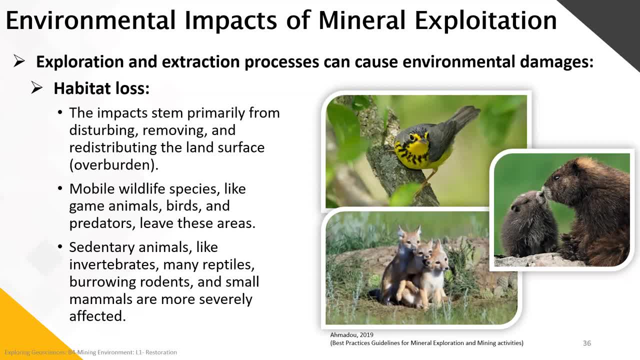 Mostly, they will just move on. The sedentary animals, them like the invertebrates, the reptiles, the rodents and smaller mammals. they will be the most affected because they are the ones that stay. They are the ones that stay in the area. 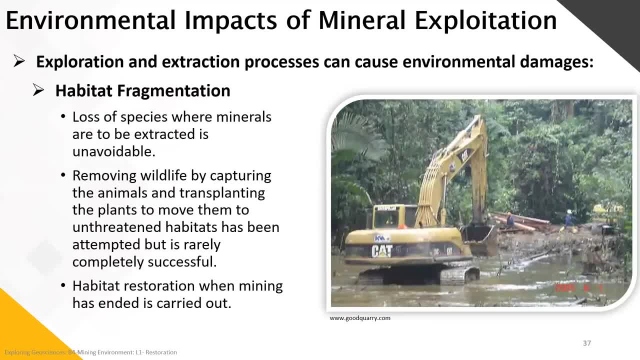 We also have what we call the habitat fragmentation due to man machinery. This also affects a lot fauna and flora, causes loss of species where minerals are to be extracted, which is unavoidable, Removing wildlife By capturing the animals and transplanting the plants to move them to untreated habitats. 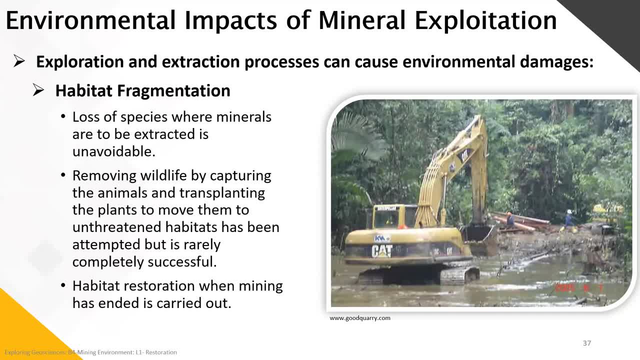 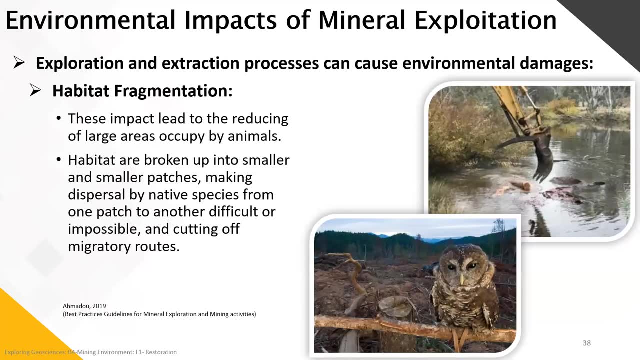 has been attempted in the past, but the rate of success has been very low. Habitat restoration when mining has ended is carried out, and that mostly works better than moving the habitat. The habitat fragmentation impact leads to the reducing of large areas. 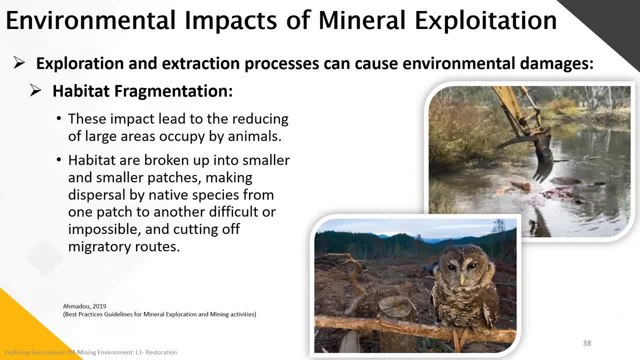 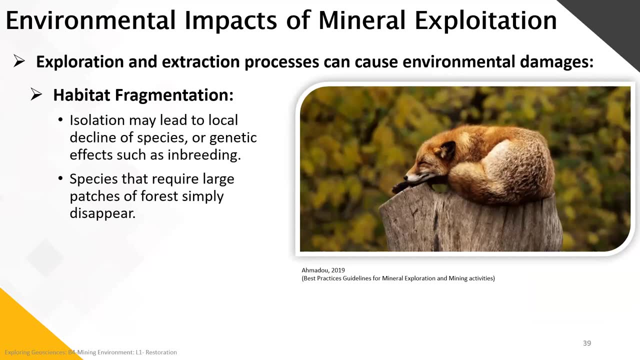 The habitat fragmentation can also cause isolation, which may lead to local decline of species or genetic effects such as inbreeding. The habitat fragmentation can also cause isolation, which may lead to local decline of species or genetic effects such as inbreeding. 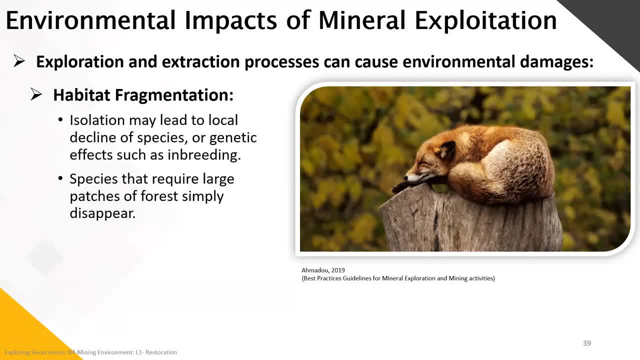 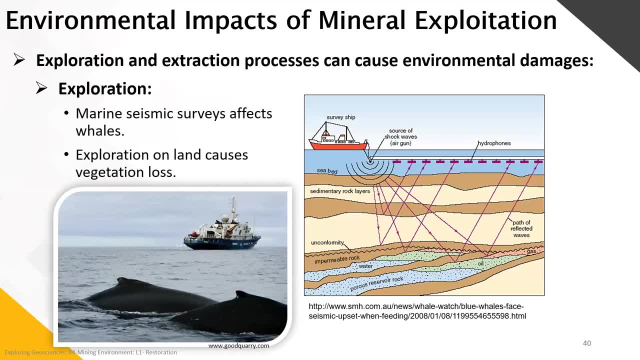 And we also have species that require large batches of forests And if they don't have that, they simply disappear. Just to complete with the other lessons we saw, I wanted to also show environmental damages for the marine exploration. So marine exploration is mainly done searching for new deposits. through what we saw yesterday, 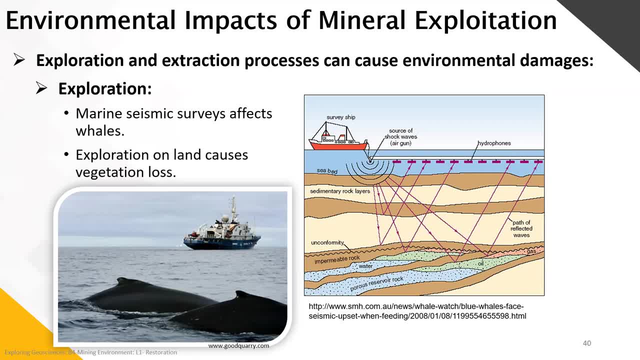 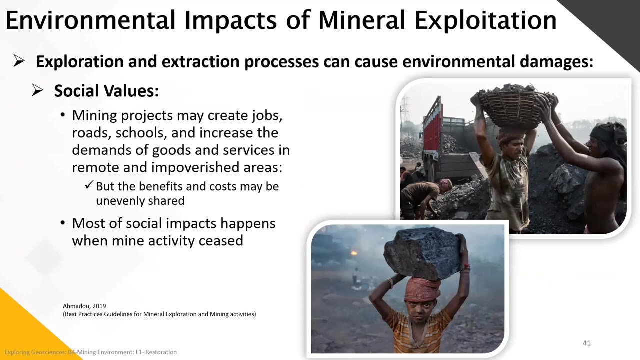 the marine exploration saw the geophysical seismic surveys and these directly impact the whales so and they cause a lot of um a lot of these exploration surveys cause a lot of land and vegetation loss for social values. so that is another major branch of environmental damage um social values. 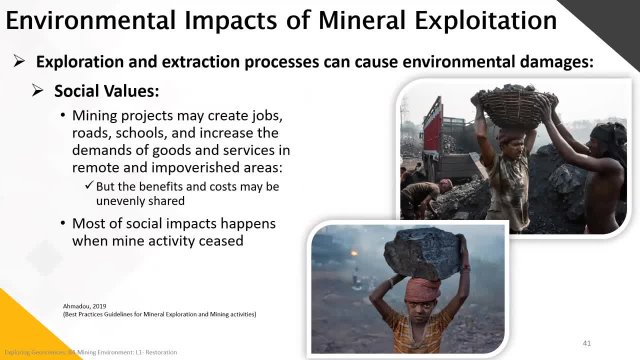 damages vary from developed to underdeveloped countries. um mining projects may create jobs, roads, schools and increase the demands of good goods and services in remote and impoverished areas, but um within mostly underdeveloped countries, the benefits and costs may be unevenly shared, unfortunately, and so the local population, who is mainly working on the mining projects. 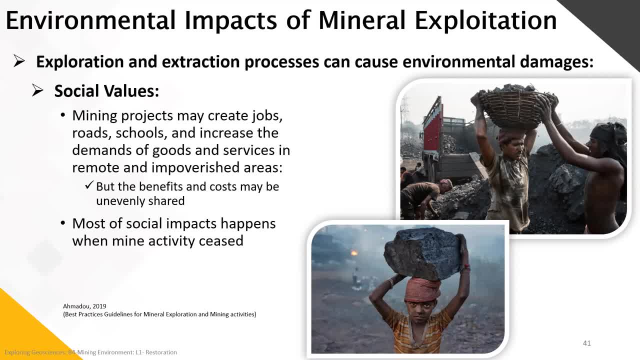 are not working in these mines are not really improving their lives. most of social impacts happens when mine activity uh ceased. when they are gone in these areas and countries we have a double impact on these societies uh. they lose completely any uh sense of work or impossible employment, and these people are 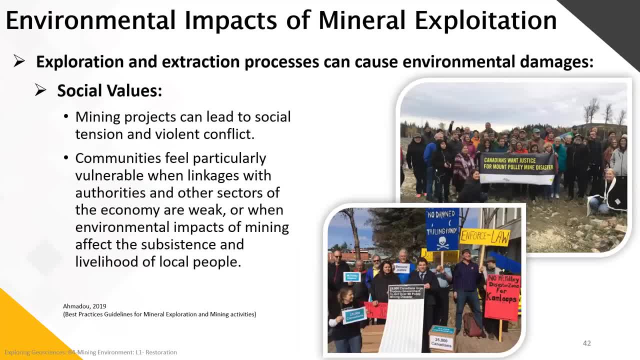 uh are left to themselves. mining projects can lead to many social and violent uh tensions, conflictual tension. communities feel particularly vulnerable when linkages with authorities and other sectors of the economy are weak or when environmental impacts of mining affect the subsistence and the view of local local people. this happens a lot within the um. 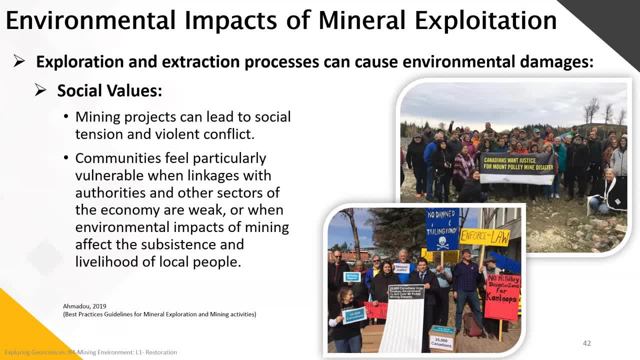 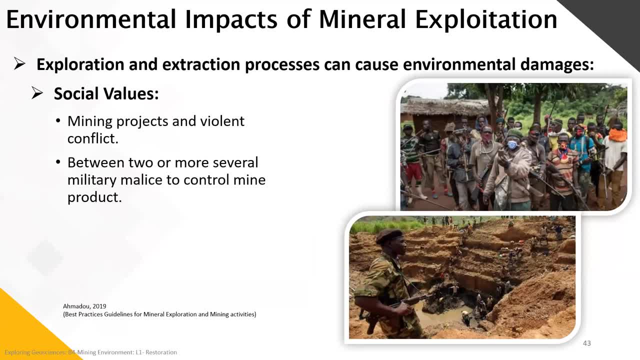 southern america and african uh mining science. we have also um, like i said, the main mining projects and violent conflicts and between two or several military values control the mine product. so that's also a question of power, power inequality within these countries which can cause a major social conflicts. so 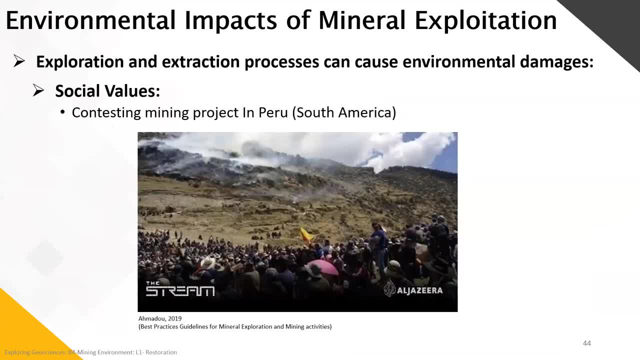 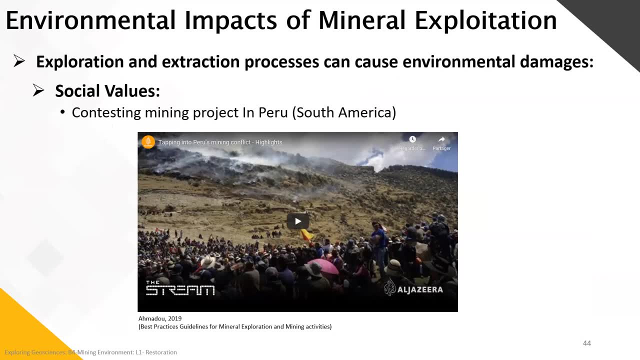 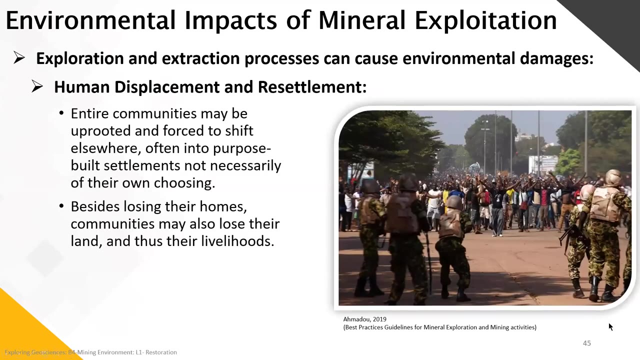 um, i have included a video showing one of the greatest mine protestation into the peru country, within south america, showing the social uh environmental damages of the area. another big social impact is when we have the uh what is called human displacement and resettlement uh, when we have entire communities which can be uprooted and forced to shift. 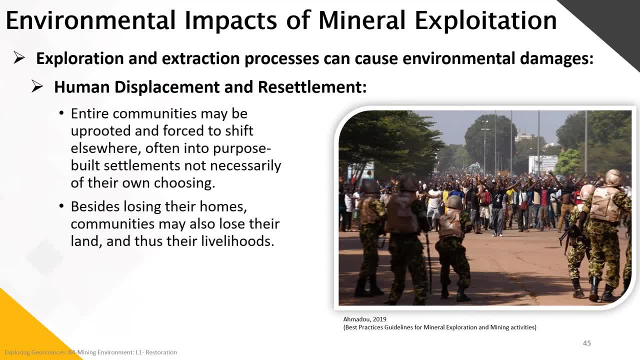 elsewhere to move, uh often into purpose uh built settlements, not necessarily of their own choosing or liking um besides losing their homes, communities, they may also lose their land, their culture and their livelihoods. these are made major um importance. we see them less in quebec and in canada, but we have seen them uh. one good example is: 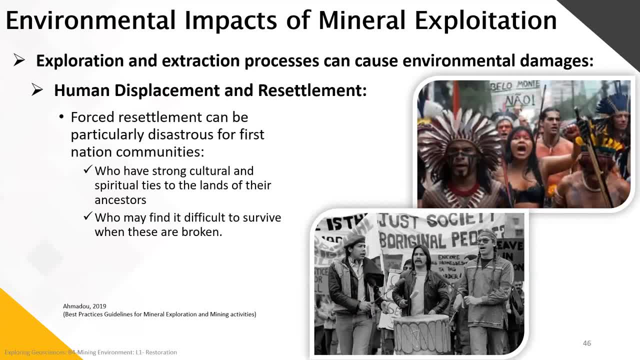 in the balartic town. uh, these forced resettlement can be particularly disastrous for first nation communities. uh, as we've seen a lot in south america, in africa, but also we've seen some in canada and the united states who have strong cultural and spiritual ties to their communities. 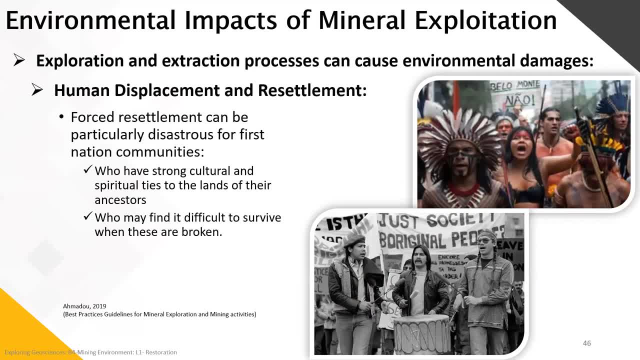 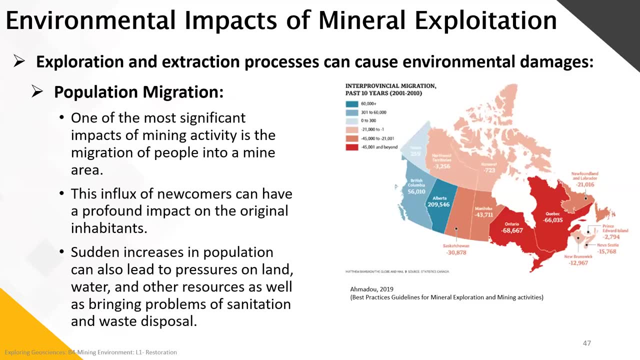 to their lands and their ancestors and who may find it difficult to survive when these are broken. and this happens, unfortunately, more within the underdeveloped countries. example here, within our country, within canada, of how population migration can affect, even if, um, the mine is opening and we have big population migrations because people are going. 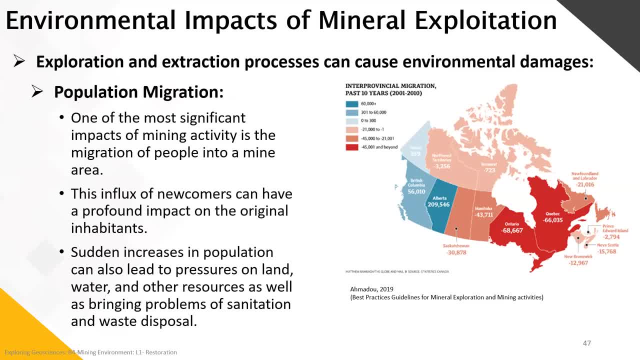 are going after these and jobs that can also cause a negative effect without even putting the mind, because the cities where we have these big population migration increase were not built to receive as many people. so all the infrastructures, all the recycling, uh, all the cleaning, uh, all these cities, plumbing systems and so on are were not built to receive as 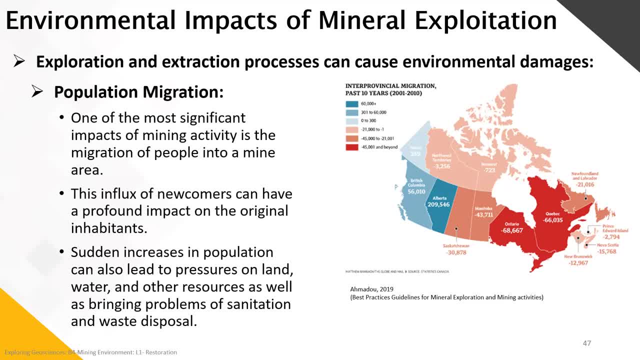 many people, so one of the most significant significant impacts of mining activity is the migration of people into a mine area. this influx of newcomers can have a profound impact on the original inhabitants because they can also feel like they are being invaded in their own privacy and way of life, and sudden increases in population can also be lead to pressures on land. 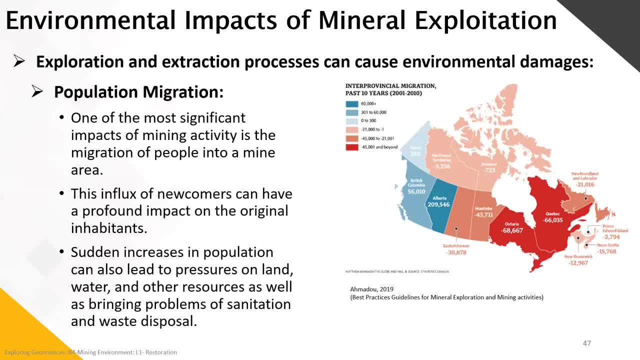 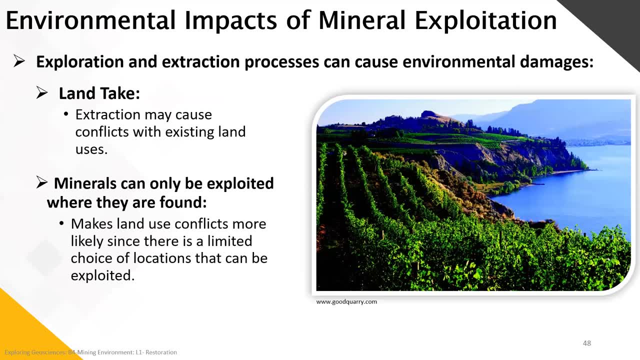 you can see that a lot of our land here have been included in the lower deep End credits and given the very low so water and other resources, as well as bringing problems of sanitation and waste litec, you can see that there are extraction that may cause conflicts with existing land use. the minerals can only be exploited where they are found- we saw that in the last lesson- so they cannot grow. we wish them, unfortunately, so wherever they are. this is the place that we need to expand more. 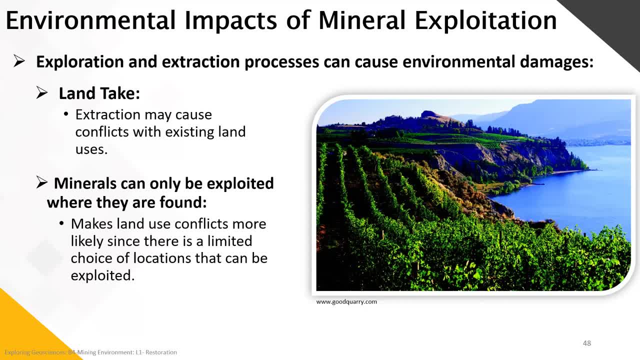 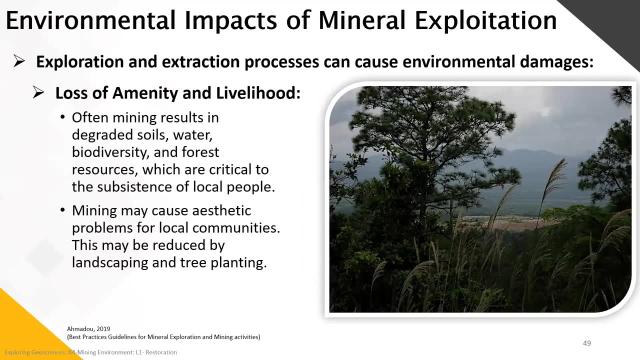 mine them. if we have to mine them, so makes land use conflicts more likely, since there is a limited choice of locations that can be exploited. the loss of amenity and livelihood also can affect uh everything that has to do with uh humanity, social values and so on. so often, often mining. 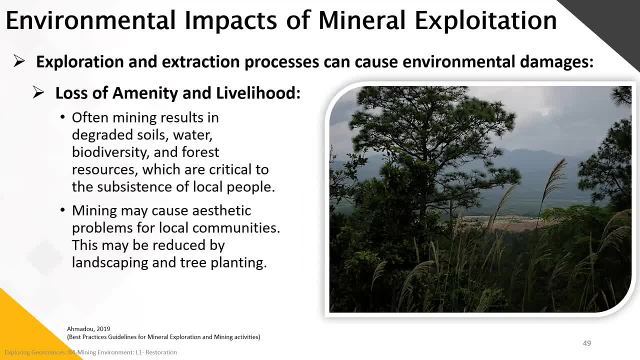 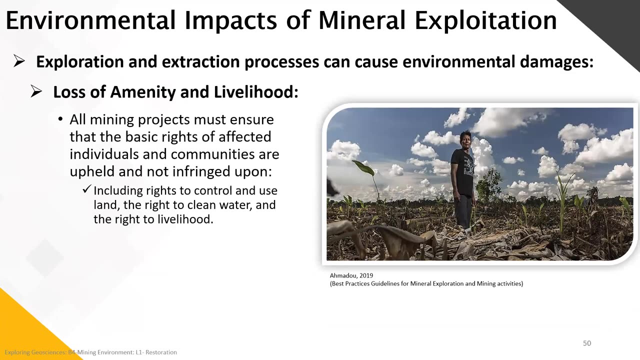 results and degraded soils, water, biodiversity and forest resources, which are critical to the subsistence of local people. mining may cause aesthetic problems for local communities and this may be reduced by landscaping and tree planting, the loss of amenity and livelihood. all mining projects must ensure that the basic rights of 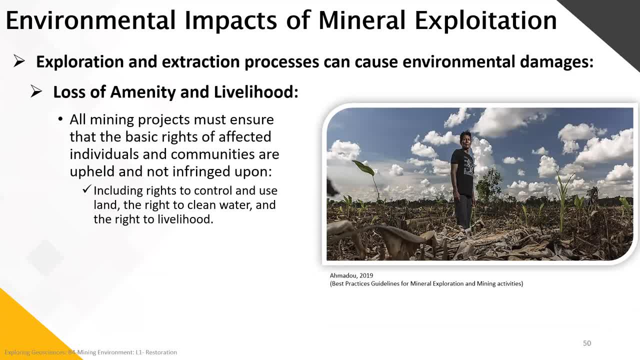 affected environment are followed. individuals and communities are upheld and not infringed upon, so including the rights to control and use the land, the right to clean water and the right to live in it. so no companies should be leaving a site or an environment without the local people having all the rights to have. 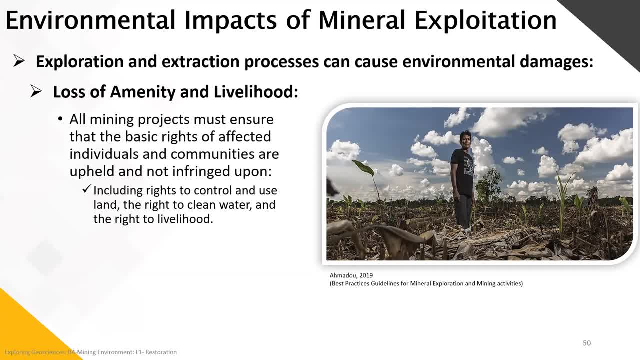 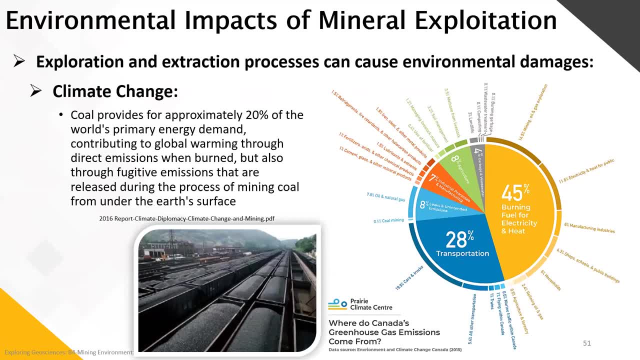 everything to live properly, like the land, the water and so on. climate change: this is a big, big one that is known to be caused again by mining industry. mining, it's not all kinds of mines. that can affect as much the mining industry. sorry, the climate change, the main. 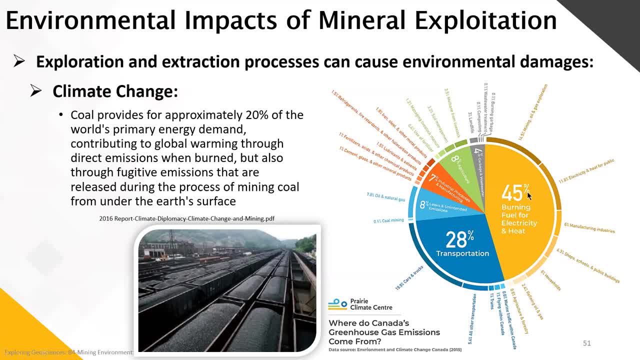 mines that affect the climate change, as seen here, 45 of these are coming from what we call the burning fuel for electricity and heat mines, mainly from coal. 20 of the world's primary energy demand, contributing to global warming through direct emissions when burned, but also through fugitive emissions that 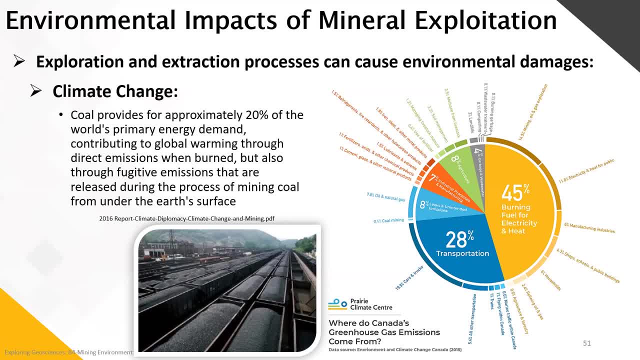 are released during the process of mining coal, but also from under the earth's surface. so burning fuel causes main- almost roughly half of the climate change impact and another quarter roughly- from the transportation of dysmateria. so this is, these are the two main areas to focus. if we move on to another factor that impacts humanity- people. 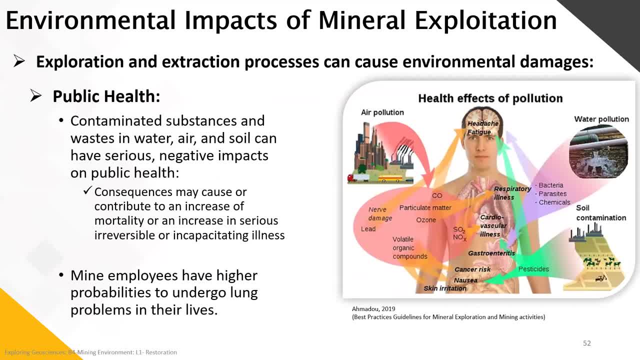 public health and society and we are talking about the massive impact and the positive impact of this populations and so on. cities is the public health. Contaminated substances and wastes in water, air, soil have serious negative impacts on public health. 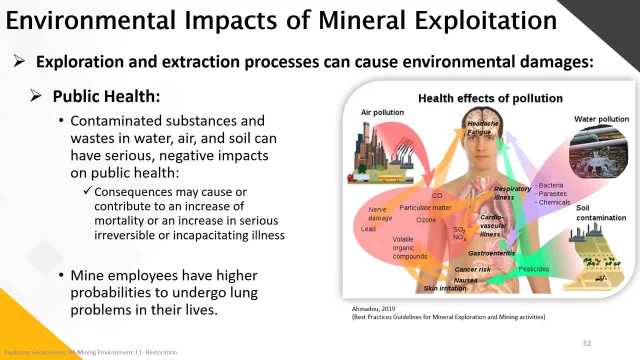 Consequences may cause or contribute to an increase of mortality or an increase in serious, irreversible or incapacitating illnesses. Unfortunately, again, many of these are directly or indirectly set upon the mind of employees which have higher probabilities to undergo long problems in their lives. 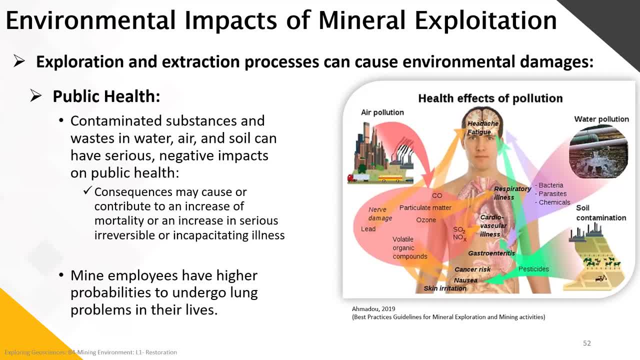 due to their contact. So that is why the companies, for several past years, have included serious programs that have been used to treat these problems, To wear the safety equipment, individual safety equipments, and have teams to make sure that these are respected for the protection of the mind and homes. 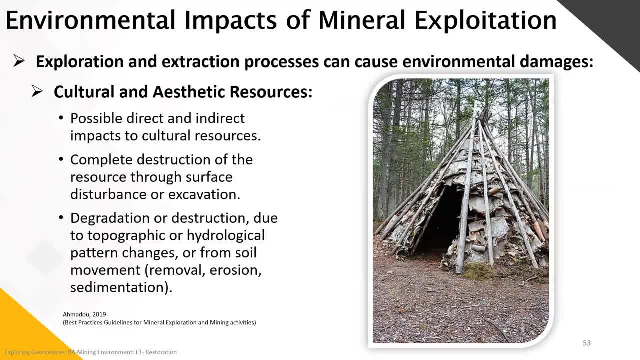 We have the cultural and aesthetic resources, So for both possible direct and indirect impacts to cultural resources. So, for example, we have the complete destruction of resources through surface disturbance or excavation, And we also can have the degradation or destruction due to topographic or hydrological pattern changes. 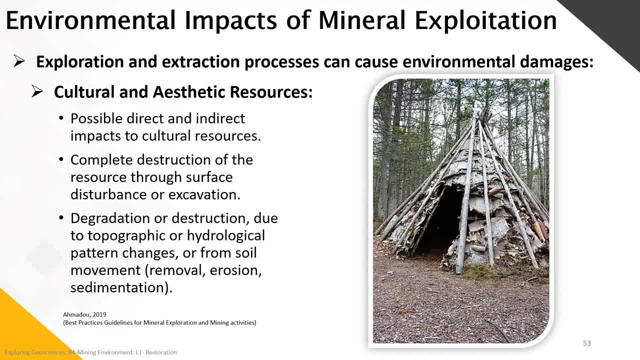 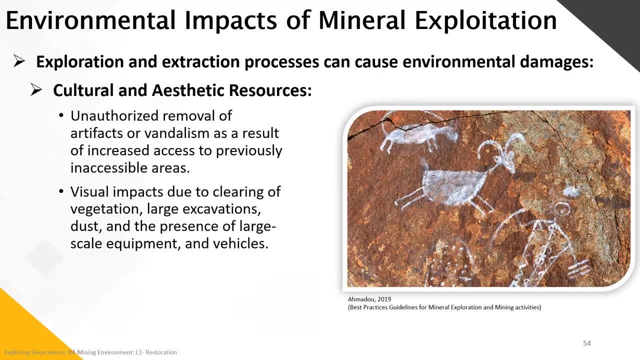 or from soil movement, removal, erosion, sedimentation and so on. Examples also that were seen mostly in South America and Europe was the unauthorized removal of artifacts or vandalism as a result of increased access to previously inaccessible areas, And also the visual impacts due to clearing of vegetation. 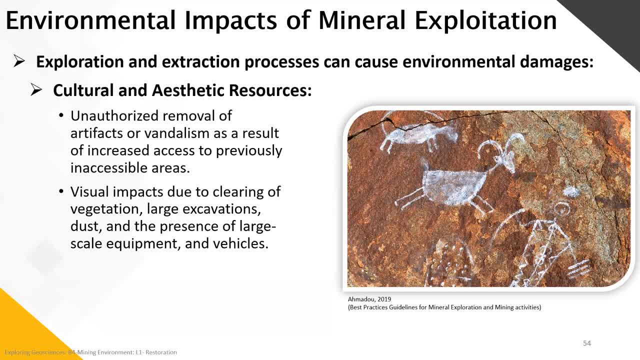 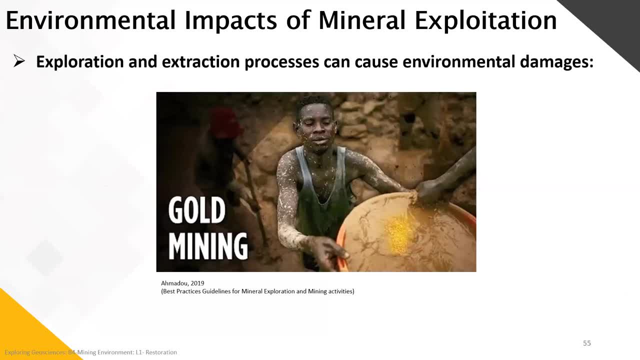 large excavation dust and the presence of large scale equipment and vehicles. I've included also for your own visual impact. I've included also for your own visual impact. I've included also for your own visual impact, the visualization: the gold mining video. 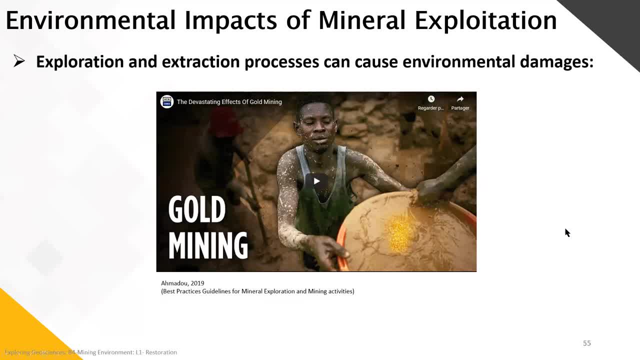 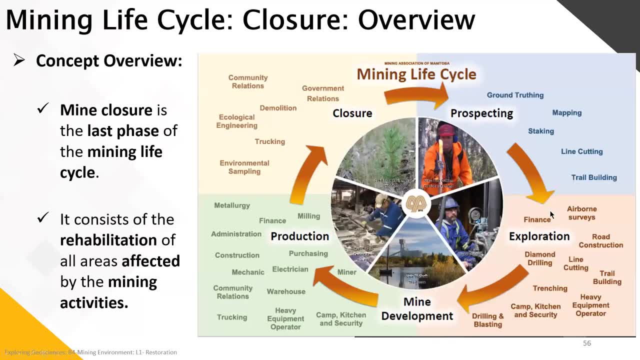 if you want to see it, And its effects on the environment. So now we're going to move on to the mines, what we want to cover, the restoration legislation. So, within the mine life cycle, we are now within the fourth and final stage: the closure. 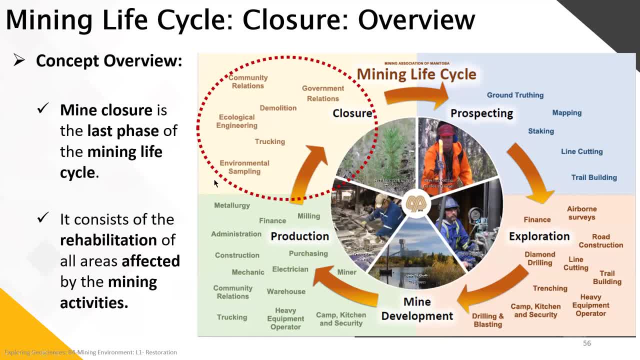 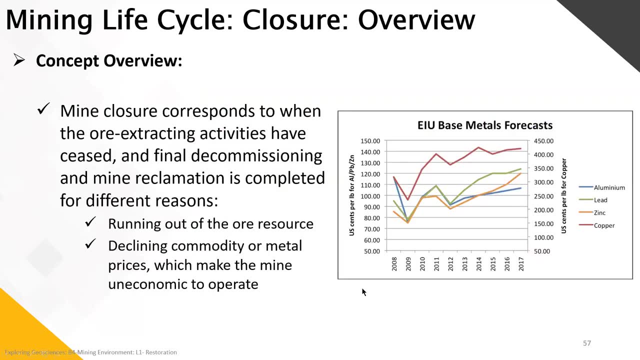 A little overview before we move on. So the mine closure is the last phase of the mining life cycle. It consists of the rehabilitation of all areas affected by the mining activities And the mine closure, as we have seen in the last lesson, corresponds to when the ore extracting activities have ceased. 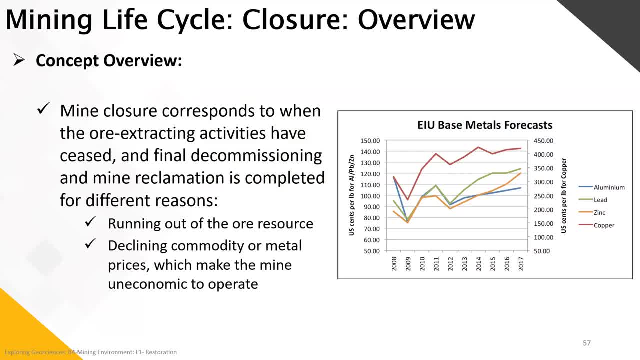 and the final decommissioning and mine reclamation is completed. for different reasons, reason mainly running out of ore resources or declining of commodity or metal prices, which make the mine uneconomical to operate at a given time. Mines must plan their closure. 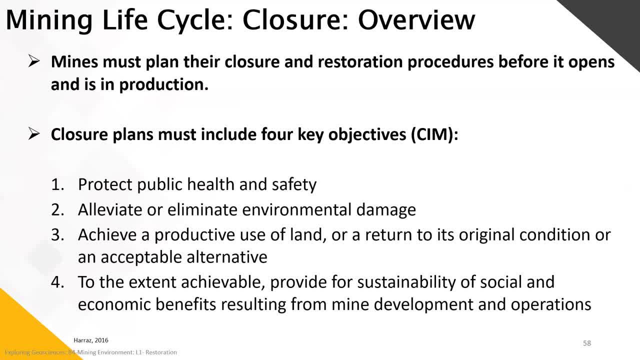 and restoration procedures before it opens and is in production. So this is a major changing legislation that has occurred and which was absent from all the historical mines' horror stories, And this was defined to make sure that no more environmental disasters effects would be done by the mining companies. So there are four for the closure plans. These 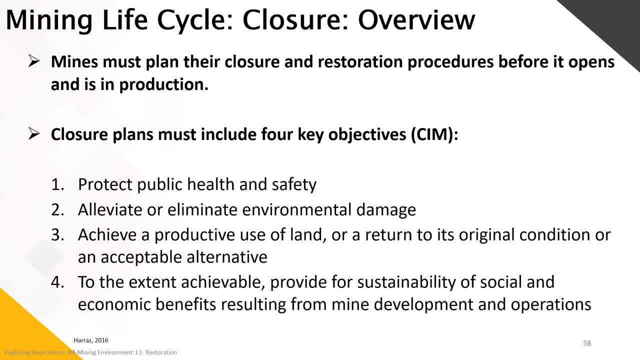 include four major objectives as defined by Tarif Al Shapiro- Soria, the canadian institute of mining, vcim. so they are done to mainly to protect the public, health and safety. to alleviate or eliminate environmental damage. to achieve a productive use of land or a. 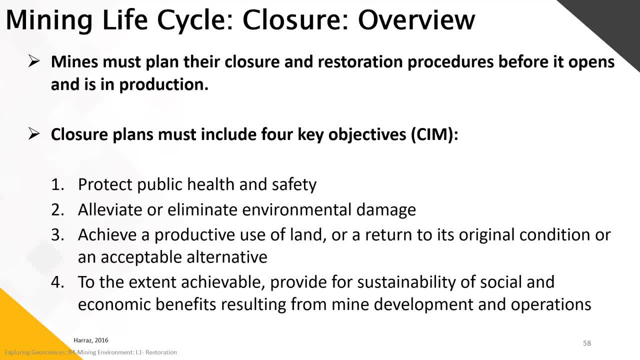 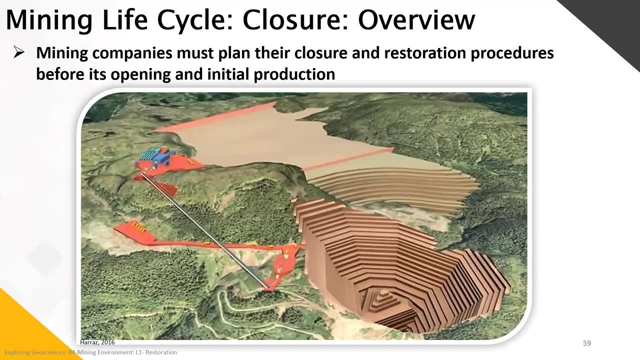 return to its original condition or unacceptable alternative and finally, to the extent achievable, to provide for society sustainability of social and economic benefits resulting from mine development and operations, as we've seen in the last lesson, when the mining companies must plan their closure and restoration procedures before its opening and its initial production. as this is done, it also has to 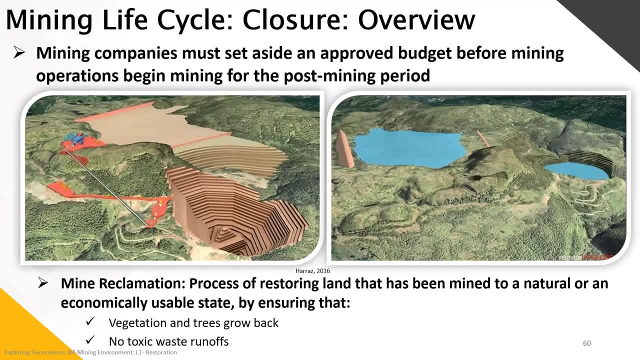 set aside and approve the budget before mining operations begin the mine for the post mining period and this is mainly done for the, the mine reclamation. so the mine reclamation process is um of restoring the land has been buying to a natural or an economically usable state, by ensuring that both 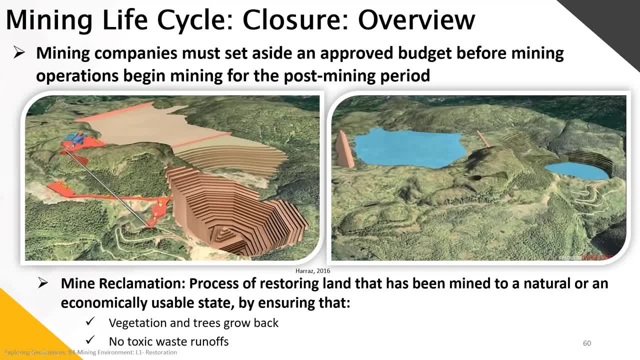 vegetation and trees grow back and that no toxic waste runoffs, so as before the mine opens. as important, the plan is to set up the concept of the development, development of the mine and all its buildings and infrastructures. they will also have a plan set up with the step by step to restore. 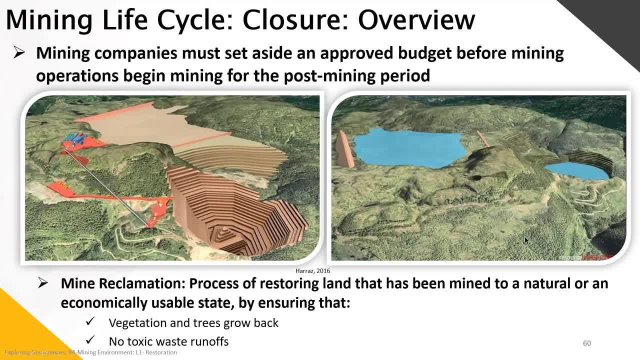 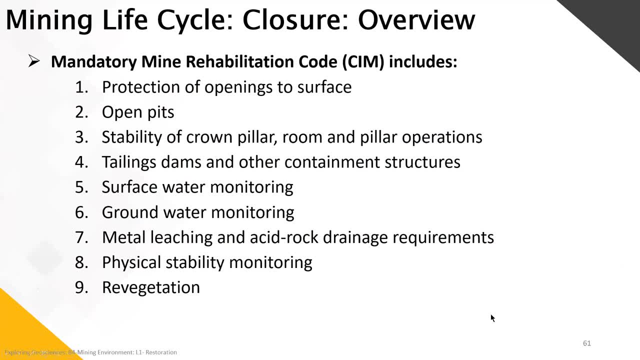 that area to a respectable natural environment process. the mandatory mine rehabilitation code from the park technique is rolled out in public at the mine. haha, a mid as it should be. basically, the team is karim affa is key to its success in the back-end, so the mean is standing Momo. 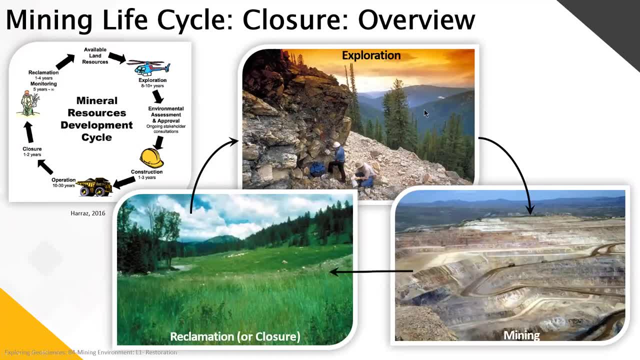 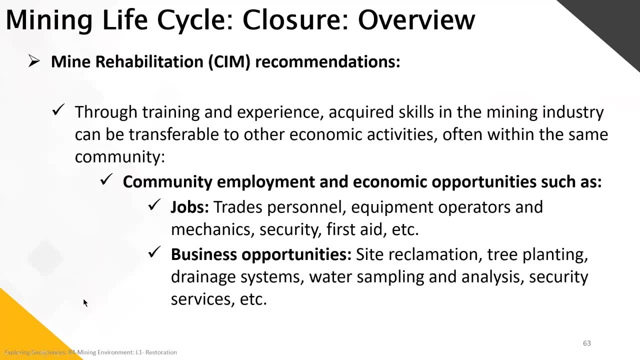 sign up embaixo. that's me. so, Milie, Monique, As we've seen in the last two lessons, exploration, mining, recreational exposure, So the mine rehabilitation from the CIN the main recommendation. through training and experience, acquired skills in the mining industry. 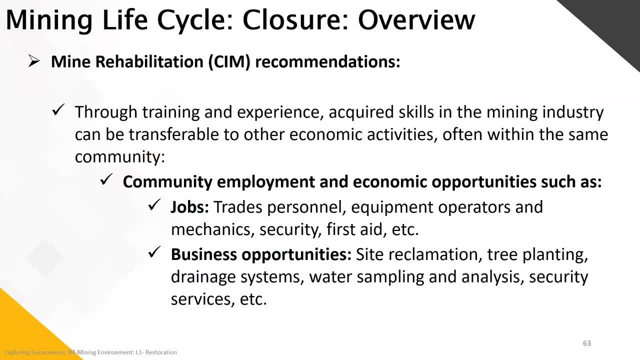 can be transferable to other economic activities, often within the same community. This is very important because community employment and economic opportunities, such as the jobs and the business opportunities, so both for the jobs that were created to work on the mine, so the trades personnel, the equipment operators. 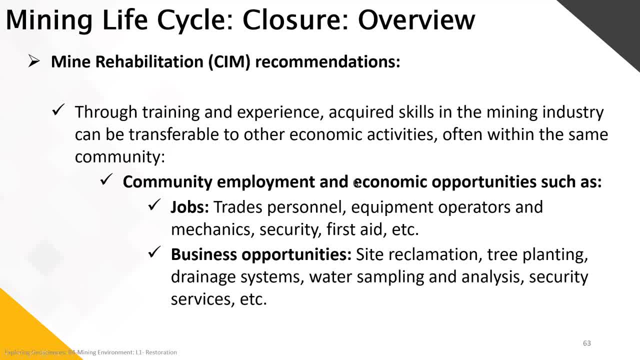 and the mechanics, security, first aid, et cetera. they would be used for, within the business opportunity for the end of the cycle. They could be on site for the site reclamation, the tree planting, the setup of the drainage system, the water sampling and analysis. 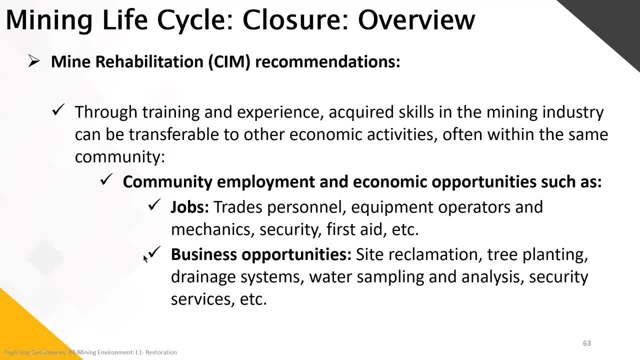 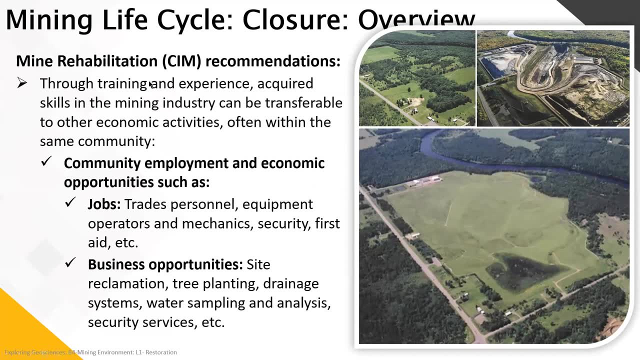 and the security services, So these traits could be recycled to be present within the last phase of the mine, The mine rehabilitation recommendations through the training and so on that we see. So this is an important factor as when the company needs, At the same time the company assures 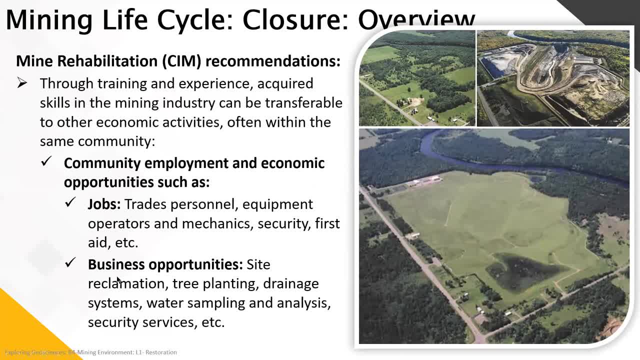 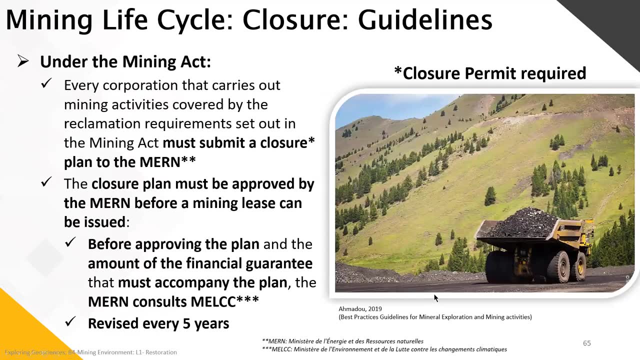 that all the community within the area can be economically active and secure their finances through ongoing work on the site for several years. So now we're going to move on to the closure guidelines And I'm just going to give you some important excerpts from the major legislation. 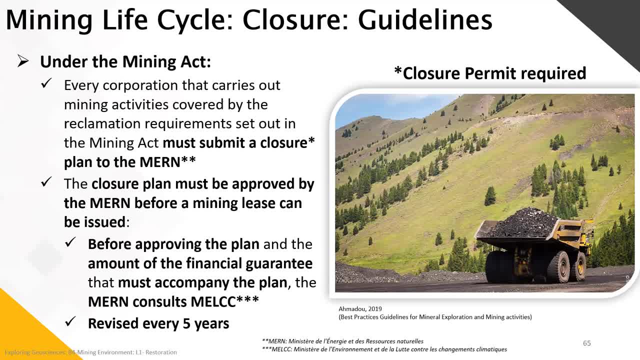 I've included in the documents for this lesson many of these official PDF files, And I will also include on my slides the important links for these legislation. But for this presentation I wanted to generalize these so that the major knowledge of these can be exerted within this lesson. 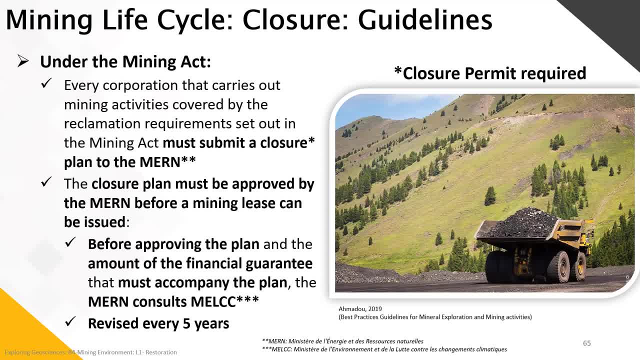 So under the Mining Act, every corporation that carries out mining activities covered by reclamation requirements set out in the Mining Act, they must submit a closure plan to the Ministry, the Ministry of Energy and Resources of Quebec. So their closure plan, they need to have a closure permit. 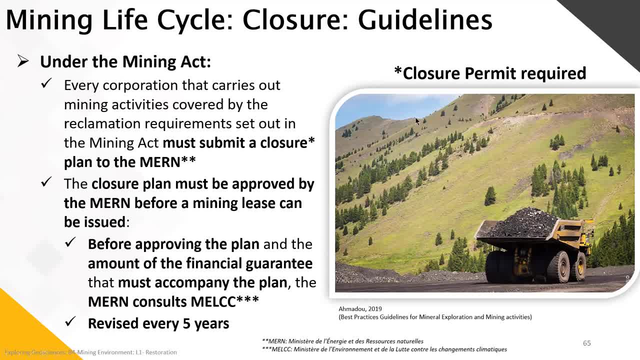 requirement. That's one of them. The closure plan must be approved by the MERN before a mining lease can be issued. So before approving the plan and the amount of the financial guarantee that must accompany the plan, the MERN itself will consult the MELC. 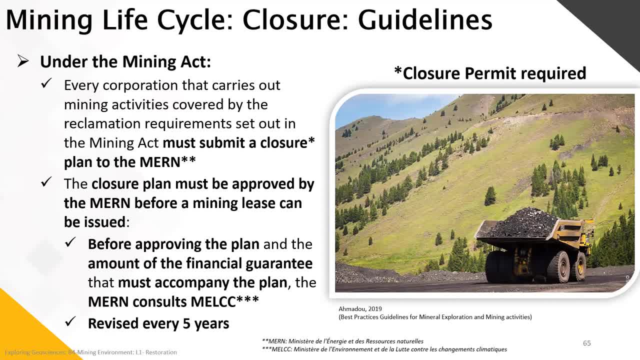 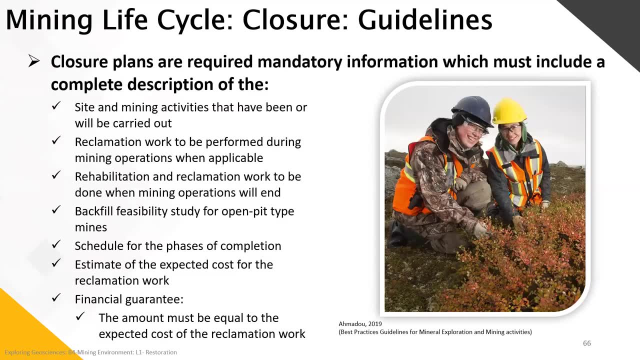 The MELC is the Ministry of Environment and their fight against the climatic changes. And this plan, importantly, is really important to the Mining Act. It must be approved by the Mining Act and it must be revised every five years. The closure plans are required, mandatory, to give mandatory. 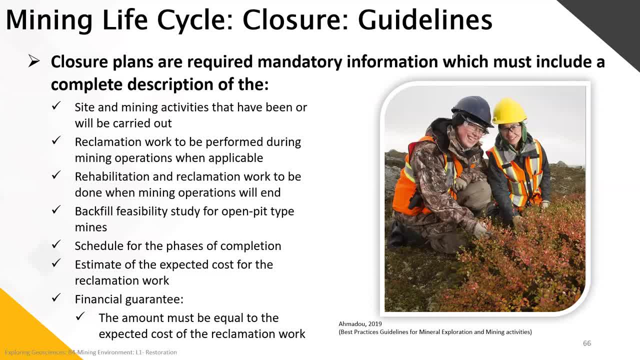 information, which must include a complete description of the following points: Site and mining activities that have been or will be carried out. The reclamation work to be performed during mining operations, when applicable. The rehabilitation or reclamation work to be done when mining operations are completed. 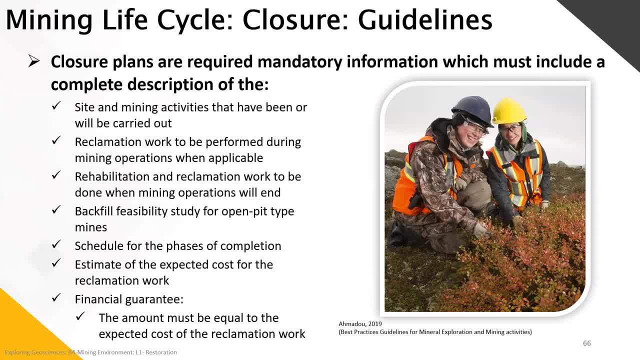 And the backfill feasibility study for open pit pipe mines, The schedule of the phases of completion, The estimate of the expected cost for the reclamation work And the financial guarantee. Yes, the financial guarantee, That's a big point, major point. 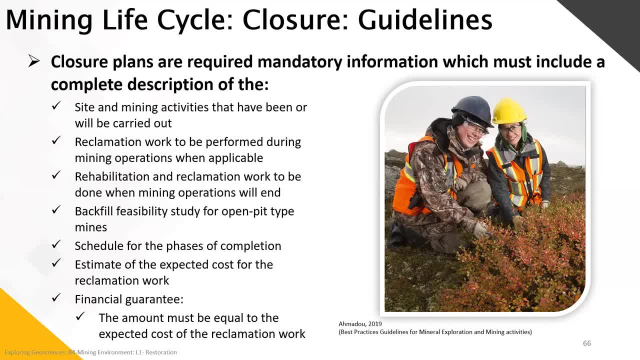 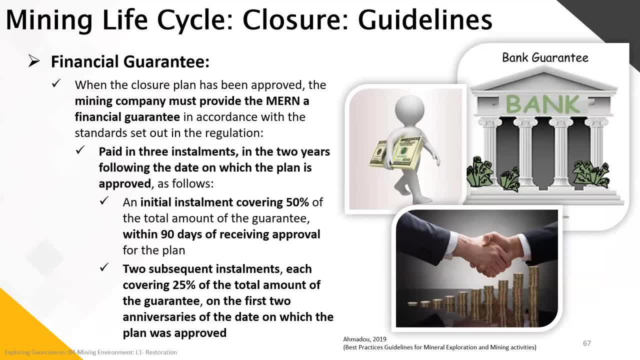 The amount must be equal to the expected cost of the entire reclamation work. So the financial guarantee: When the closure plan has been approved, the mining company must provide the MIRN a financial guarantee in accordance with the standards set out in the regulation. 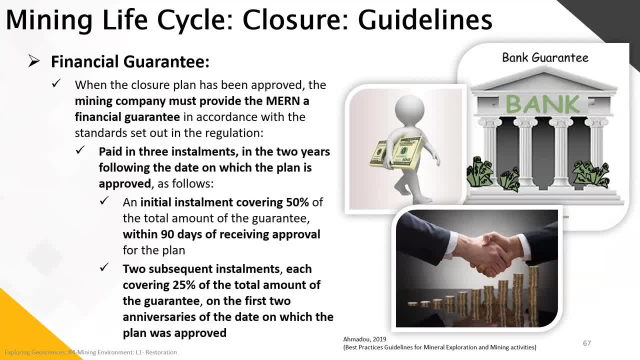 They must be paid in three installments in two years following dates on which the plan is approved And the payment. the installments are done as follows: There is an initial installment covering 50% of the total amount of the guarantee Within 90 days of receiving approval for the plan. 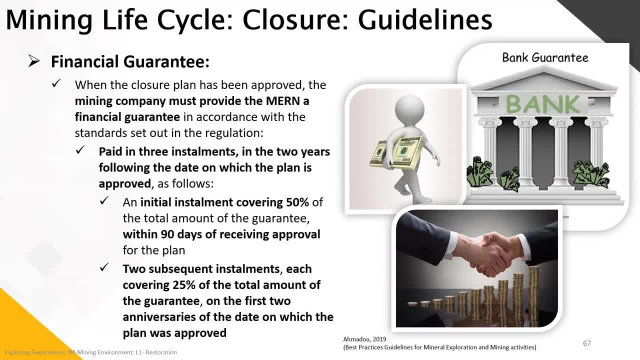 So half of it is already paid before the mine is even constructed. Two subsequent installments each covering 25% of the total amount of the guarantee on the first two anniversaries of the date on which the plan was approved. We- I will just do a little bracket for temporary. 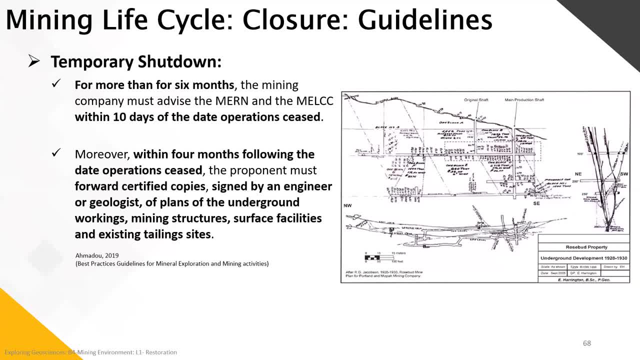 So the first two anniversaries of the date on which the plan was approved, We- I will just do a little bracket for temporary. So the first two anniversaries of the date on which the plan was approved, We have the temporary shutdown. 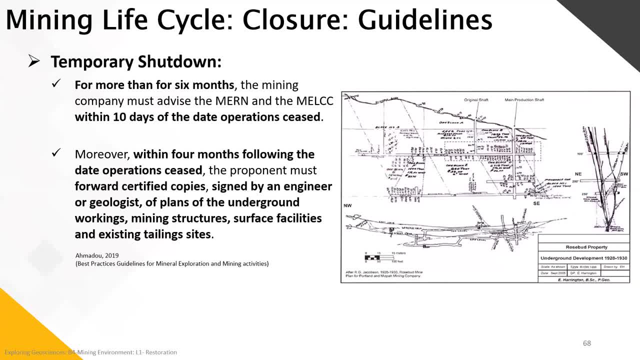 that sometimes that can show some mines shut down temporarily. Historically, some of these temporary shutdown we're not monitored and cause some environmental damages, And so the Ministry also applied some legislations for these temporary shutdown to make sure that the both the mining company would not run. 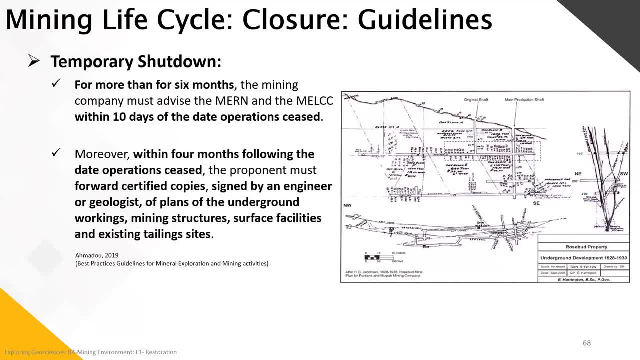 off without being responsible. So for temporary shutdown for more than six months, the mining company must advise the Ministry and the MEL within 10 days of the date operation ceased. Within four months following the date of operation ceased, the proponent must forward certified copies, signed by an engineer or geologist, of the plans if it is an underground shutdown. 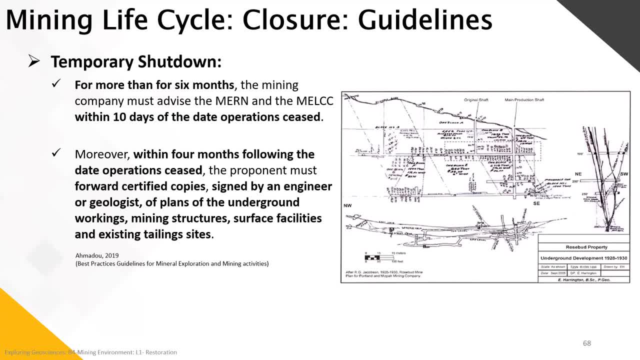 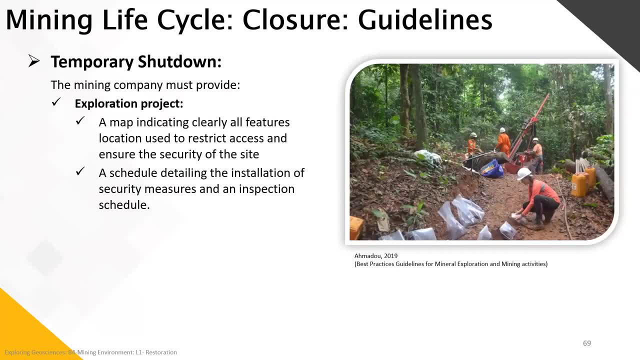 mining structures, including the mining structures, the surface facilities and all existing tailings sites. If we are working on an exploration project stage for a temporary shutdown, the mining company must provide a map indicating clearly all the features, locations used to restrict access and ensure. 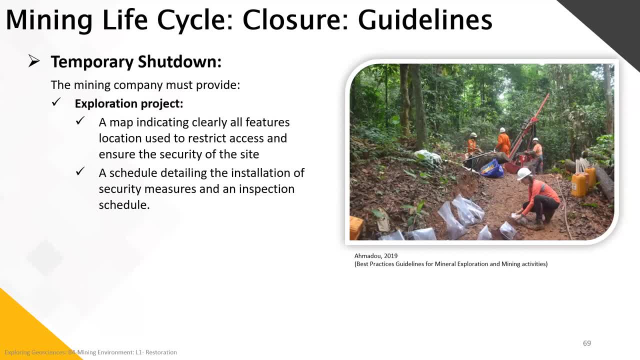 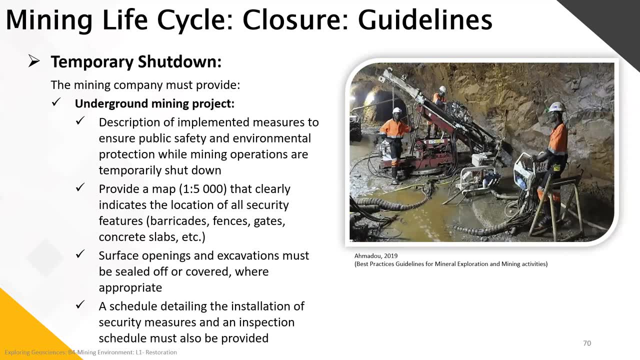 security of the site and also include a schedule detailing the installation of its security measures and an inspection schedule. If we are working with any underground mining projects, the mining company for a temporary shutdown must provide the following, including description of implemented measures to ensure public safety. 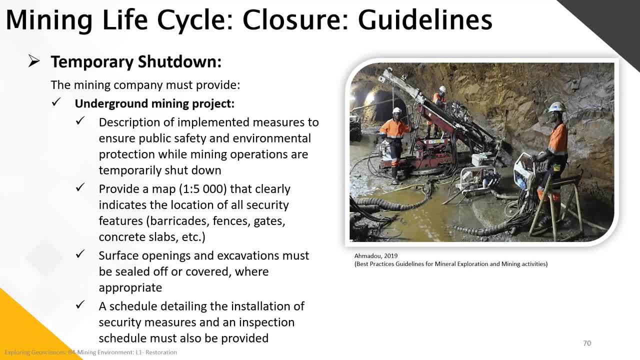 and environmental protection while mining operations are temporarily shut down. They must provide a detailed small scale- 1 to 5,000, that clearly indicates the location of all security features, like the barricades, the fences, the gates, concrete slabs, etc. 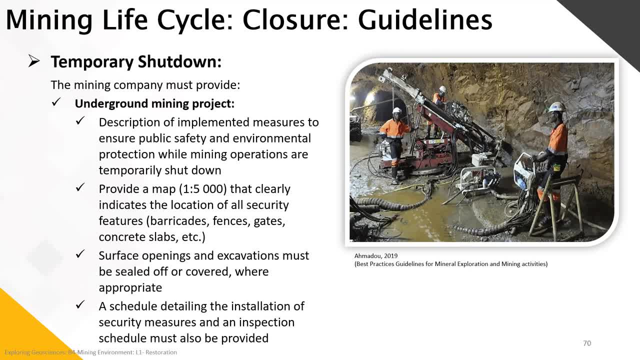 They will also need to give surface openings, and excavations must be sealed up or covered where appropriate. And finally, they must also provide a schedule detailing the installation of security measures, and an inspection schedule must also be provided to make sure that the site is not abandoned. 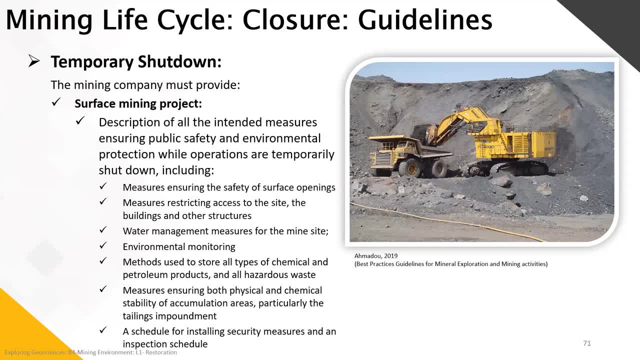 For surface mining projects, the mining company must provide a description of all the intended measures ensuring public safety and environmental protection while operations are temporarily shut down, and these must include all the measures ensuring the safety of the surface openings, all the measures restricting access to the site, the 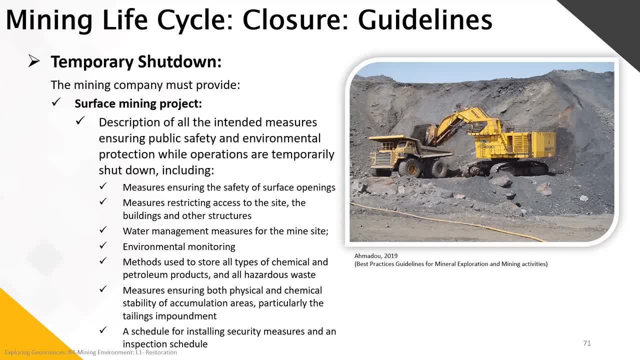 buildings and other structures, the water management measures for the mine site, the environmental monitoring of the mine site, the methods used to store all types of chemicals and the maintenance of the site. They must include all the necessary technical and petroleum products and all other such 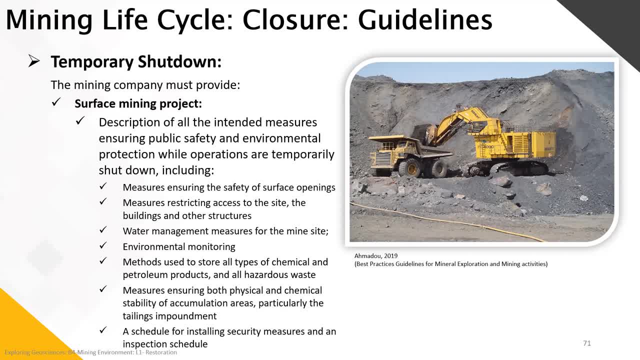 waste. since the mine is temporarily shut down, All this material is sitting there on the mine site and has to be monitored. Measures must also include the measures ensuring both physical and chemical stability of accumulation areas, particularly the tailings and fibers, And finally also a schedule for installing security measures and an inspection schedule. 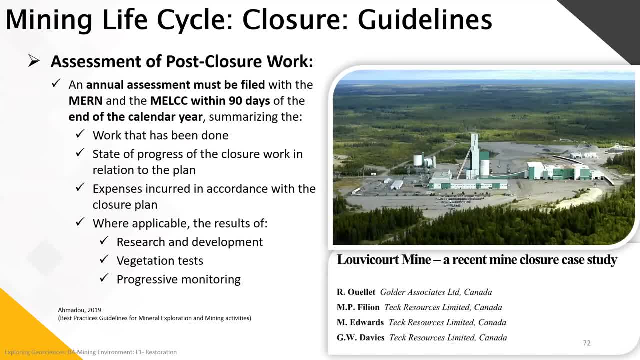 Thank you. Thank you, Bye-bye. For the assessment of post closure work. I've included an example of the Louisville mine within the Abitibi area, the plan that was done, So I have a PDF file that was included with this lesson. 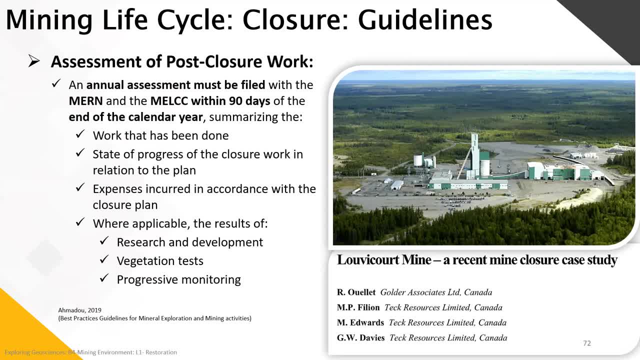 And it will show how it was done. So, basically, it was an annual assessment that was filled with demerin and the milk within 90 days of the end of the calendar year, as said before, And this summarizes the work that has been done, the state of progress of the closure work in relation to the plan, expenses incurred in accordance within the closure plan and, finally, 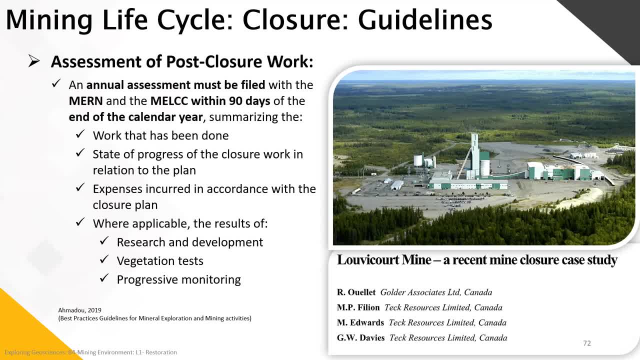 the results of research and development, vegetation tests and the progressive monitoring. So you have to understand that a lot of these closed mining sites are becoming also the field where a lot of research teams go to test either new methods, new vegetation to apply for the re-vegetation of the area. 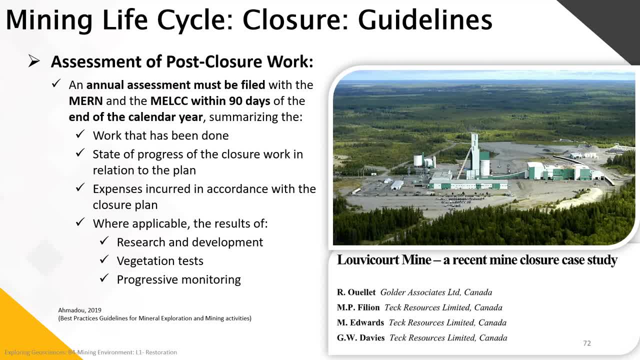 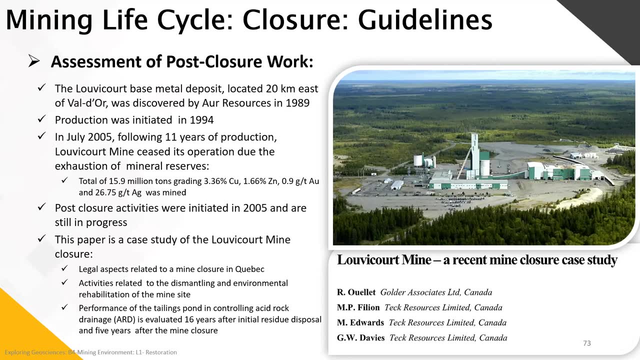 And this is really important- And also to monitor these studies. So this becomes a nice research playground for the research teams Mainly- I will not go through everything, but mainly- within the Lubico area. The example will show how the mine started and how the post closure activities were initiated. 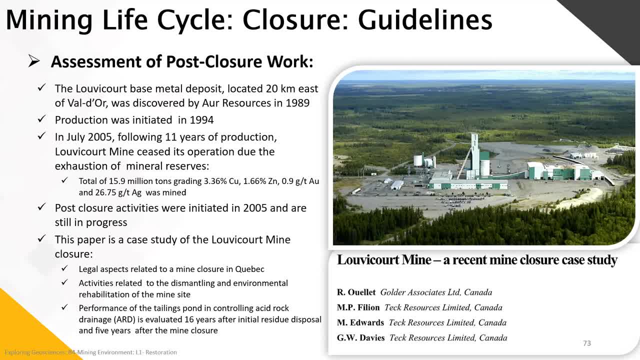 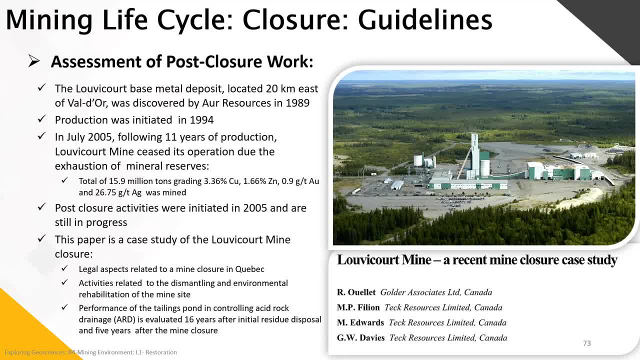 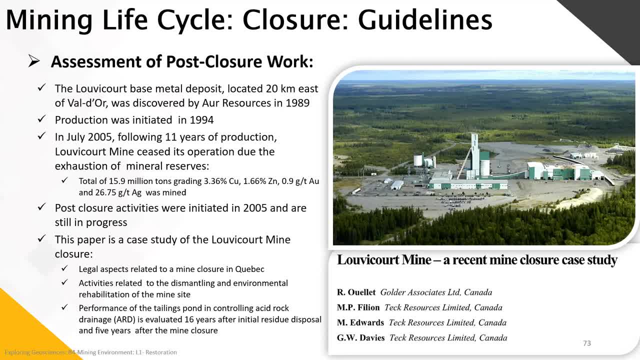 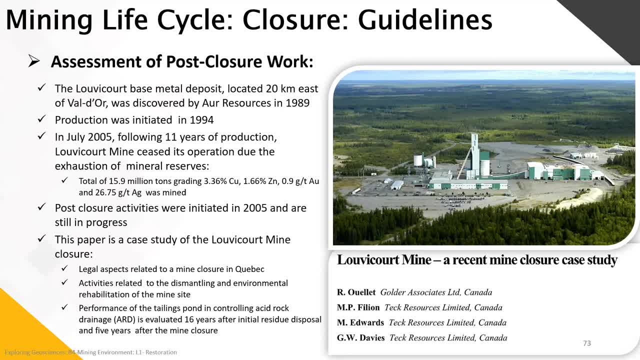 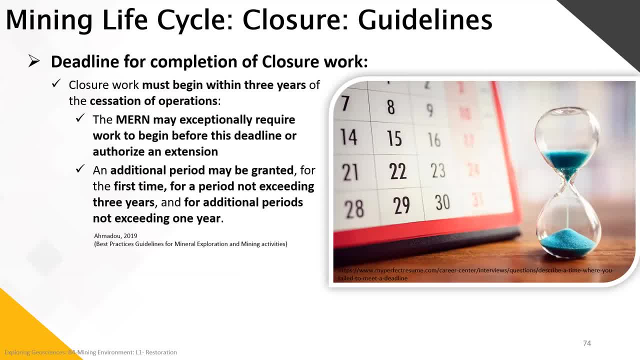 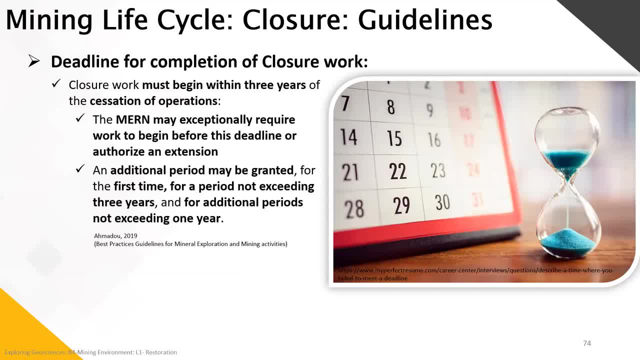 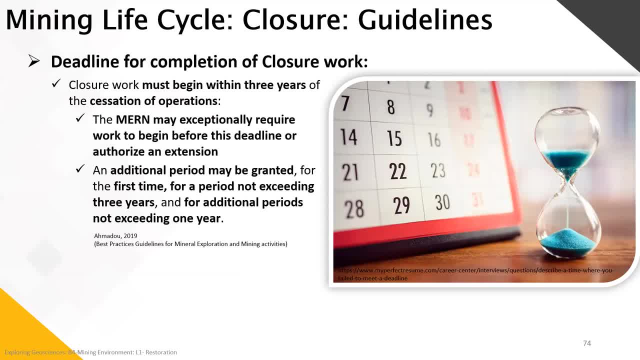 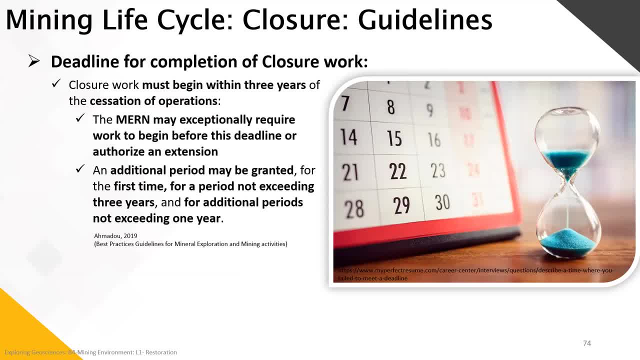 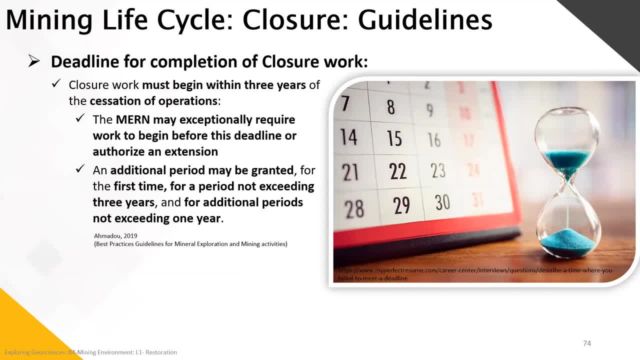 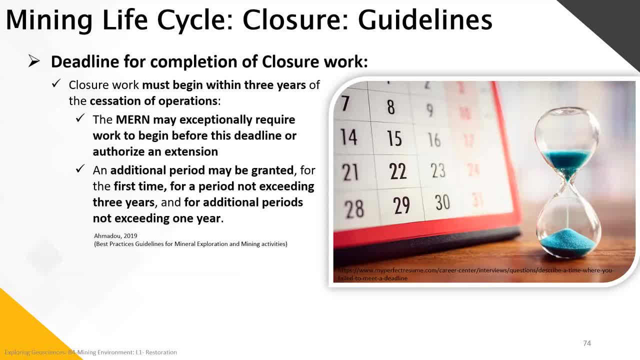 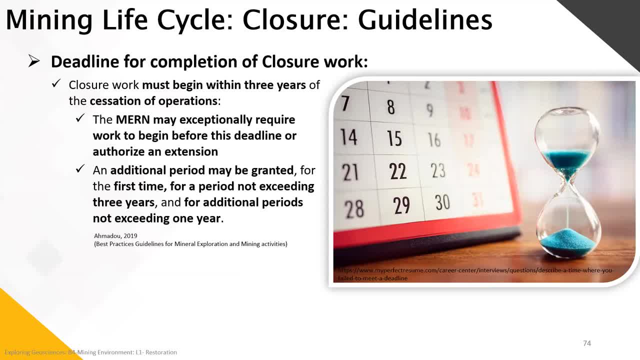 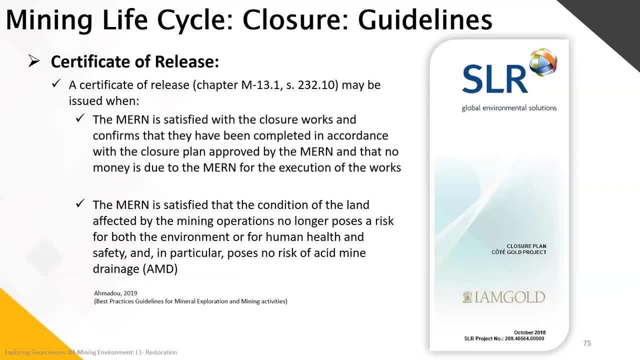 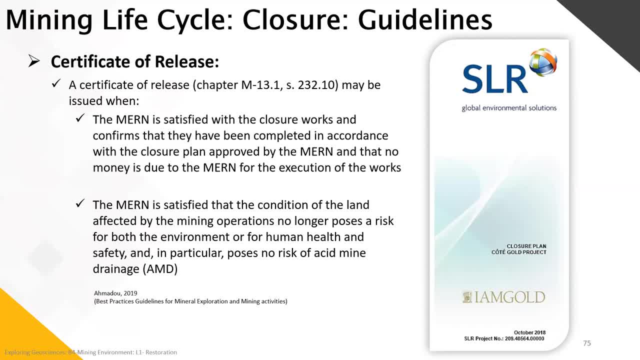 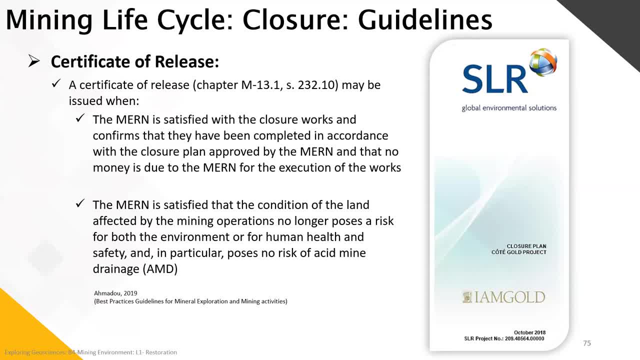 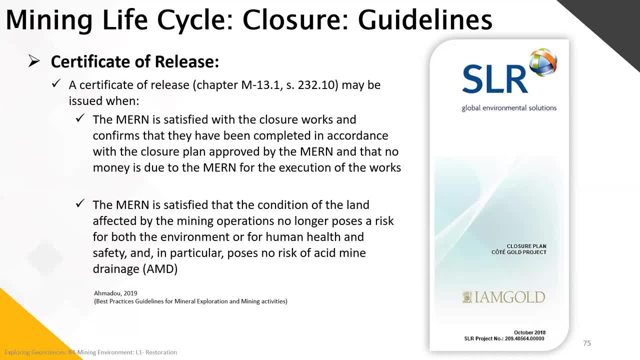 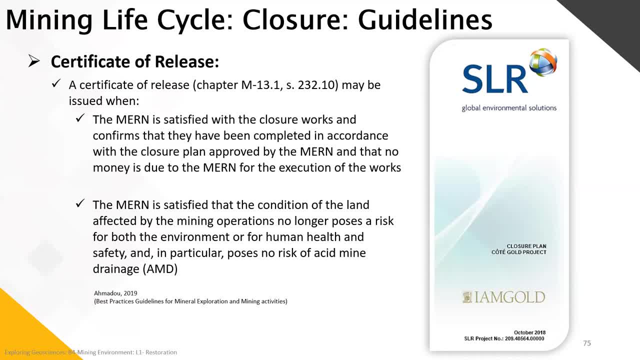 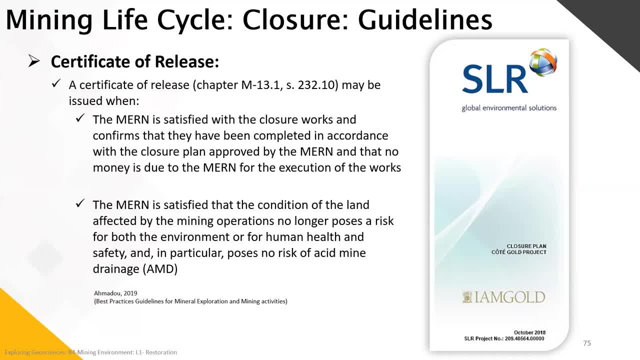 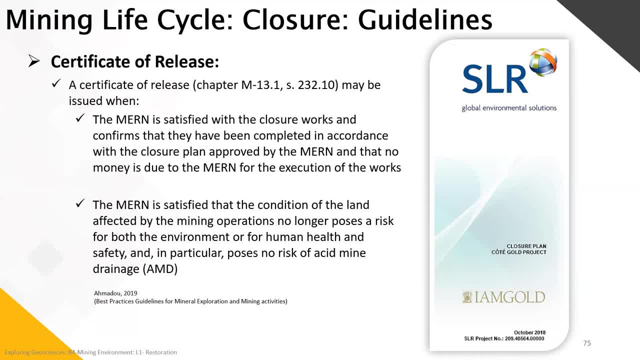 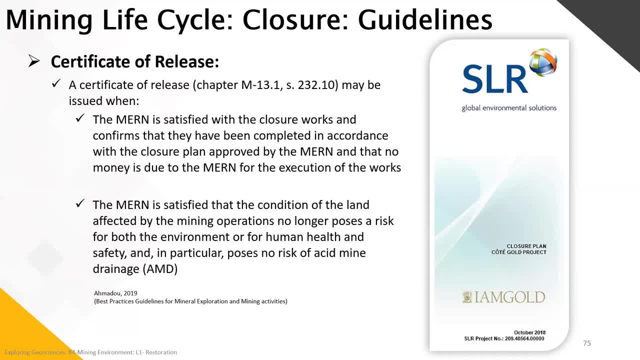 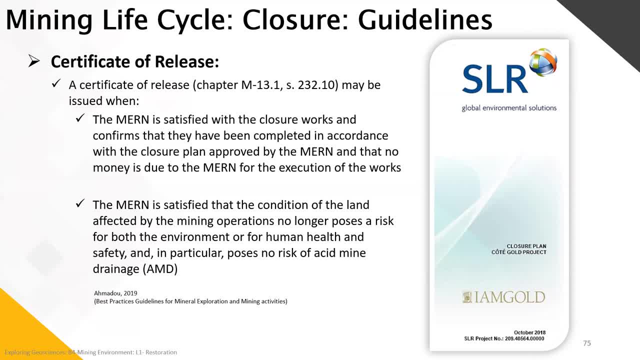 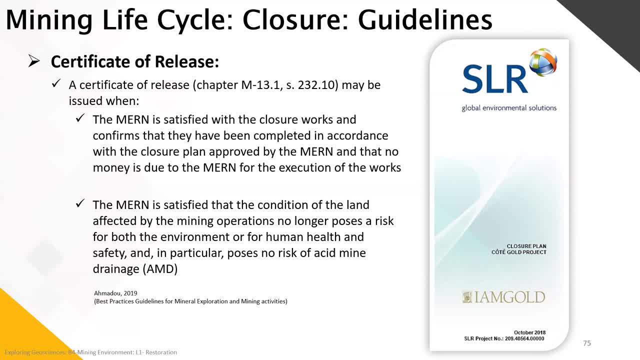 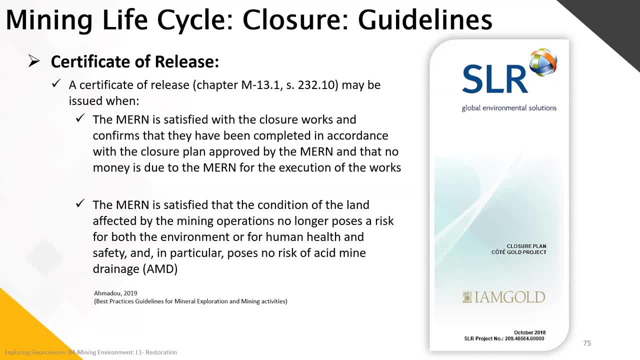 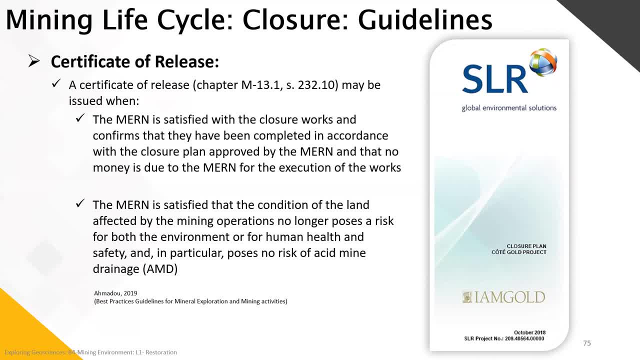 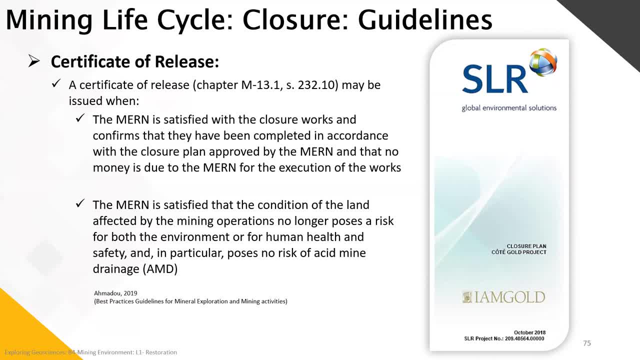 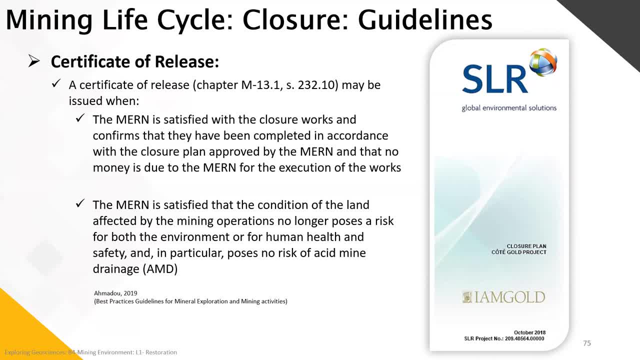 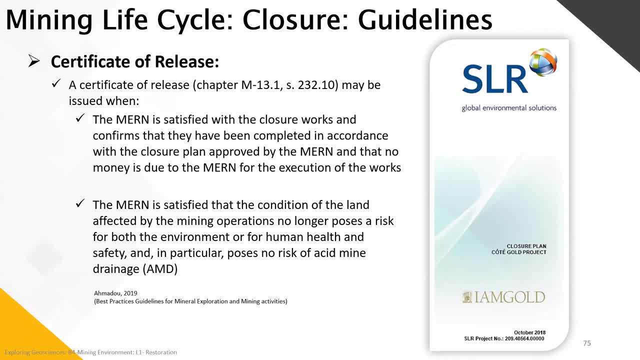 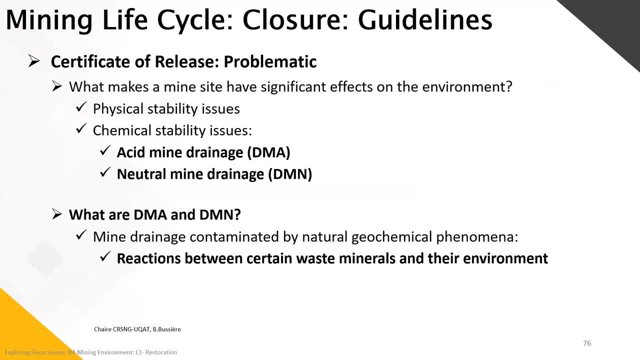 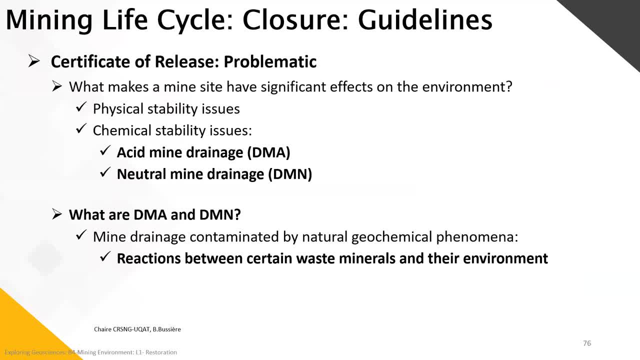 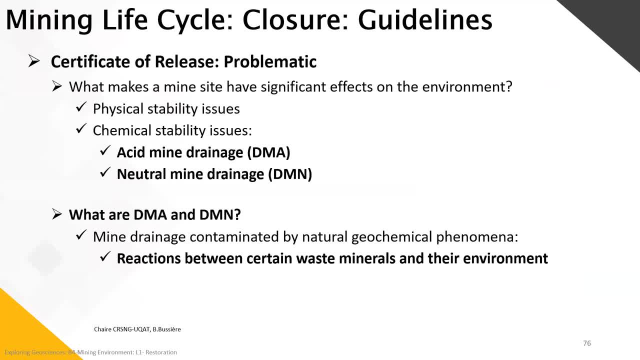 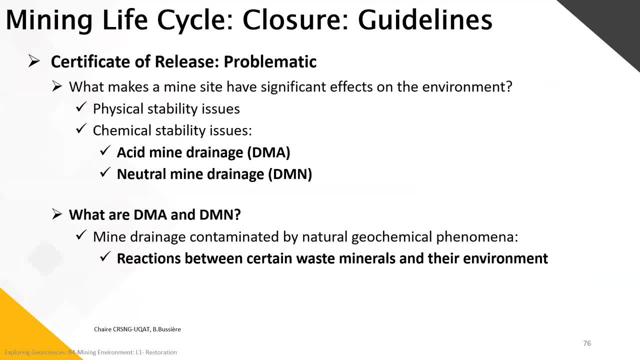 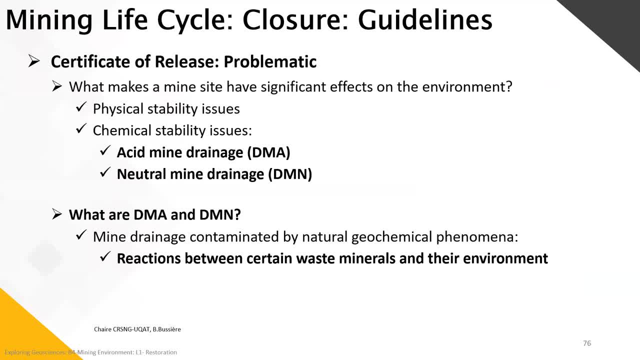 And it is the case study showing how the mine started. And it is the case study showing how the mine started And it is the case study showing how the mine started drainage. So what makes a mine site have significant effects on the environment? We have both the 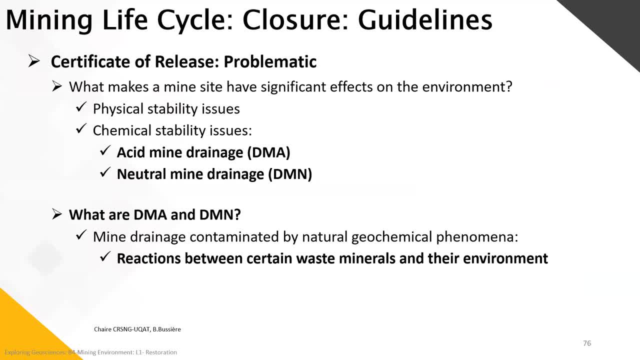 physical stability issues and the chemical stability issues. What are the DMA and DMM? So the mine drainage contaminated by natural geochemical phenomena, The reactions between certain waste minerals and their environment. But understand that the waste minerals, we call them waste minerals but they are natural occurring minerals. So for the acid mine: 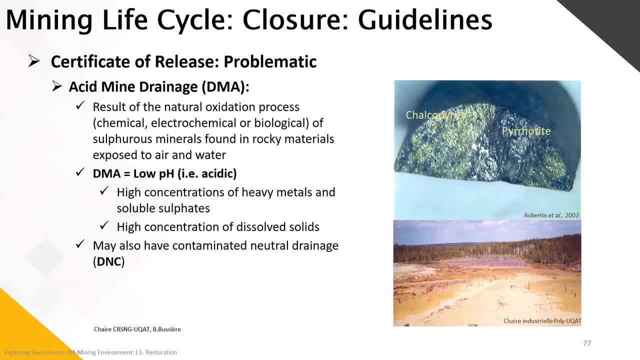 drainage. the result of natural oxidation process is either from chemical, electrochemical or biological, like we saw before, from bacteria, Of sulfurous minerals found in rock united materials exposed to air and water. So it's natural oxidation process. DMA drainage is. 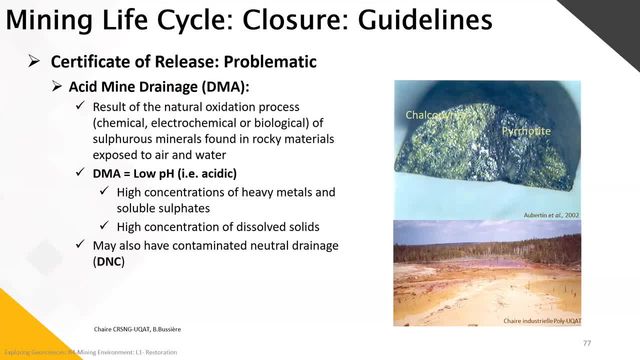 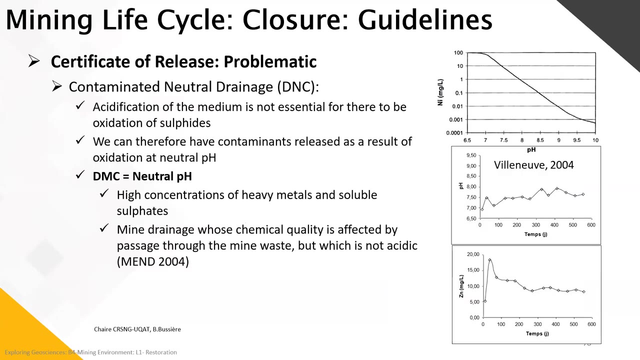 basically low pH. so within acidic environments And the high concentrations of heavy metals and soluble sulfates are within these sites with high concentration of dissolved solids They may also have contaminated neutral drainage And these they reflect acidification of an area. Here's PAH. We're in the 5 pH range. So we're in the 5 pH range where there are no oxidations. 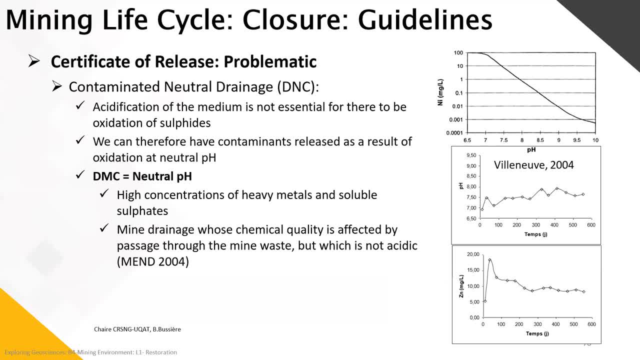 of the sulfide, So we can therefore have contaminants released as a result of oxidation, But at a neutral pH range. this time we are within the 7 pH, which is not acidic, And these are within high concentrations of heavy metals and soluble sulfates And the mine drainage. 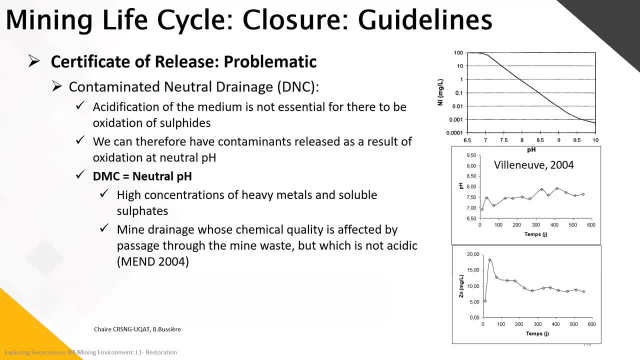 whose chemical quality is affected by these solutions. As I said, it depends on the Pakistan, the by passage to the mine waste but which is not acidic, as seen here, within time, the concentration of zinc within the time and within time, the concentration of the pH, which is majorly. 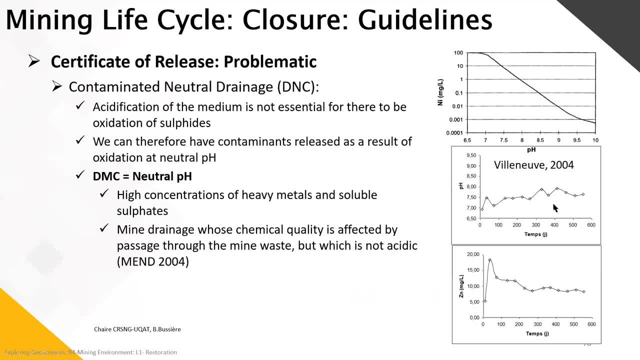 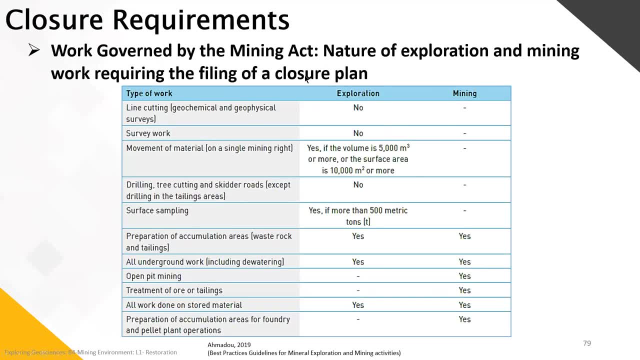 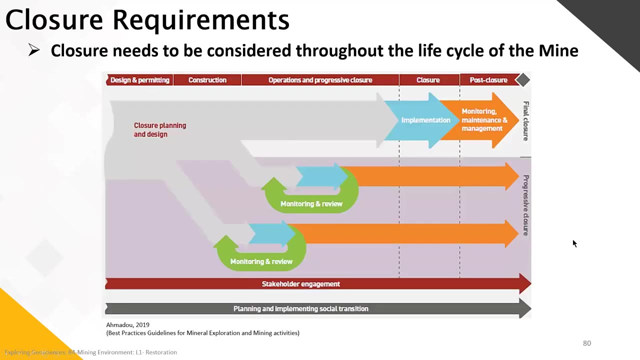 neutral around the 7-7.5 pH. This I've included so you can see the difference between the Mining Act legislation. if you are within an exploration or a mining project, The closure needs to be considered throughout the life cycle, as we've seen so far, and is not just 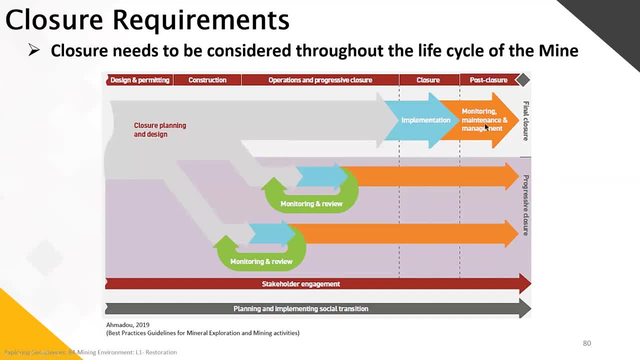 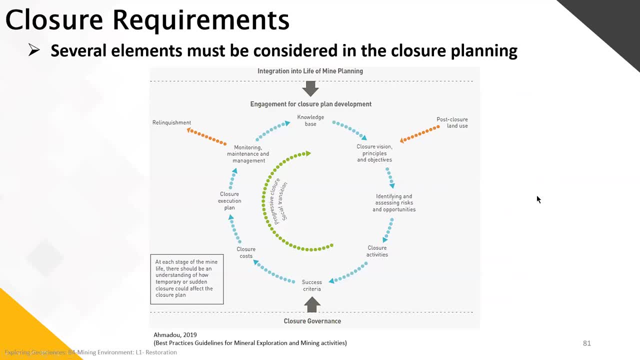 happening at the last state or the post closure step. These will show the several elements that must be considered, Considered in the closing of the mine planning. and the closure of the mine Planning is a cycle itself, so I will start with knowledge base. 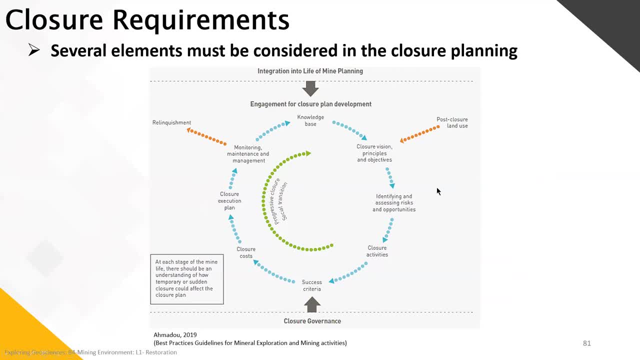 using to define the plan. the closure vision, the principles and the objectives are defined with this knowledge and then identifying and assessing and the opportunities, risk for this Planning, the closure activities, the success criteria, the closure cost and the closure. 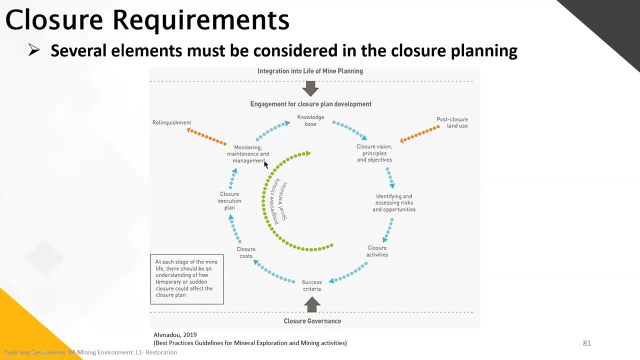 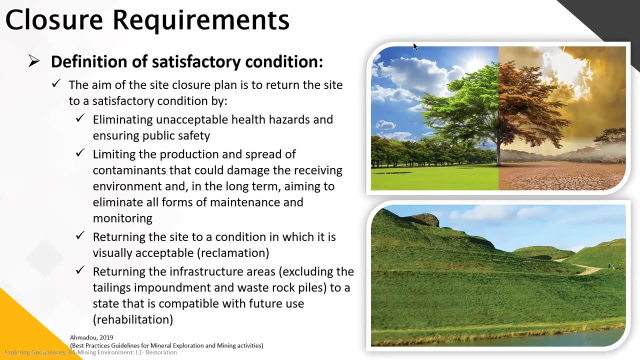 execution plan to make sure that everything is monitored, maintained and managed. to make sure that this plan is certified The definition of satisfactory condition. At the top I put the utopic visualization: We are moving from this environment To a perfect green environment. 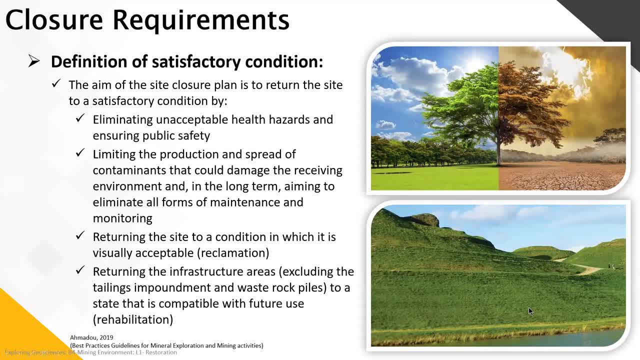 This is utopic. This is realistic, So we can still see some of the topography effect of the mining, but these are reduced and revegetated and so then the area can be reused for other purposes. So the aim of the site closure plan is to return the site to a set 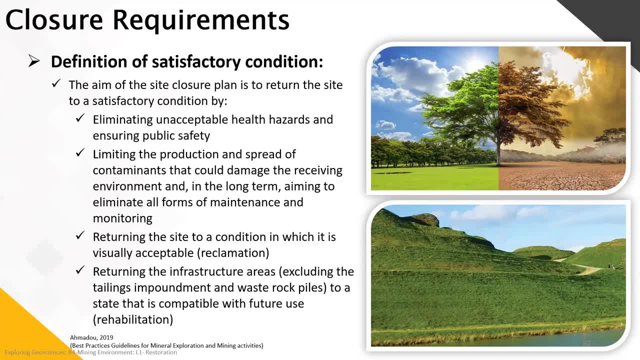 satisfactory condition. That is the thing to remember. It will never be returned to its initial state. Eliminating unacceptable health hazards and ensuring public safety, limiting the production and spread of contaminants that should damage and receive environment and, in the long term, aiming to eliminate all forms of maintenance and monitoring. returning the site to a condition. 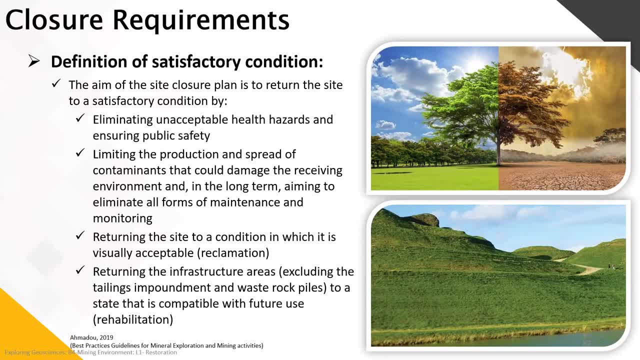 in which it is visually intact, It will be acceptable, which is called a reclamation, and returning the infrastructure's areas, including the tailings, impoundments and waste rock piles, to a state that is compatible with future use. This is the rehabilitation. 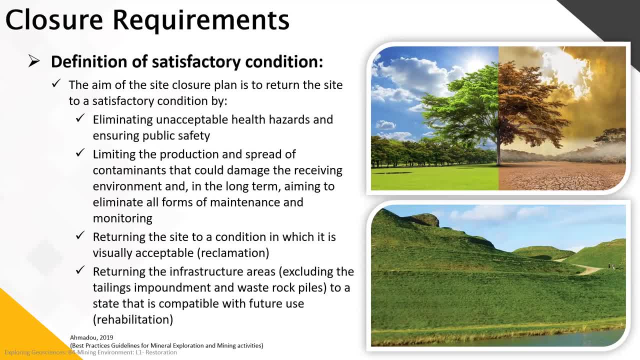 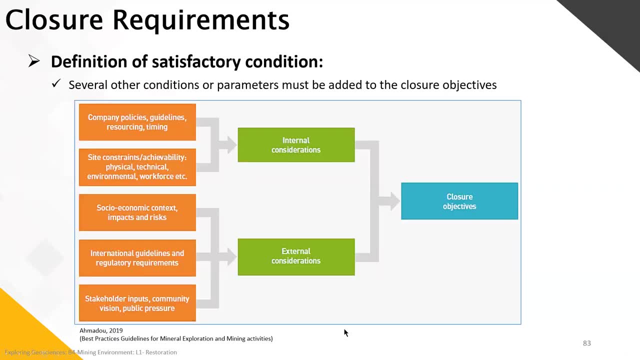 So this is the major thing to remember too- That of course, it will never come back to its initial state, but it will come back to a satisfactory state That will be used for future purposes. Several other conditions or parameters must be added to the closure objectives. 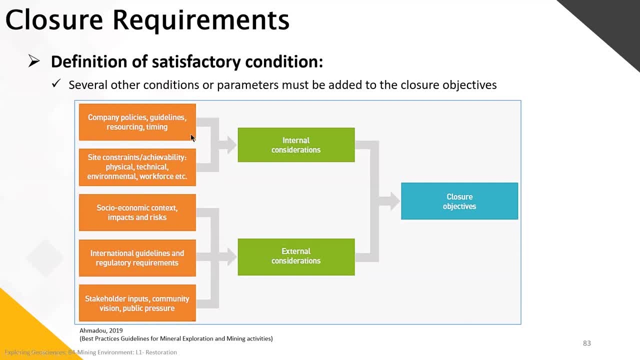 So it must include the company policies guidelines, resource, timing. These are separated into the internal, so the company's considerations, versus the external considerations. So the internal is the company's policy policies guidelines, resourcing, timing and the site constraints, the physical, technical, environmental. 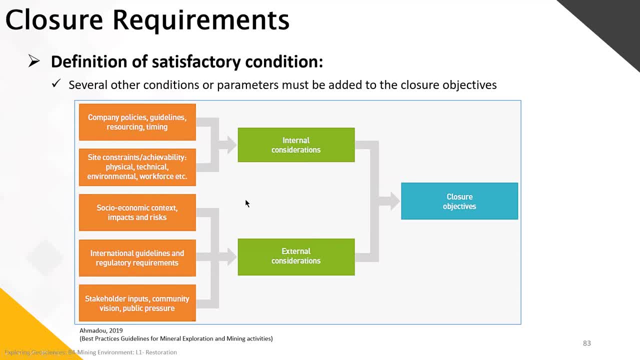 and workforce, and so on. For the external, it needs to take into consideration everything that has to do with the socio-economic context: impacts and risks to the local communities, the international guidelines and regulatory requirements and, finally, the stakeholders' inputs. community. 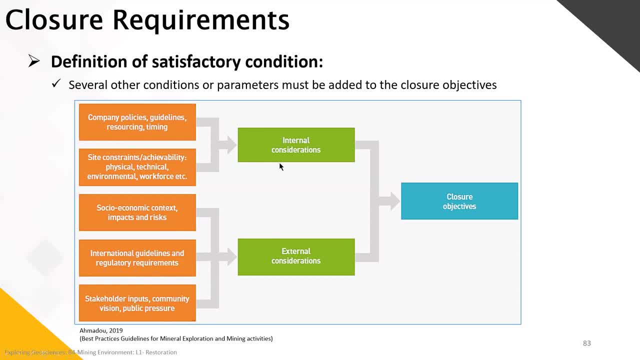 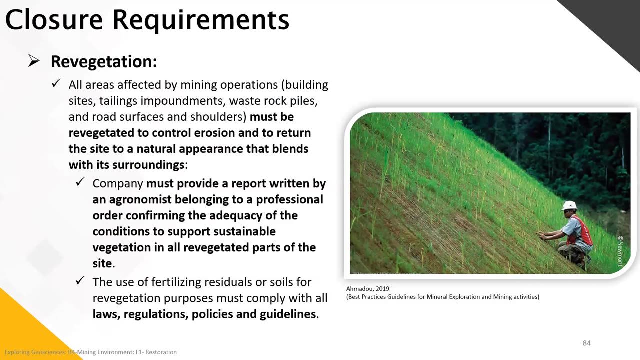 and vision, public pressure. So both considerations- and internal, external, will go into the closure objectives. The re-vegetation is considered as all areas affected by mining operations, including the building sites, the tailing impoundments, the waste, rock files and road. 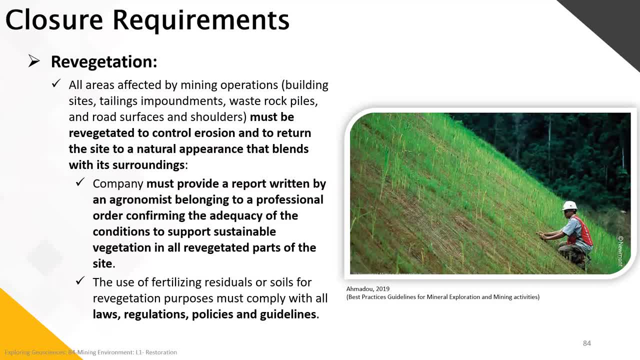 surfaces and shoulders. They must be re-vegetated to control erosion and to control and to return the site to a natural appearance That blends with its surroundings. So natural appearance blending with its surroundings, That's two key terms here. The company must provide a report written by an agronomist belonging to a professional. 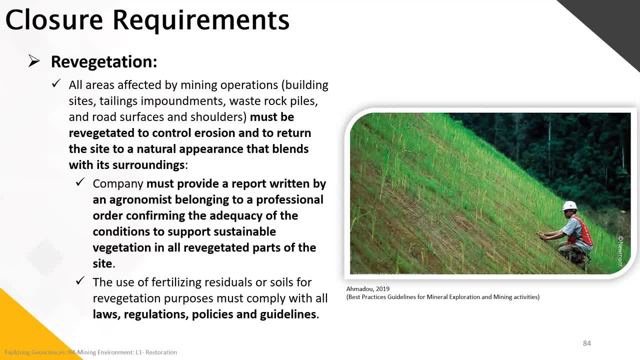 order confirming the adequacy of both conditions to support sustainable vegetation in all re-vegetated parts of the site and the use of fertilizing residuals or soils for the re-vegetation purposes must comply with all laws, regulations, policies and guidelines. 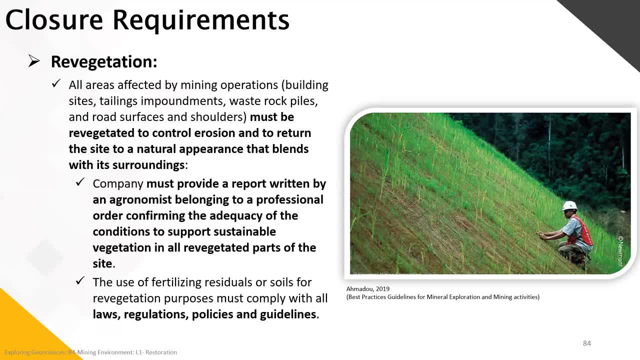 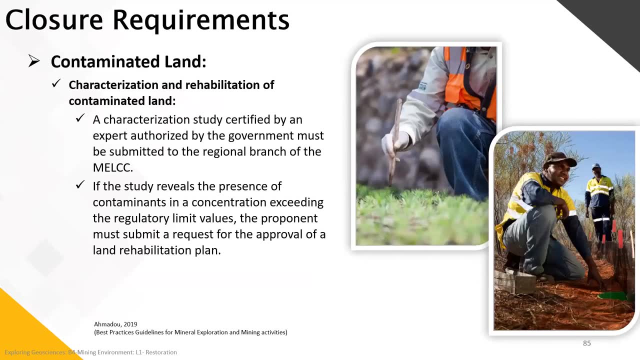 So this again, we need a professional to say that the work has been done using all the right methods and the results are satisfactory For the contaminated land. we need to characterize and we need to characterize and we need to re-evaluate the contaminated land. 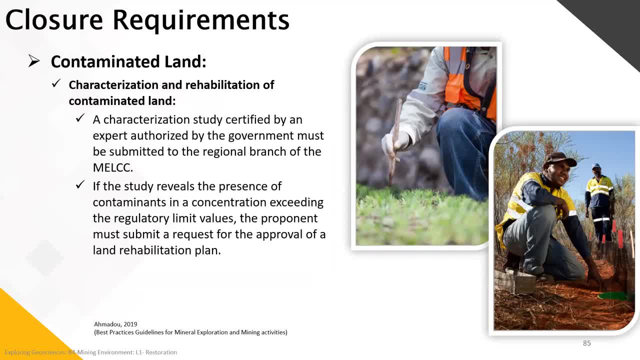 So a characterization study certified by an expert authorized by the government must be submitted to the regional branch of the MILC. If the study reveals the presence of contaminants in a concentration exceeding the regulatory limit values, the proponent must submit a request for the approval of a land rehabilitation. 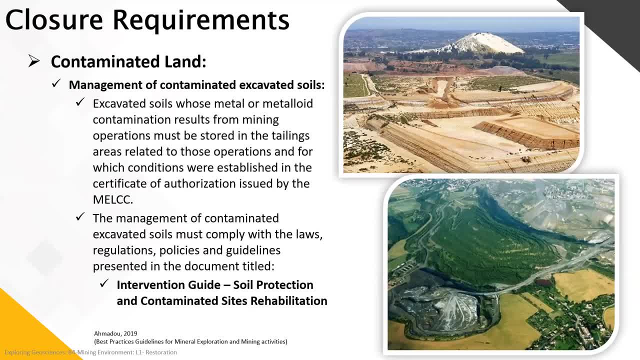 plan. The management of contaminated excavated soils must include: excavated soils whose metal or metalloid contamination results from mining operations must be stored in the tailings areas related to the operations and for which conditions were established in the certificate of authorization issued by the MILC. The management of contaminated excavated soils must: 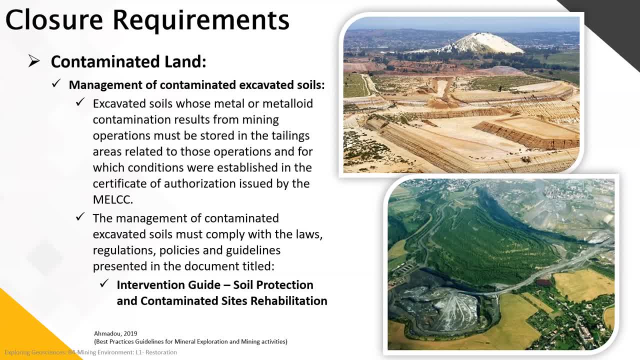 comply with the laws, regulations, policies and guidelines presented in the document called the Interaction Guide: Soil Protection and Contaminated Sites Rehabilitation. So again, we need to move from the operated mining site, possibly contaminated land, to a complete re-vegetalized area which complies with the environmental 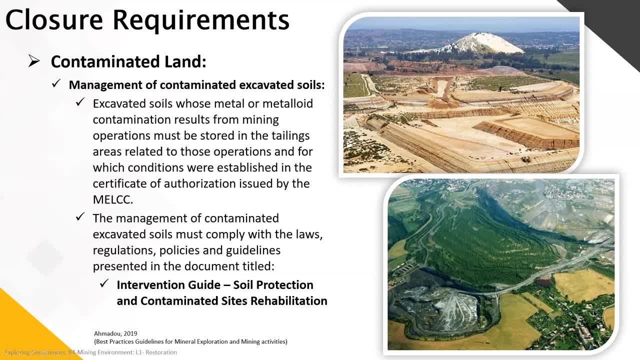 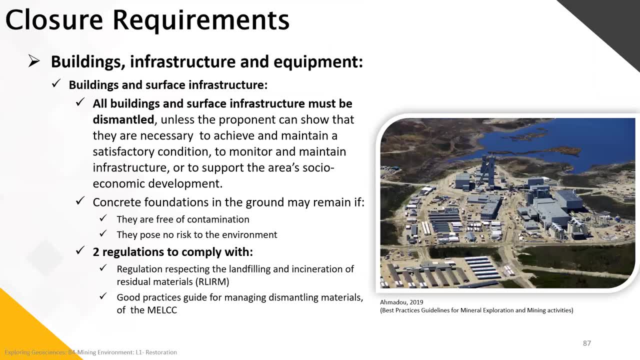 look and characteristics For the buildings, infrastructure and equipment. the buildings and surface infrastructure: all the buildings and surface infrastructure must be dismantled unless the proponent can show that they are necessary to achieve and maintain a satisfactory condition, to monitor and maintain infrastructure or to support the areas. 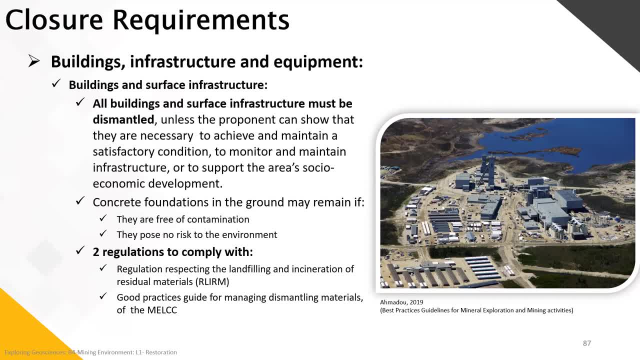 in addition to the environmental and social economic development, All the concrete foundations in the ground may remain if they are free of contamination and if they pose no risk to the environment. Two regulations to comply with. we have the regulation respecting the land filling and incineration of residual materials. 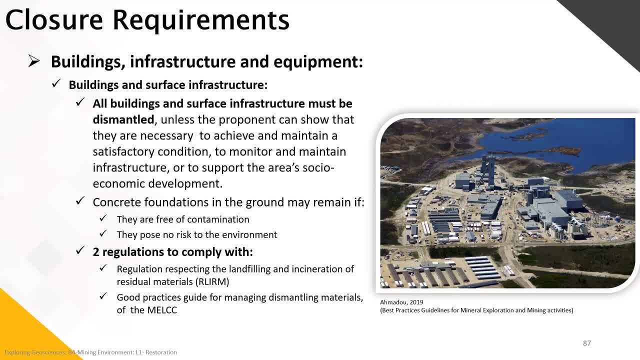 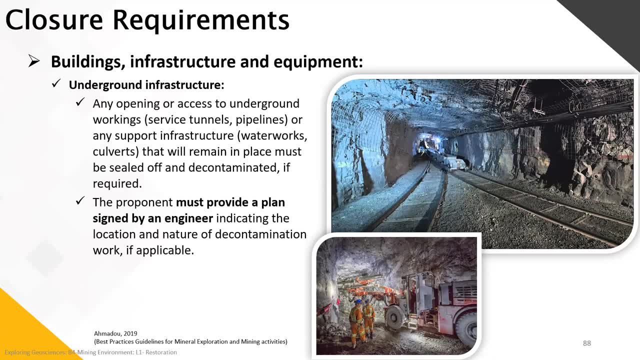 and the good practices guide for managing dismantling materials of the MILC For underground infrastructure. any opening or access to the underground workings, service tunnels, pipelines, drifts or any support infrastructure waterworks culverts that will remain in place must be sealed off and decontaminated if required. The proponent. 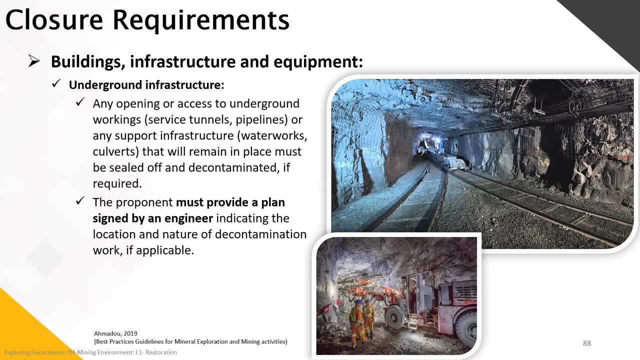 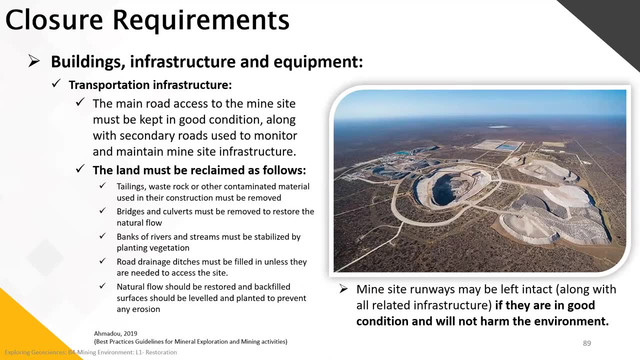 must provide a plan, signed by an engineer, indicating the location and nature of decontamination work. if, if some of the variousasz not applicable, The transportation infrastructure—again the main road access to the mine site must be kept in good condition along secondary roads used to monitor and maintain the mine site infrastructure. 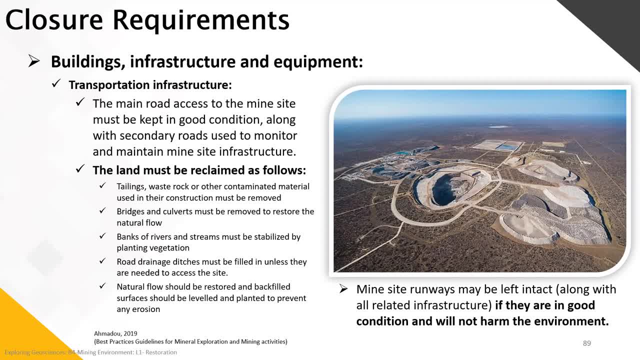 The land must be reclaimed as follows: The tailings, waste, rock or other contaminated material used in their construction must be removed. Wr�بات عliner Alfρس removed to restore the natural flow of any water banks. The banks of rivers and streams must be stabilized. 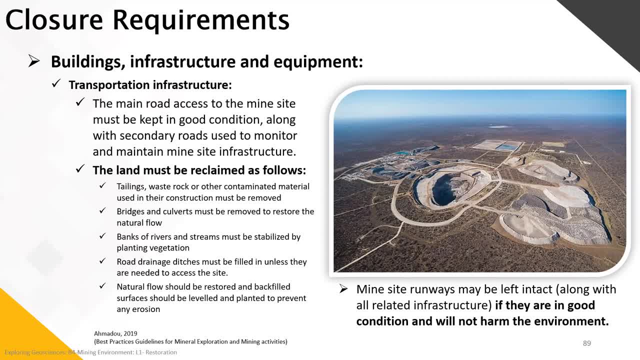 by planting vegetation. The road drainage ditches must be filled in unless they are needed to access the site, And the natural flow should be restored, and backfield surfaces should be leveled and planted to prevent any erosion, So the mine site runways may be left intact. 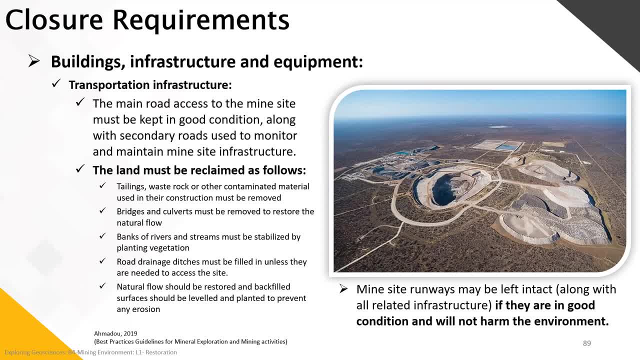 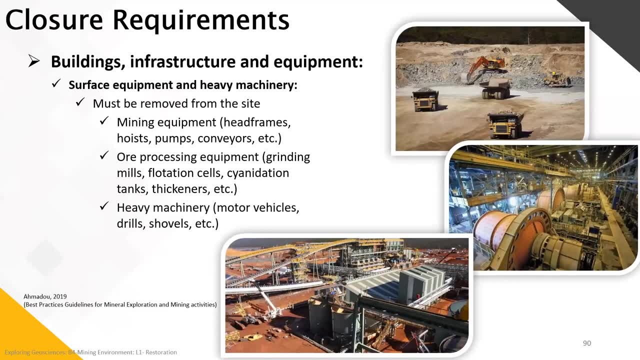 along with all related infrastructures, if they are in good condition and will not harm the environment. All the surface equipment machinery. now they must be removed from the site. All the mining equipment: head frames, hoists, pumps, conveyors, et cetera. 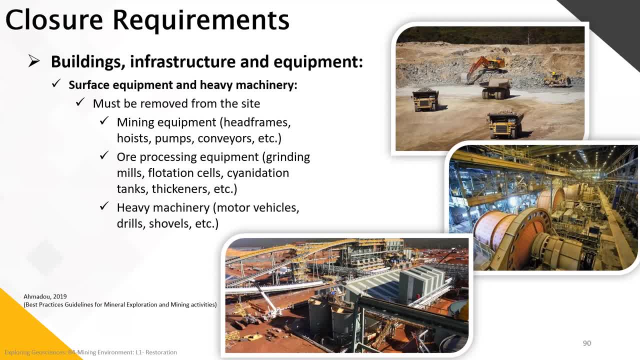 All the ore processing equipment, the grinding mills, the precipitation cells, the cyanidation tanks, the thickeners, et cetera. All the heavy machinery, the motor vehicles, the drills, the shovels, blah, blah, blah, et cetera. 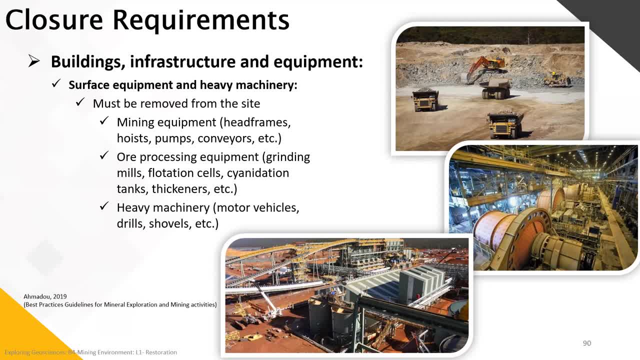 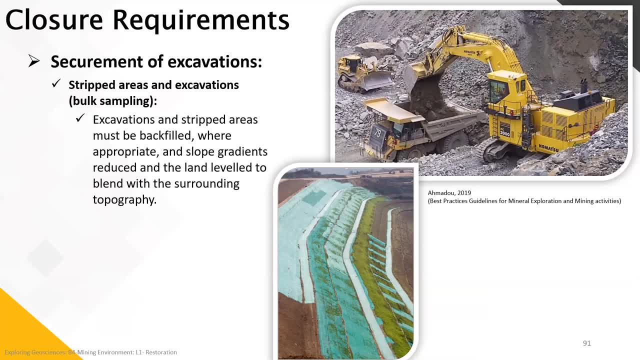 All that. they must all be removed from the site. The strip areas and excavations, for example for a ball. something has to be put back as much as possible to a natural topography of the area. So the excavations and strip areas must be backed. 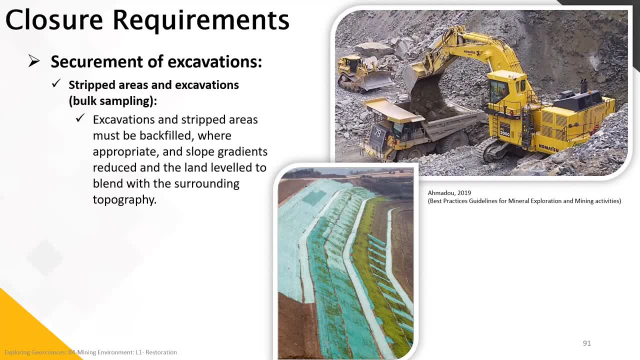 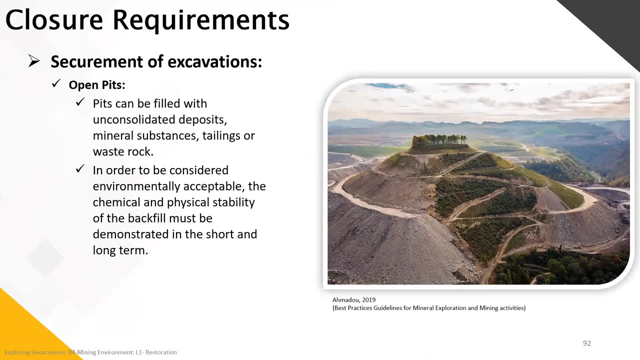 filled where appropriate and slope gradients reduced and the land level to blend with the surrounding natural topography For the open pits. the pits can be filled with unconsolidated deposits, mineral substances, tailings or waste flow In order to be considered environmentally acceptable. the chemical and 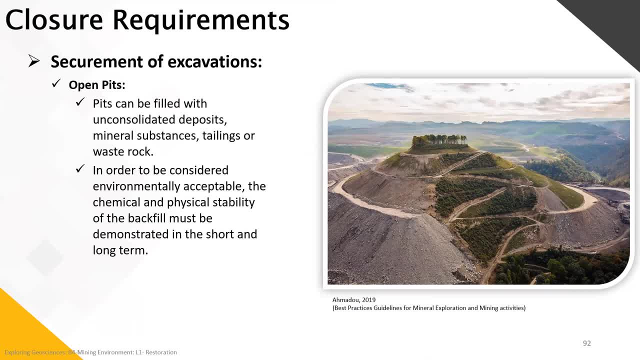 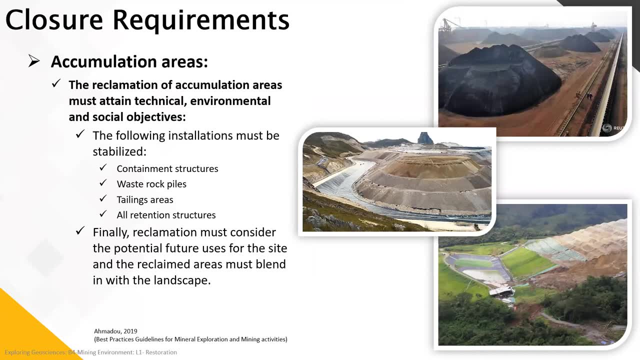 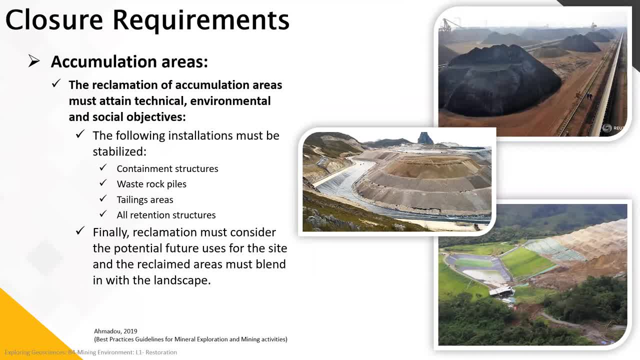 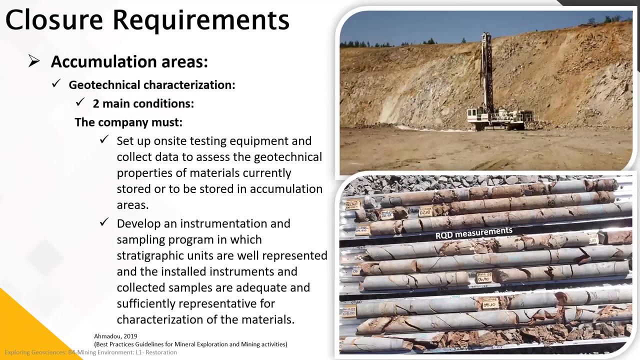 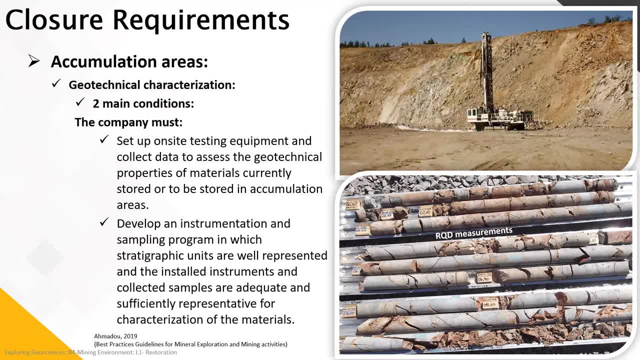 waste-pollutants. the waste-pollutants and the reclaimed areas, the tailings ofization and all retention structures. And finally, the reclamation must be considered by potential, have their geotechnical characterization using two main conditions: The company must set up on-site testing equipment and collect data to assess the geotechnical properties of materials. 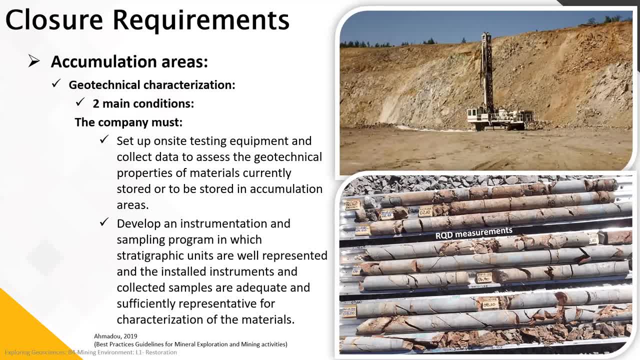 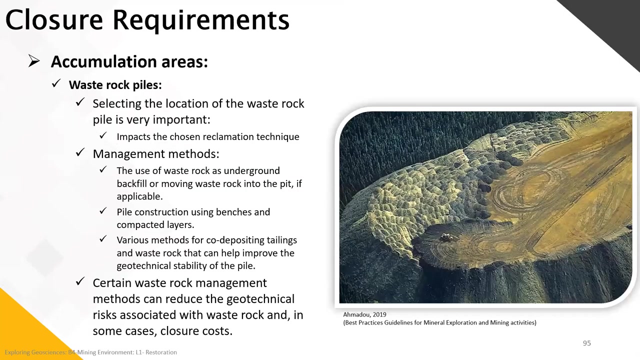 currently stored or to be stored in an accumulation area, And they must develop an instrumentation and sampling program in which stratigraphic units are well represented and the installed instruments and collected samples are adequate and sufficiently representative for the characterizations of the materials, and these mainly include the RQD measurements. 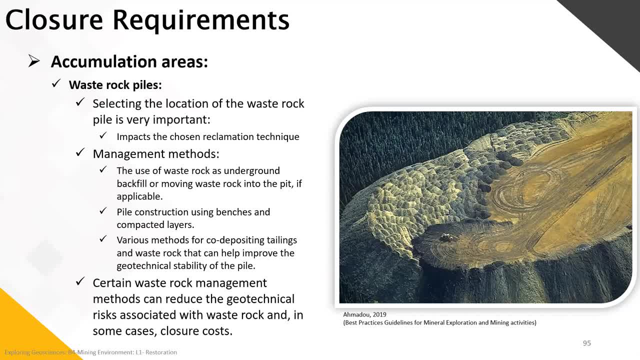 For the waste rock piles. selecting the location of waste rock piles is very important. It impacts the chosen reclamation techniques. The management methods of these waste rock piles is either to use the waste rock as underground backfill or moving waste rock into the pit, if applicable. 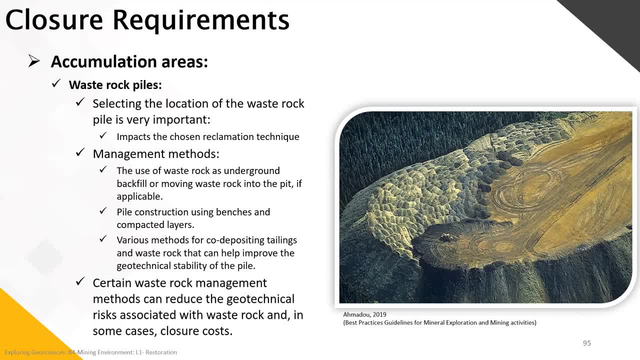 The pile, construction using benches and compacted layers, and the various methods for co-depositing tailings and waste rock that can help improve the geotechnical properties. This is to reduce the liability of the pile by mixing two tailings or waste rock. 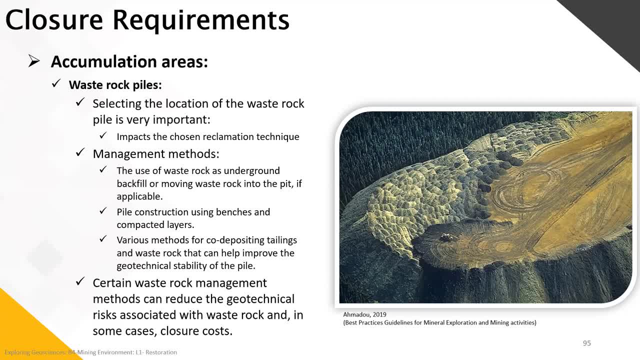 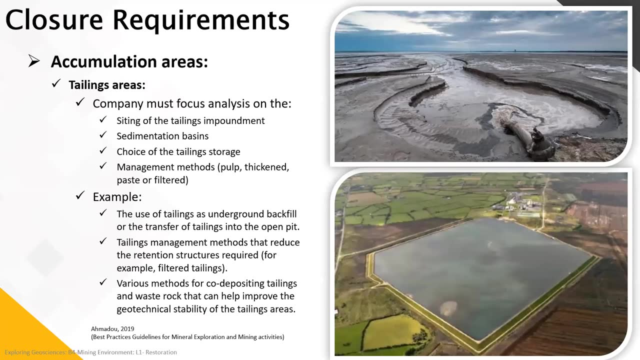 Certain waste rock management methods can reduce the geotechnical risks associated with waste rock and, in some cases, closure costs For the tailing areas. the company must focus their analysis on the siding of the tailings' impoundment, the sedimentation facets. 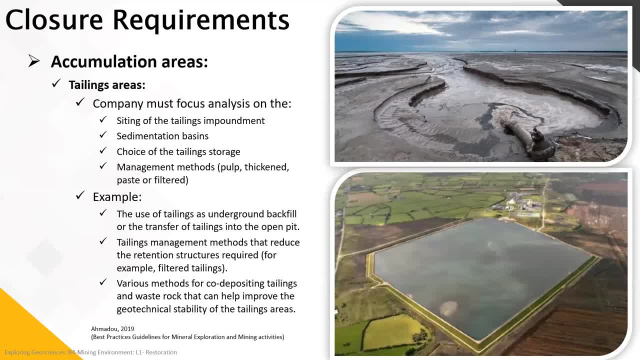 acids. the choice of the tailings storage and the management methods for use: either pulp, thickened paste or filtered Example. the use of tailings as underground backfill or the transfer of tailings into the open pit. The tailings management methods that reduce the retention structures. 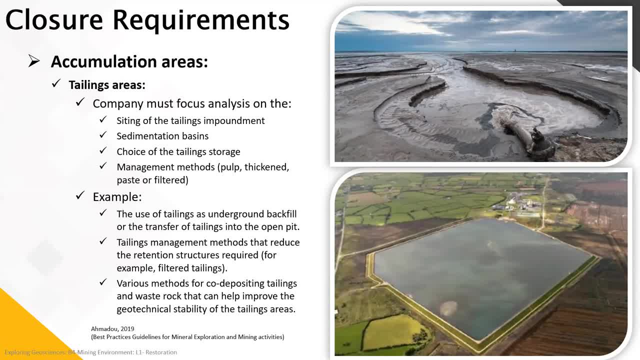 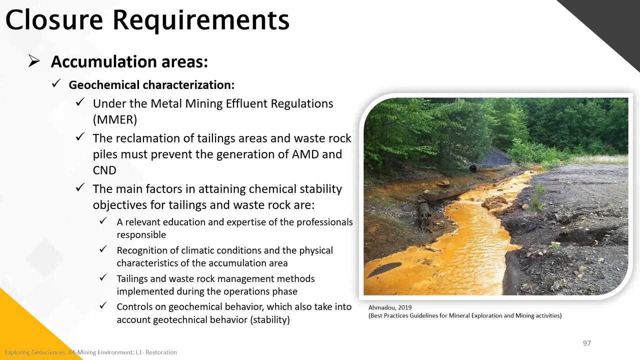 required, for example, filtered tailings and various methods for co-depositing tailings and waste rock that can help improve the geotechnical stability of the tailings areas. The geochemical characterizations of these accumulation areas under the metal mining influence regulations, so they have their own legislation. the reclamation of the 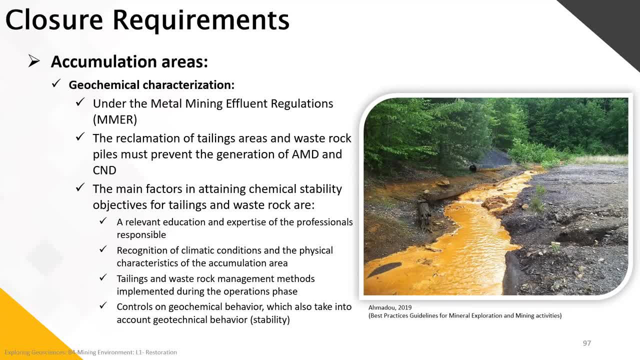 tailings areas and waste rock piles must prevent the generation of acidic mining drainage and the natural deneutral mining drainage. The main factors in attaining chemical stability objectives for tailings and waste rock are either a relevant education and expertise of professionals responsible, the recognition of 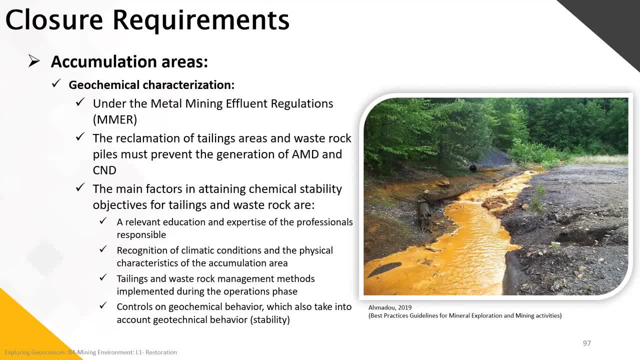 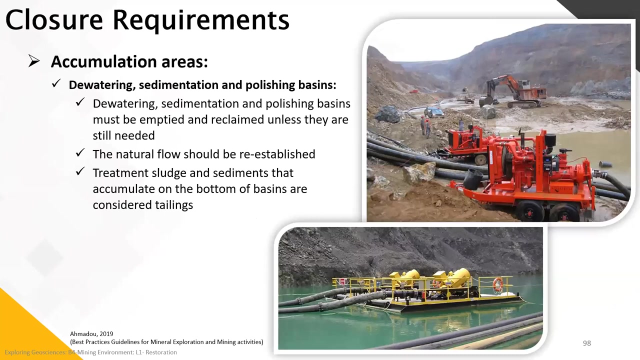 climatic conditions and the physical characteristics of the accumulation area, tailings and waste rock management methods implemented during the operation. The geochemical behavior, which also takes into account the geotechnical behavior or the stability of the accumulation areas, Dewatering, sedimentation and pollution facets. so the watering, sedimentation, pollution. 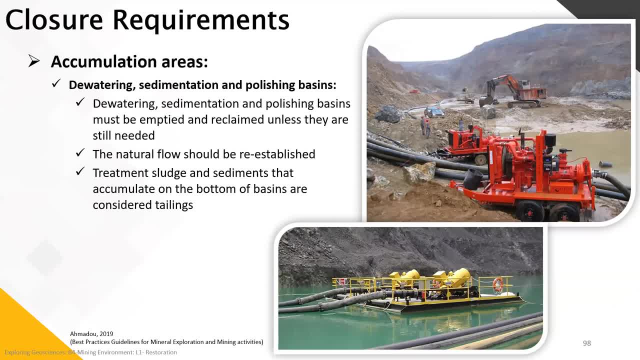 facets must be emptied and reclaimed unless they are still needed. The natural flow should be reestablished within the area using the natural topography of the area, and the treatment sludge and sediments that accumulate on the bottom of the basins are considered to be tailings. 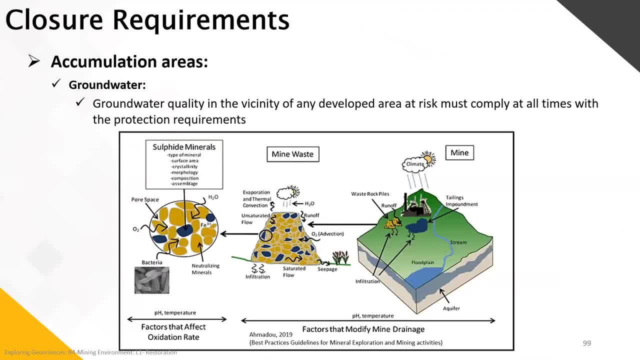 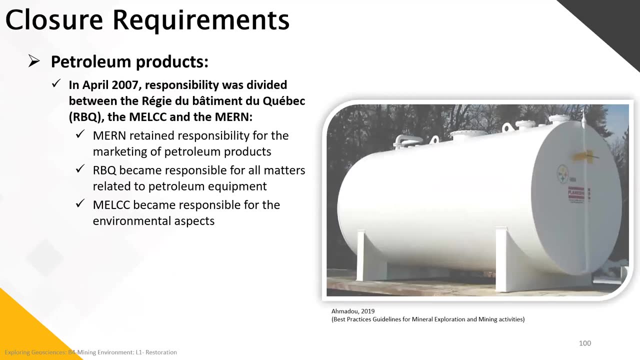 For the groundwater, for the groundwater quality in the vicinity of any developed area at risk, must comply at all times with the protection requirements. A little bracket here for the petroleum industry, Petroleum products, just to note that these legislations the responsibility of the petroleum. 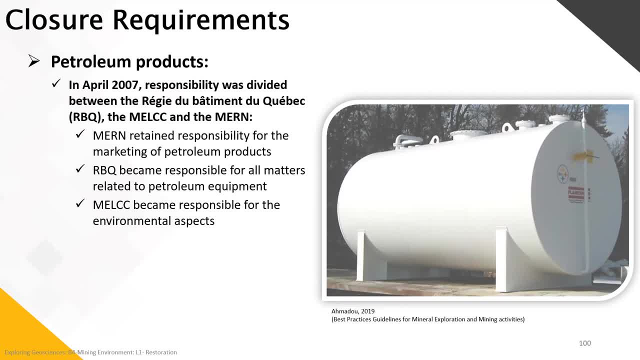 industry has been divided into April 2-7 between the RBQ- Régime du Petit Mer du Québec- the MELC and the MERN. The MERN will take the responsibility for the marketing of the petroleum products, While the RBQ becomes responsible for all matters related to petroleum equipment and the MELC becomes. 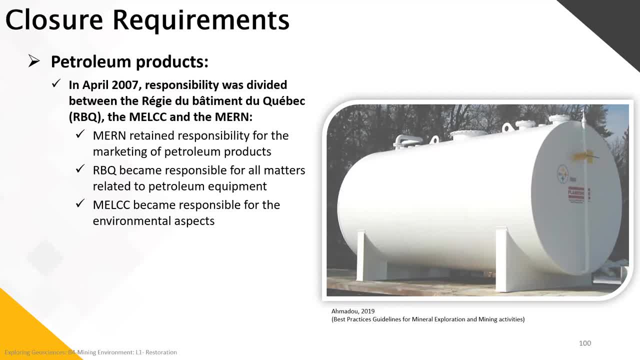 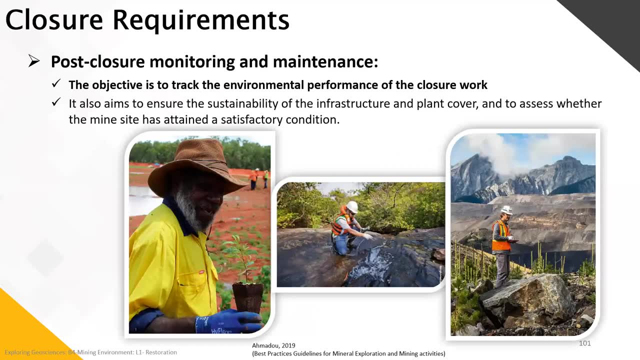 responsible for the environmental aspects of the petroleum industry. Moving on to the post-cooler monitoring and maintenance, that is also very important because, as much as a company wants to make the best work, some times some non-seen or unobserved interpretations lead to future contamination without. 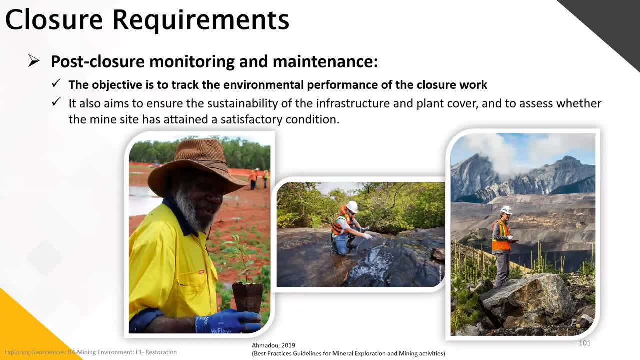 the company knowing if there is no tracking for medium, short, medium and long term time. So the objective is to track the environmental performance of the closure work. It also aims to ensure the sustainability of the infrastructure and plant cover and to assess whether the mine site has attained a satisfactory condition. 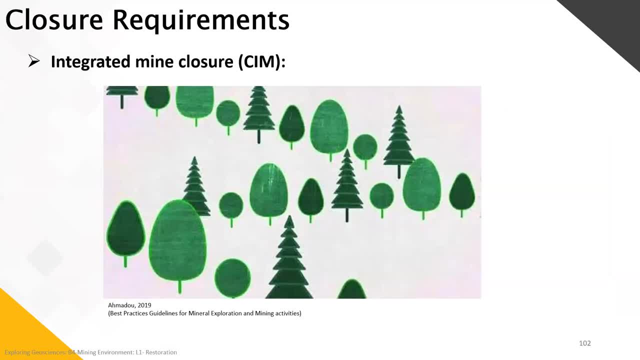 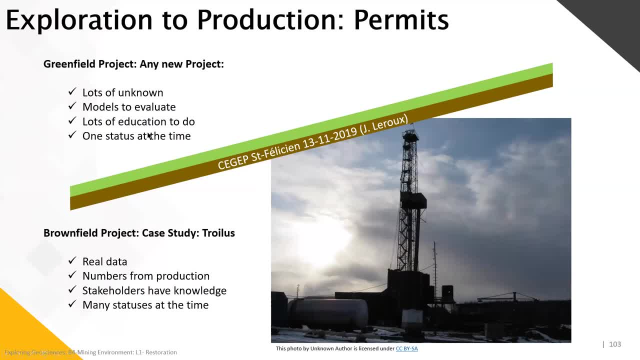 you have many models to evaluate. you have lots of education to do and you are doing or moving on one status at a time When you move on into a brownfield project. you have real data from your study, you have numbers from production, you have stakeholders that have knowledge and you have 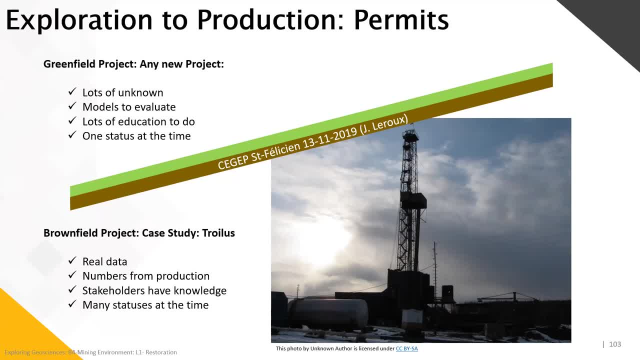 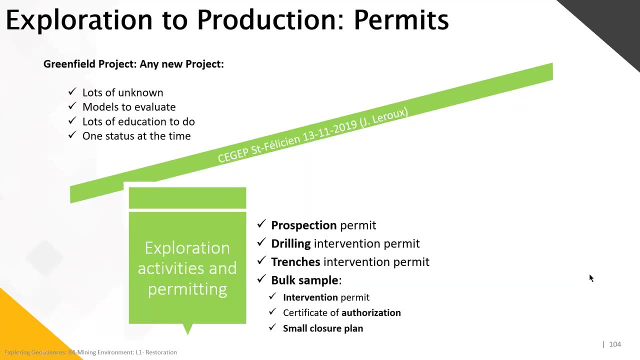 many statuses at the same time. Basically, when we use the term brownfield, that means we are within a mining project or a mature mining camp. Example, moving on with the UK study of Troilus. So when it was at its exploration, greenfield prospection state. 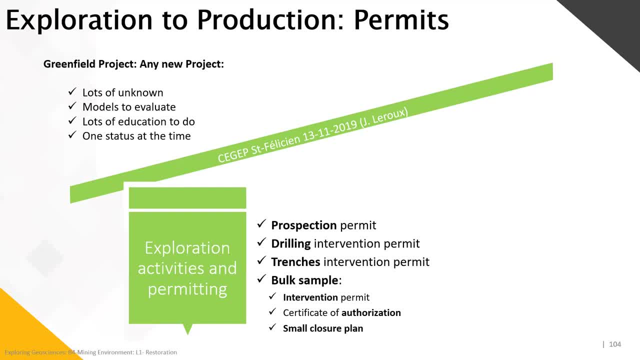 the permitting that was needed to move on this project was prospection permit, drilling iteration permit, trenches iteration permit. Once the discovery was done and we needed to have future studies to make sure that this deposit would move on to a OR state or a OR ranking, we needed to do some bulk sampling. So 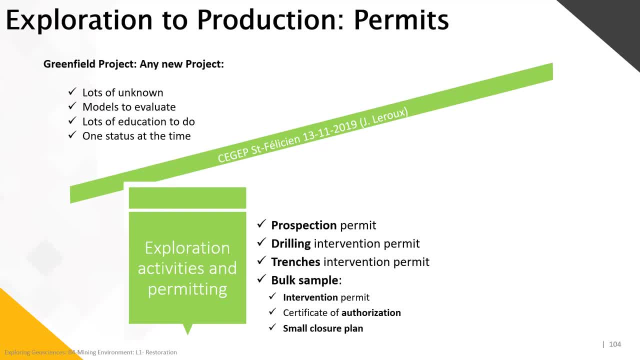 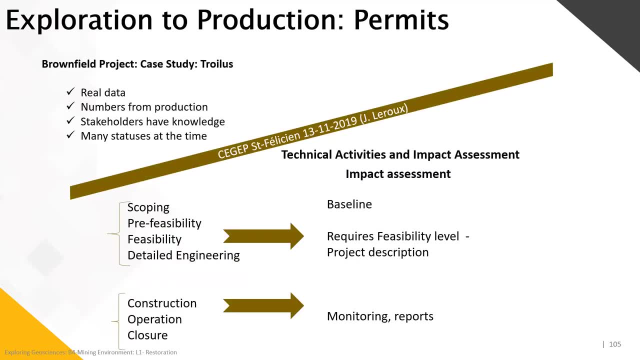 the bulk sampling. we did some bulk sampling. we did some bulk sampling, we did some bulk sampling. we needed the iteration permit, the certification of authorization and a small closure plan. Once we move on to the brownfield test, we have technical activities and impact. 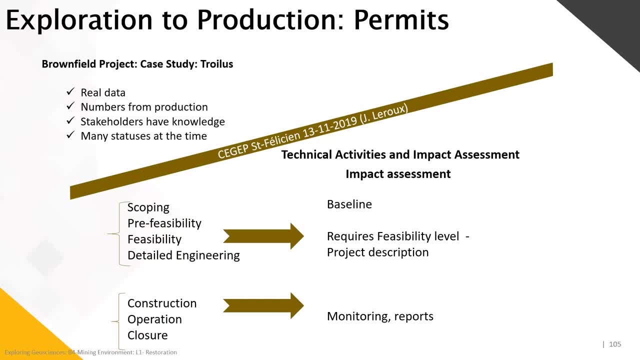 assessment. so we're moving on from scoping to pre-feasibility, to feasibility, to detailed engineering- and that requires the feasibility level, project assessment description- And moving on to the construction, operation and closure of the mining each. 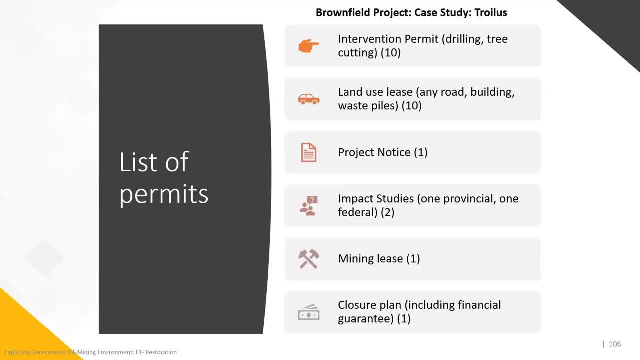 needs the monitoring reports. Example for the Troilus case study, we have the list of permits that were needed to move on from an exploration project to a mining project. We needed, of course, the first intervention permits, including the drilling the tree. 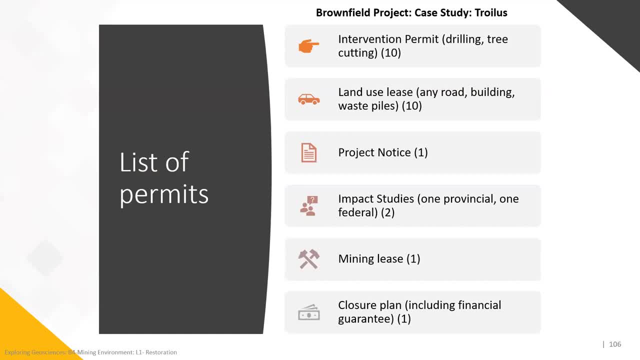 cutting, etc. We needed the land use lease for any road building waste pile. We needed to have a project notice. We needed to have studies, impact studies, both for the provincial and federal government. We needed to have the mining lease. Then we needed to have the 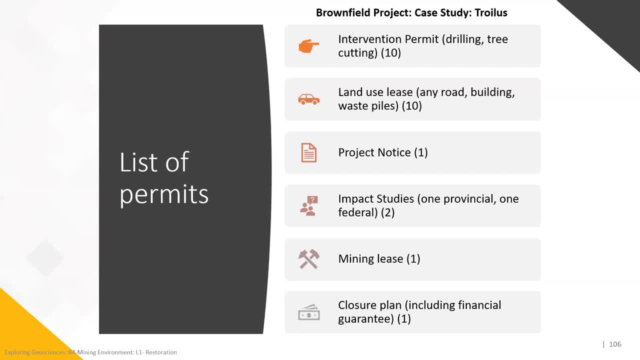 closure plan including all the financial guarantees budgets. Finally, we had FONA permits. We also had archaeology permits. Archaeology permits for us, mainly in Quebec and Canada, are for the surface and subsurface studies, where we have archaeological teams coming in and digging for some artifacts that can be found within an area. 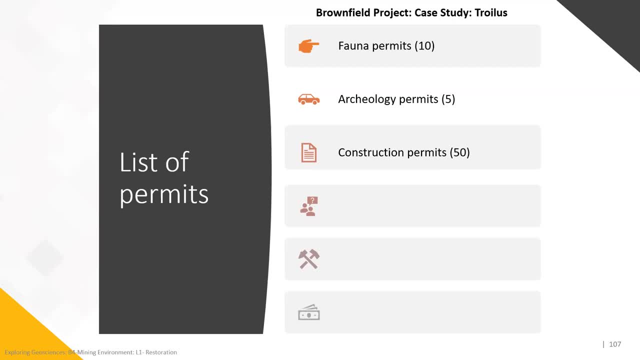 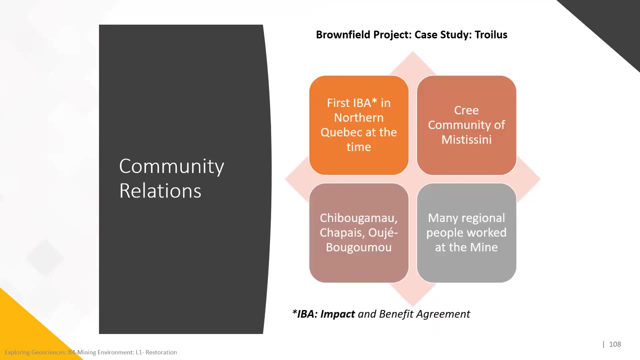 so that it is done prior to the mine construction, so that these are not lost. Finally, we have the construction permits. Example here from the case study for Troilus. it was one of the first to have built community relations. It was the first IBA in northern Quebec at the time. 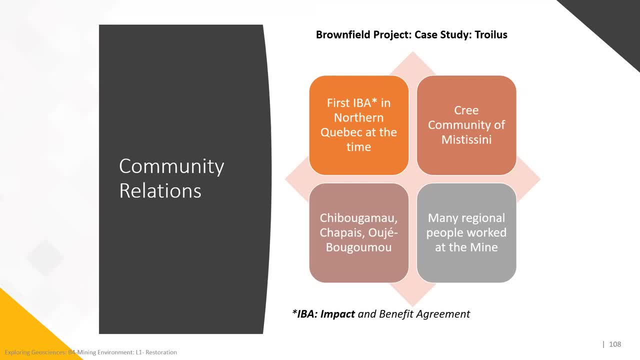 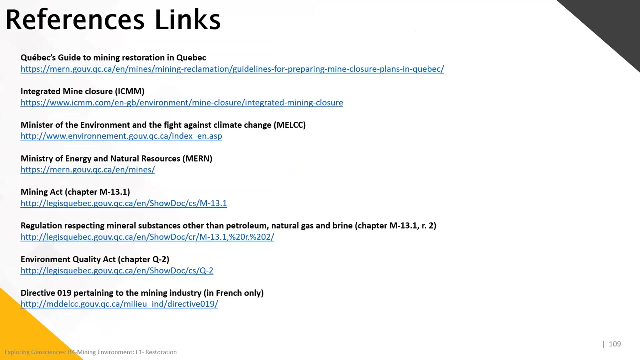 It was an impact and benefit agreement with the First Nation population. It was an agreement with the Cree community of friendliness but it also included the Gitgemo statue and And many regional people worked at the mine. All the PDF files I have given to Charles for this study. 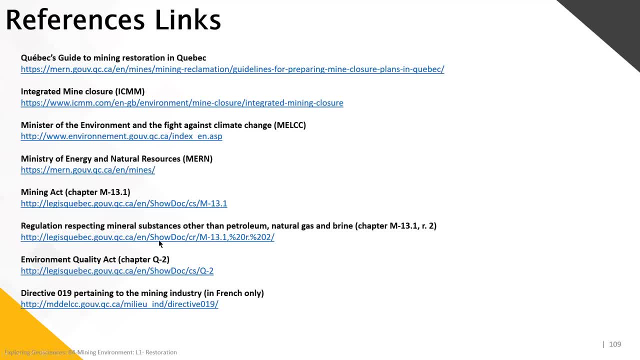 for this lesson. I've also included their own links, their website links, and I've also included their PDF file formats, if you are interested. So these include the Quebec's guide to mining restoration in Quebec, the integrated mine closure from the CIM, the minister of environment. 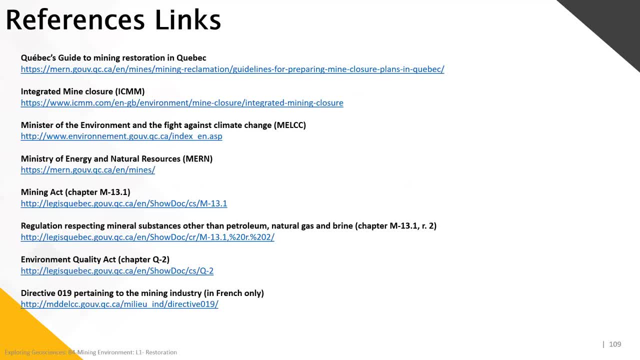 and fight against climatic change website. the ministry of energy and natural resource website. mining act. the regulation and respecting mineral substances other than petroleum, natural gas and wine- chapter from the legislation. the environment quality act and, finally, the directive pertaining to the mining industry. 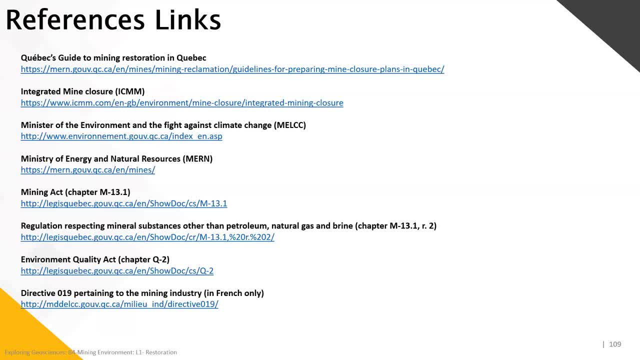 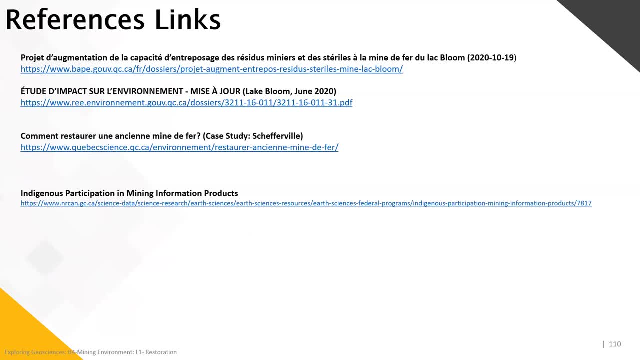 Unfortunately, for now it is mainly only available in French. I've also included some references for specific actual environment impacts that we hear in the news. First two for the iron lake bloom area and the third one is for the red waters from the Sheckerville area. 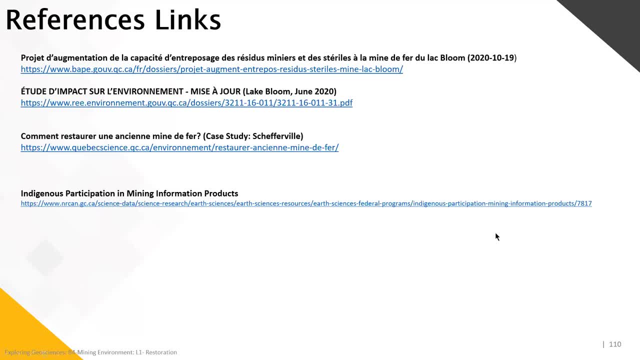 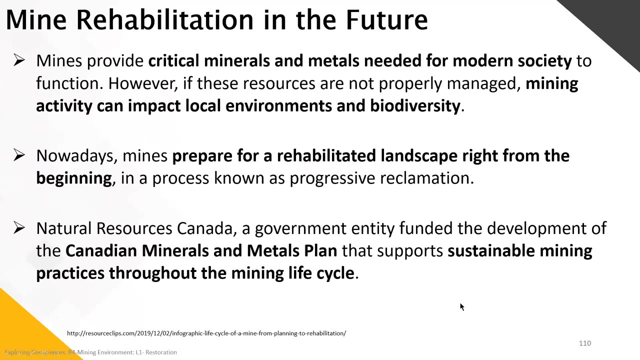 And finally, I've included the website that lists a lot of programs and knowledge that impacts the participation of first nations within mining companies or mining projects. And before showing you an example video of a real invitation for a gold mine, just wanted to move on and show the mine revelation in the future. 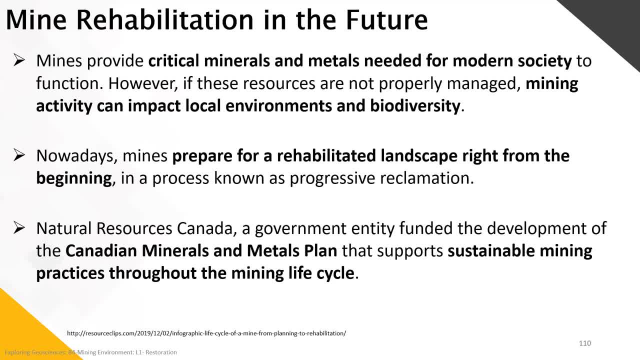 Just wanted to move on and show the mine revelation in the future, Which is taken very seriously to prevent any of the historical horror stories. And I've included all of the main PDFs for these files too. So these show that the mines, as we all know. 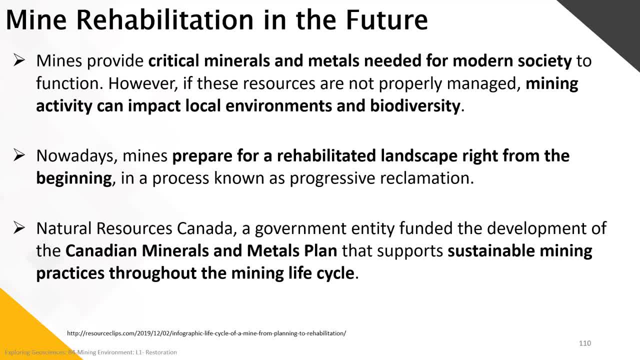 provide the critical minerals and metals needed for modern society, but these resources are not properly damaged And the mining activity can impact local environments and biodiversity if they don't follow the legislation, and biodiversity if they don't follow the legislation. Nowadays, the mines prepare for rehabilitated landscape. 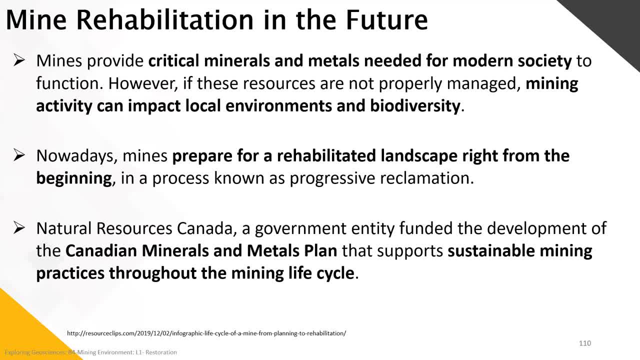 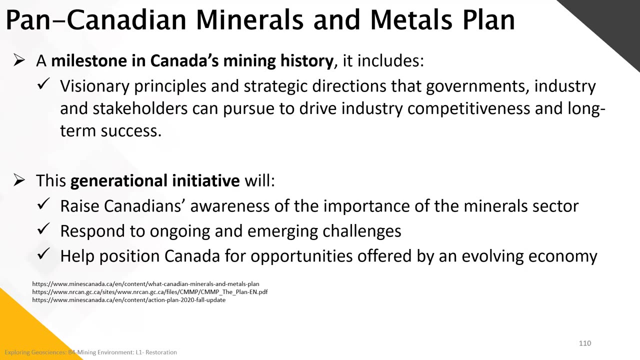 right from the beginning in a process known as progressive reclamation. So the Natural Resource Canada government funded the development of what is called the Canadian minerals and metals plant And that supports all the natural resource sustainable mining practices throughout the mining life cycle. It is a milestone in Canada's mining history because it includes visionary principles and 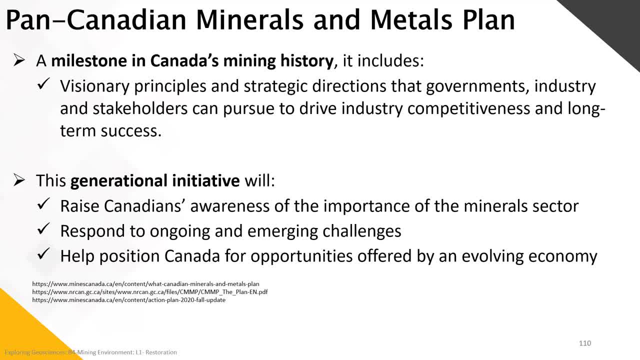 strategic directions that governments, industry and stakeholders can pursue to drive industry competitiveness and long-term success. This is a generational initiative and will raise the Canadians awareness of the importance of the mineral sector. It will respond to ongoing and emerging challenges for all its impacts on the communities and it will help position 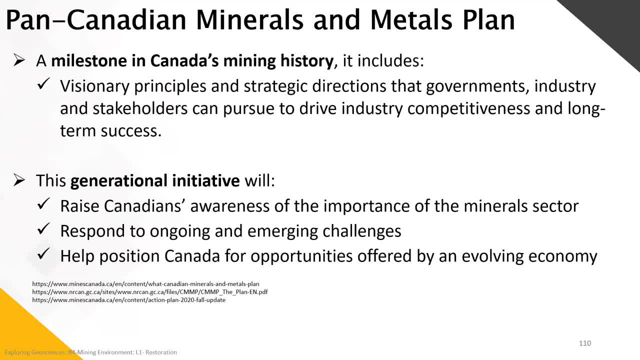 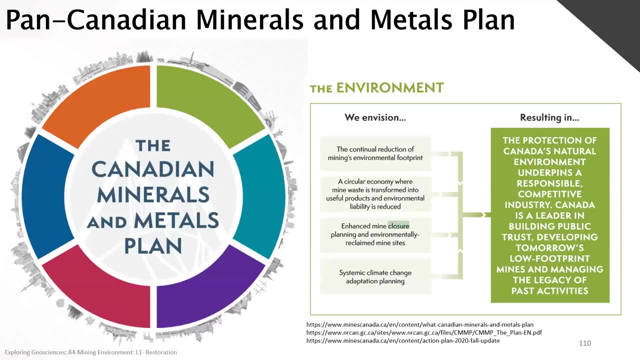 Canada for opportunities offered by an evolving economy. So I have included the links to either the websites or the web, also the documents, PDF slides. So the main: the Canadian minerals and mineral plans have extracted some of the main chapters. just a little summary. So for the environment, what they see is a continual reduction of mining. 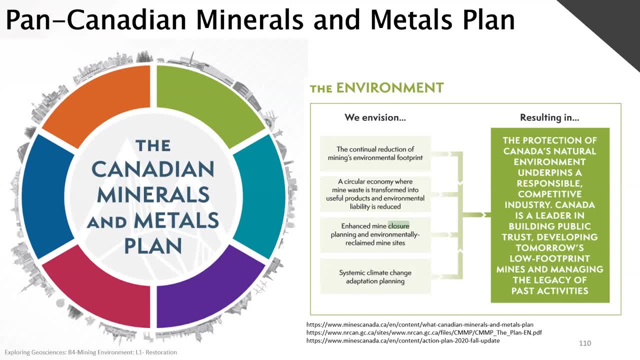 environment footprint, a circular economy where mine waste is transformed into useful products and environmental liabilities reduced, enhanced mine closure planning and environmentally reclaimed mine sites, and the systematic climate change adaptation planning, And all this to their goal for protection of Canada's natural environment, underpins a responsible, competitive industry. Canada is 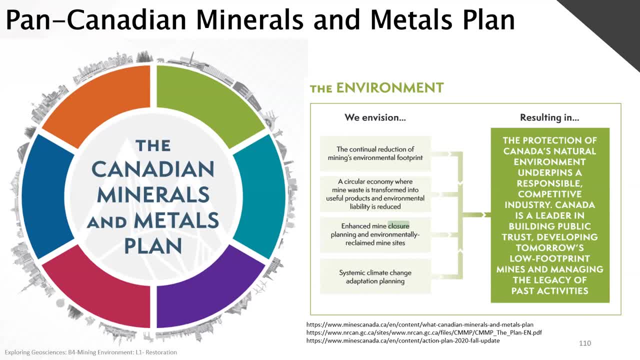 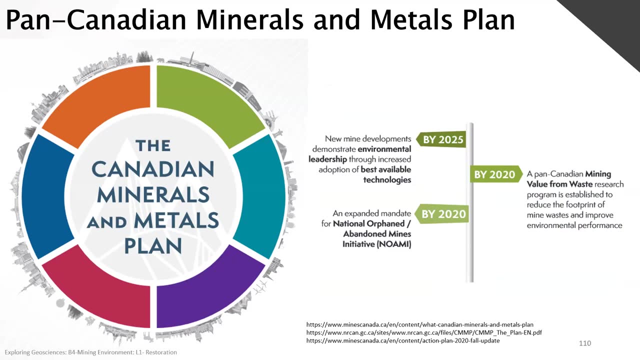 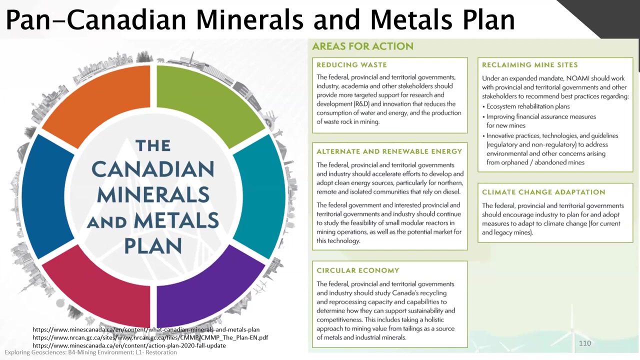 a leader in building public trust and developing tomorrow's low footprint mines and managing the legacy of fast activities. They have a vision. It was started in 2012.. 2019 and they have a planned vision through 2025.. These areas of action include the reducing of waste, the alternative and renewable energy. 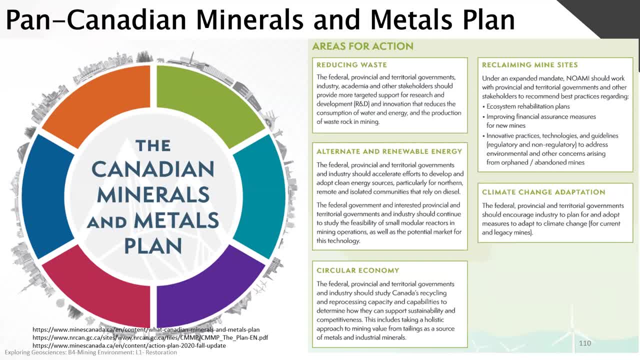 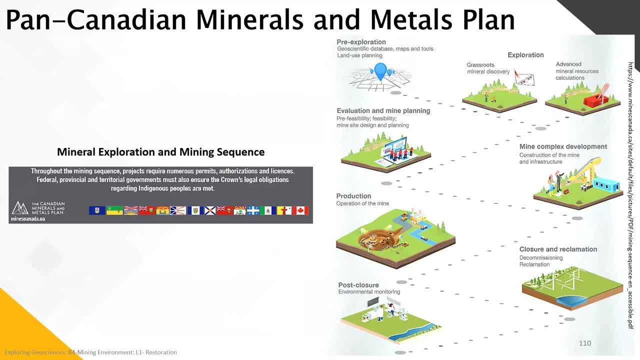 the circular economy, the reclaiming mine sites and the climate change adaptation. They also have included, based on the Lassonde curve that we've seen, the climate change adaptation. We've seen in the last lesson the mineral exploration and mining sequence, So I included. 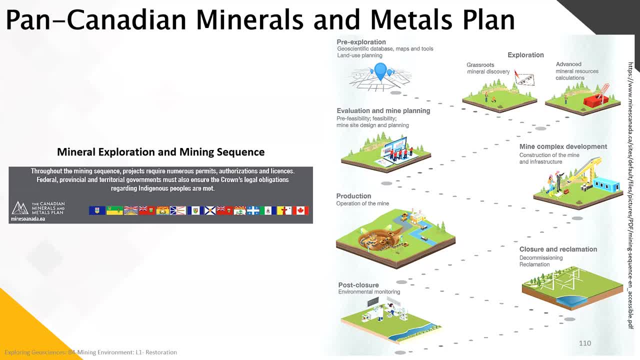 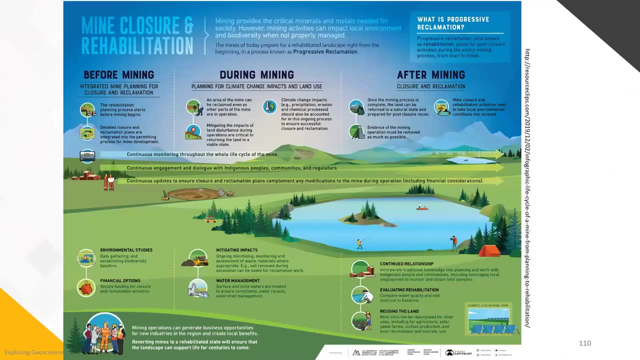 the PDF and I included just a little zoom in of the image here. So with all the steps we've seen so far, from the pre-exploration to exploration and so on, to the closure and post closure of a mine, Their mining closure and rehabilitation is also graphically well. 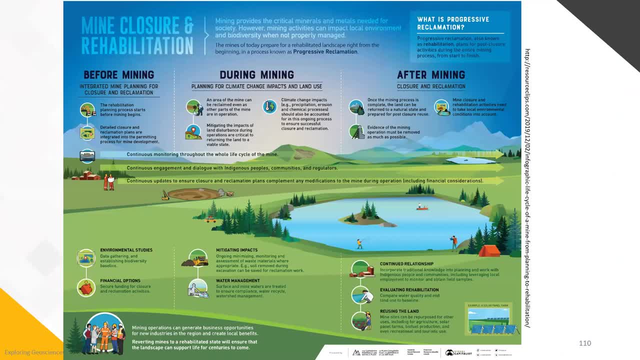 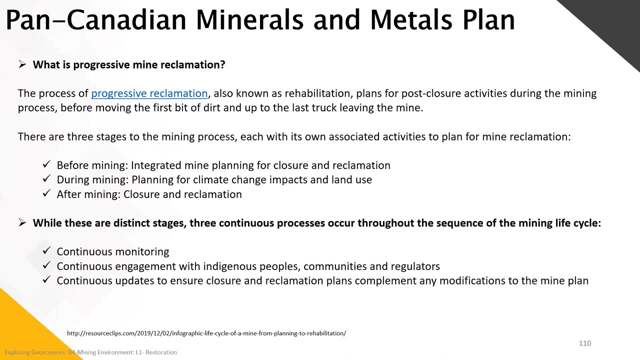 designed, as seen here, showing everything from before mining, during mining and after mining, And this comes with their long-term plan. What is progressive mine reclamation, As stated in that plan? the process of a progressive reclamation, also known as rehabilitation plans for post-closure activities during the mine process. 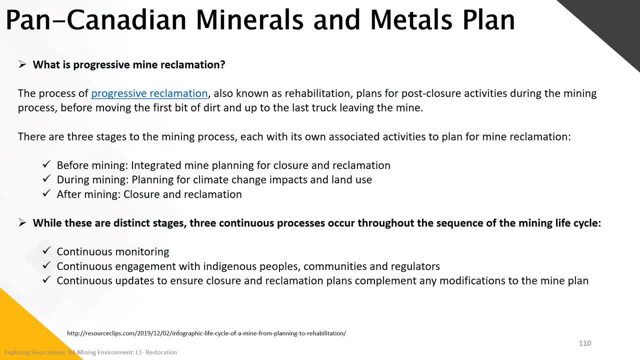 before moving the first bit of the mine out of the mine. The first step of the mine reclamation is the removal of dirt and, up to the last block, leaving the mine. So that is the big difference with the historical project. This is taken into consideration from start, during and after the project. There are 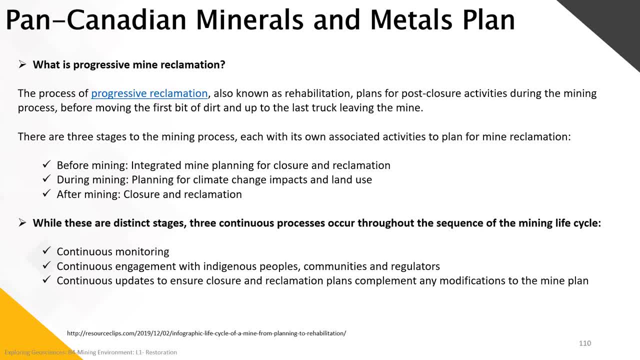 three stages to the mining process, each with its own associated activities: to plan for mine reclamation, So we have before mining, which integrates mine planning for closure and reclamation. We have during mining, so planning for climate change impacts and land use. And finally after. 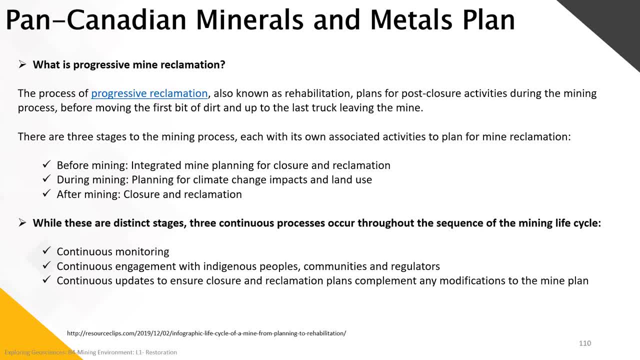 mining, the closure and reclamation processes. While these are distinct stages, three continuous processes occur throughout the sequence of the mine, the mining life cycle. We have the continuous monitoring. we have the continuous engagement with First Nation people, their communities and regulations. 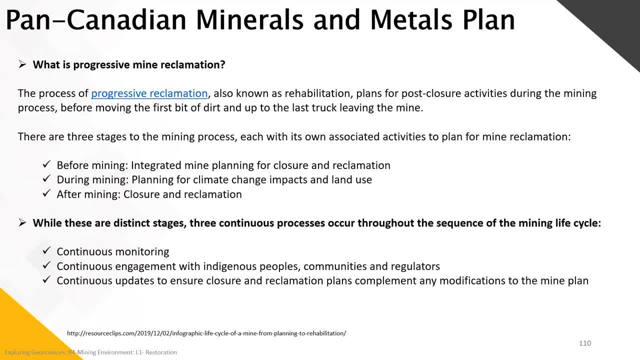 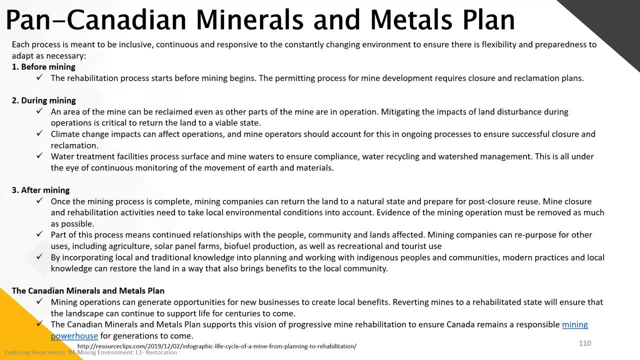 We have the continuous updates to ensure closure and reclamation plans complement any modifications to the mine plan. So these are summarized here, but again you will have the complete document if you are interested. So again, the main points for each process is meant to be inclusive. 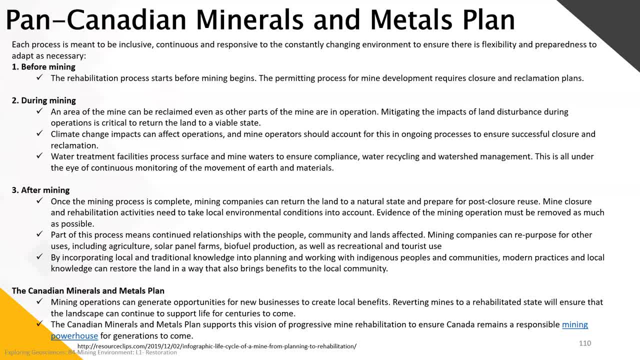 continuous and responsive to the constantly changing environment to ensure there is flexibility and preparedness to adapt as necessary for each major step before, during and after mining. Also, as seen in this lesson in the first part, for the damages and impacts. importantly, the Canadian Minerals and Metal Plans also includes mining operations. 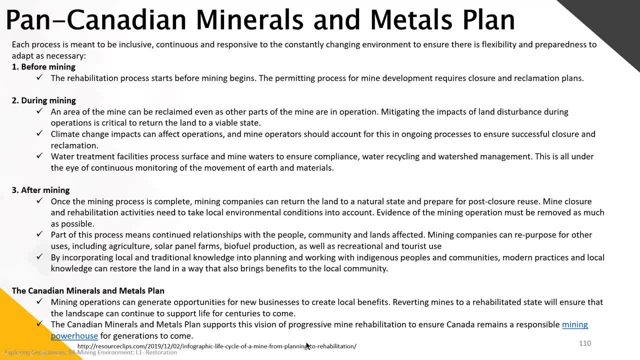 that can generate opportunities for new businesses to create local benefits. So reverting mines to a rehabilitated state will also ensure that the landscape can continue to support life for centuries to come. The Canadian Minerals and Metals Plan supports the vision to progressive mine rehabilitation to ensure Canada remains responsible mining throughout our house for. 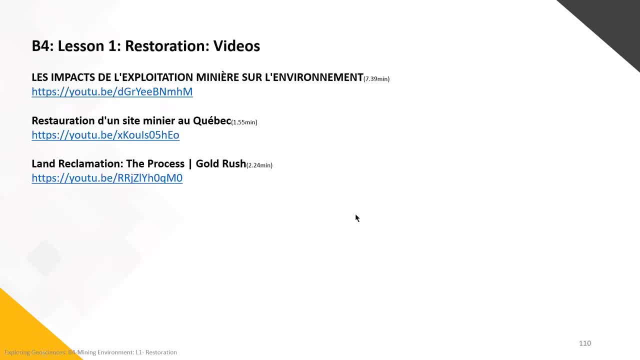 generations to come. So I've been included three videos. i'm going to show the last one today. the other two, if you are comfortable with the french speaking language, you can go and see them on your own file. we're really going to see a good example for a gold rush mining company that has shown their 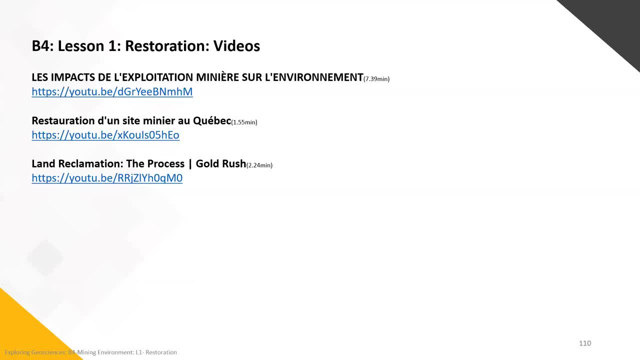 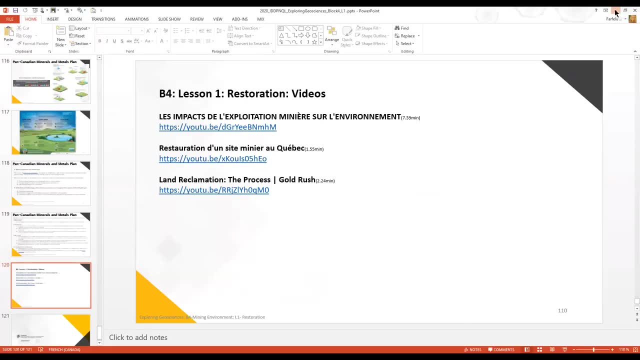 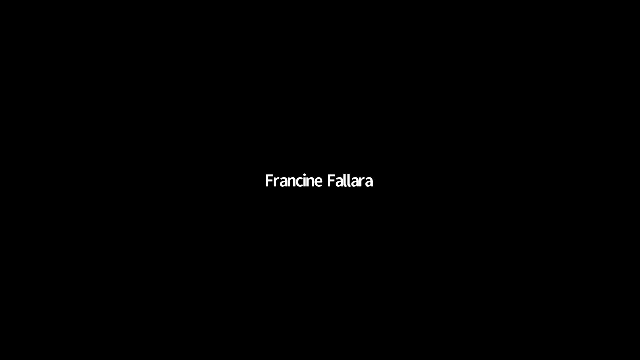 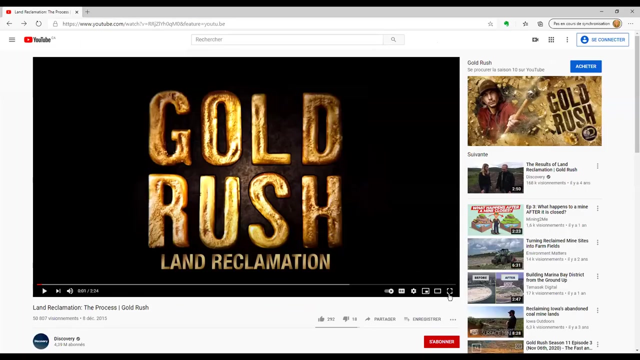 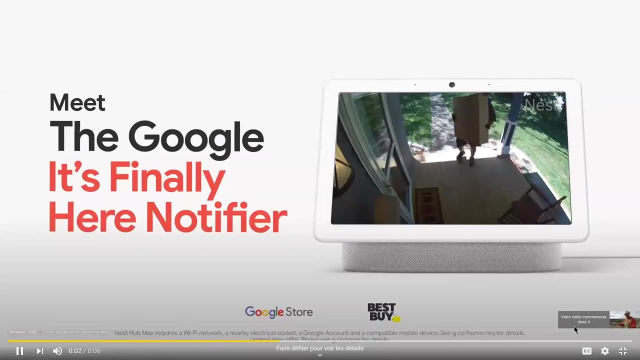 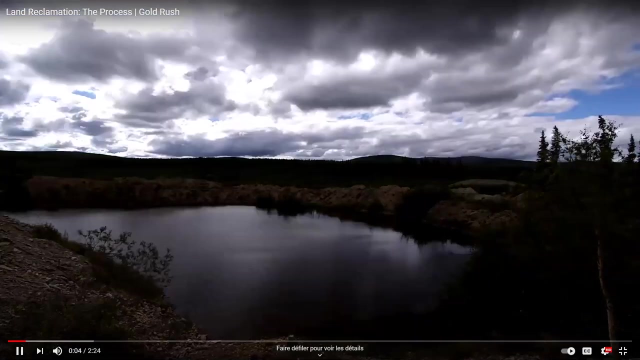 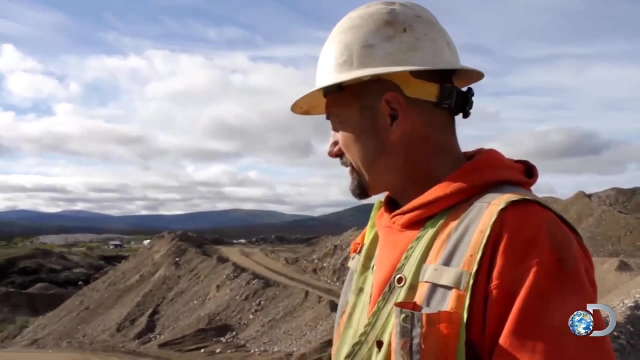 land reclamation, the process of it and the results from from it, from their work, for when your special delivery arrives, meet the google. it's finally here. notifier nest hub max from google. i know it looks bad, it looks like a big hole in the earth, but what you can't see is what we're. 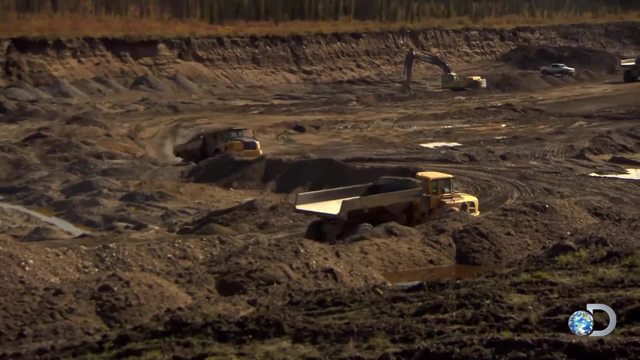 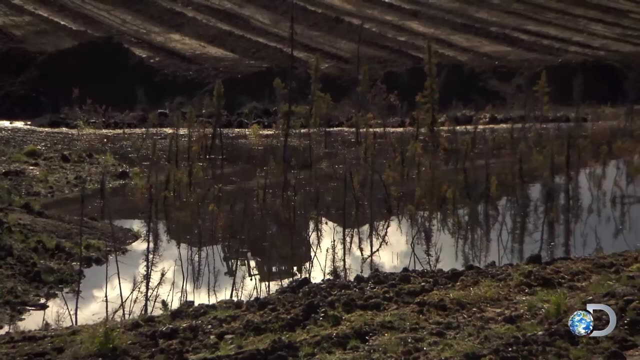 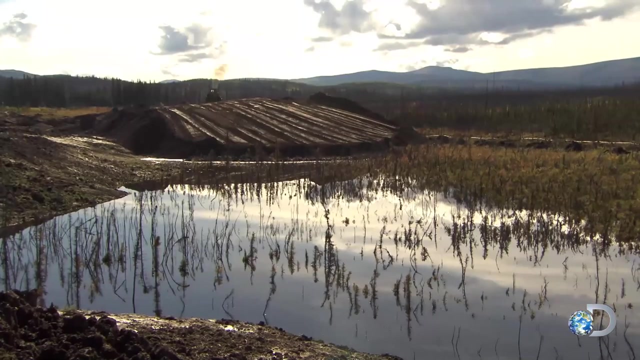 going to do. i've been a miner all my life. it's my profession and i take it seriously, and i think my dad always taught me to be stewards of the land and as you take something away, whether it's you make your business in a town, you give back to the town. if you have a relationship with people, you 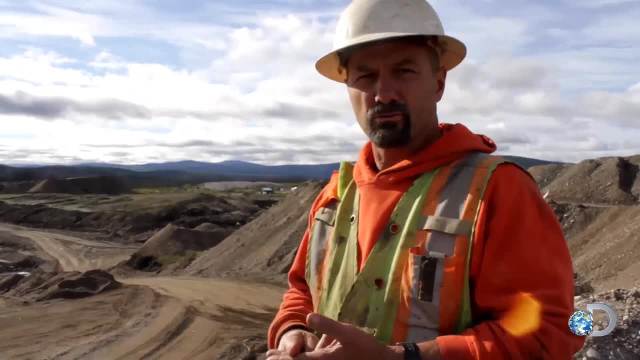 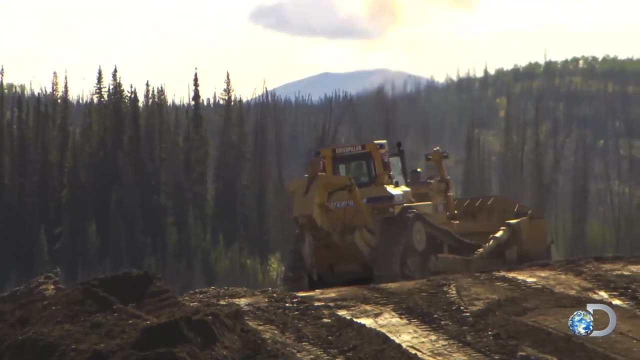 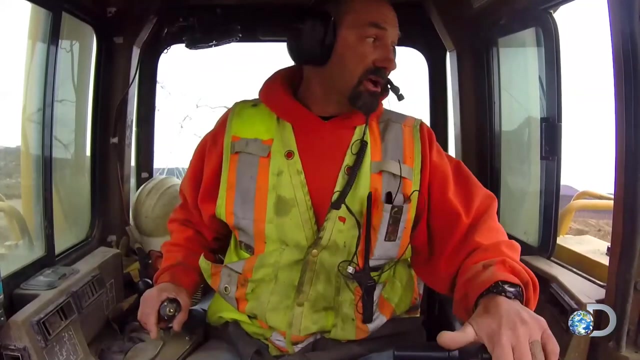 give back to the people. well, it goes the same with our earth. we take the gold out and we need to put it back. so he's always instilled that in me. good miners: as they mine, they always have the end product in mind. reclamation is expensive. every irresponsible miner that does reclamation is 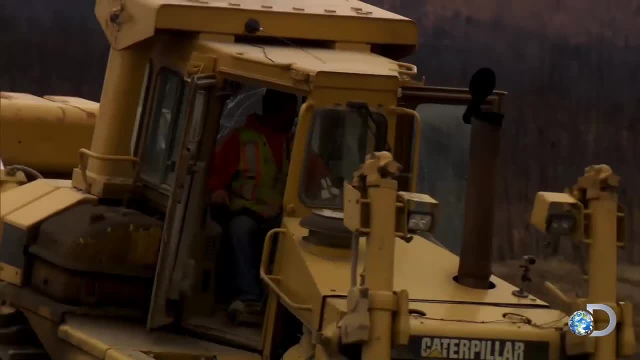 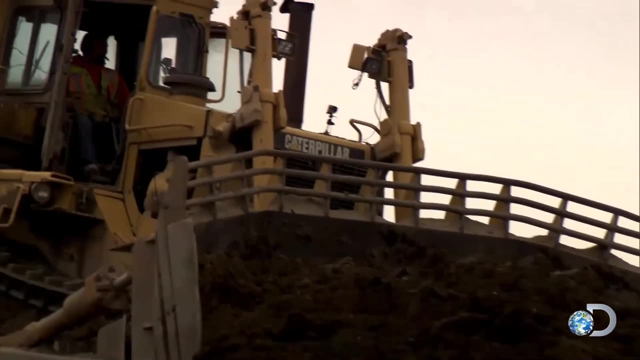 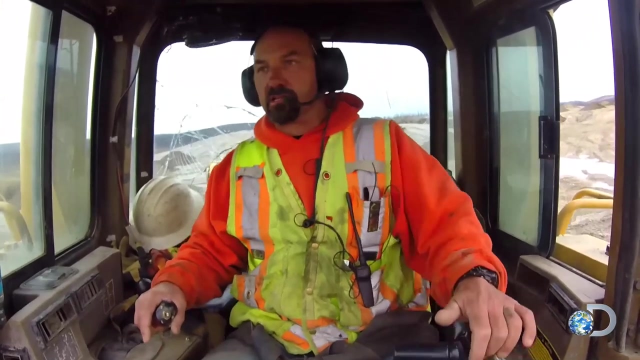 always a uh. there's always an issue between spending money that doesn't recover any costs. basically, this does nothing but cost us money. it doesn't do anything for the bottom line, but it's the right thing to do. we pulled gold out of here and this provided a living for us, and now it's 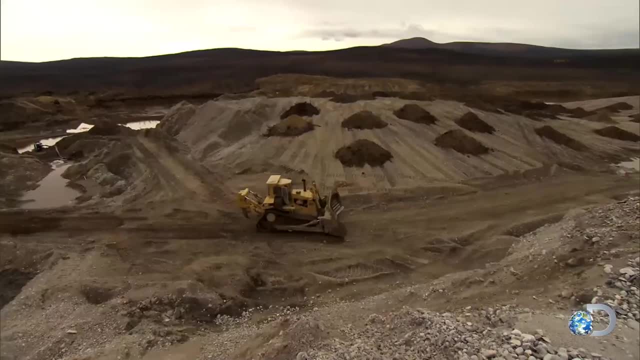 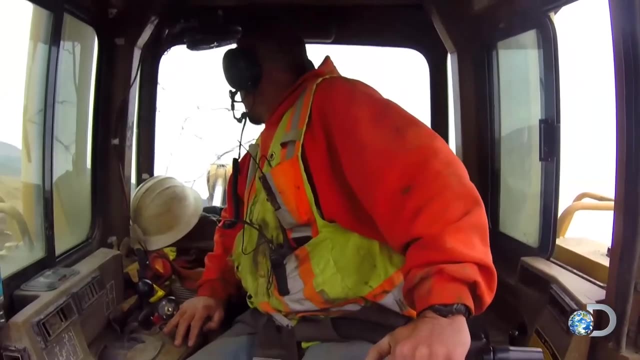 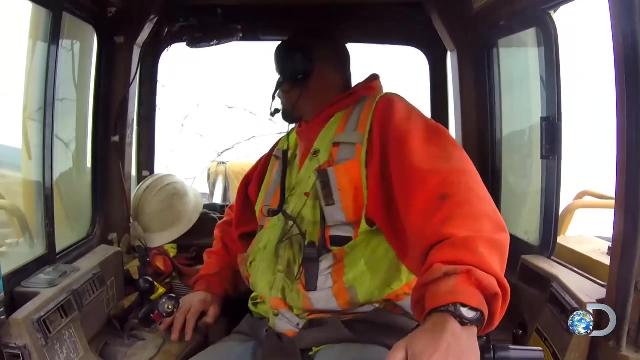 time to put something back. this top soil has everything in it to grow. it's got all the seeds, all the spores, it's got- uh, very rich compost. so this is a little bit above and beyond what we're required to do if we're just going the extra mile. 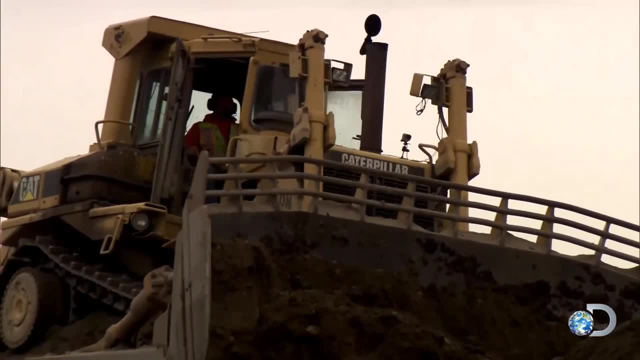 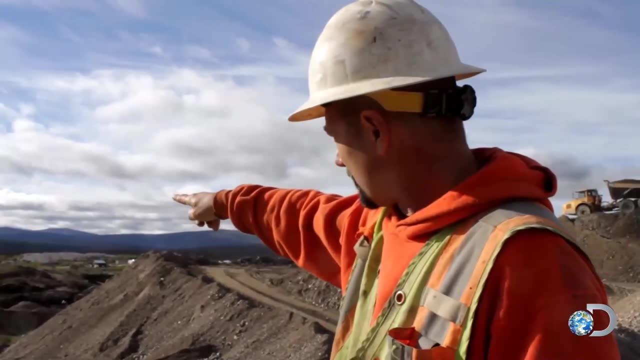 and we've kind of discovered what works around here. so the most important critical thing we can do is put the top soil back on so you can see how fast things grow. if you look over there, you can just start to see green, and that was actually in three months. three months ago we 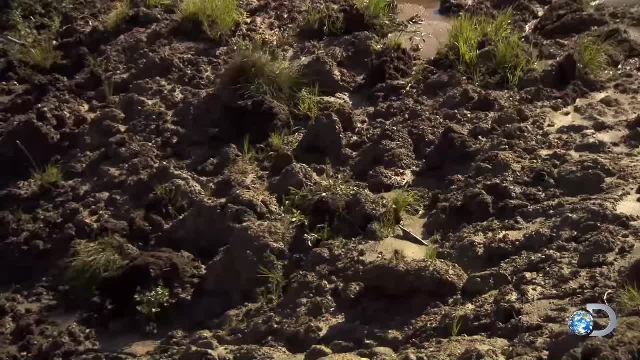 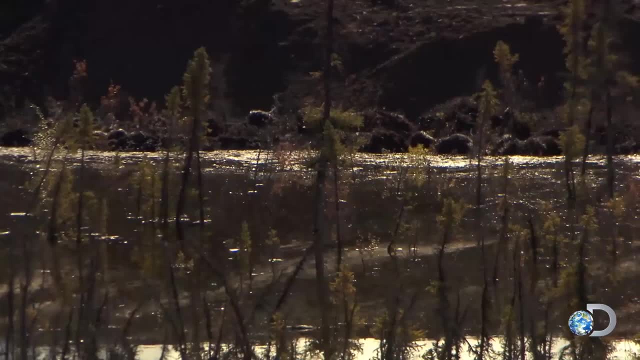 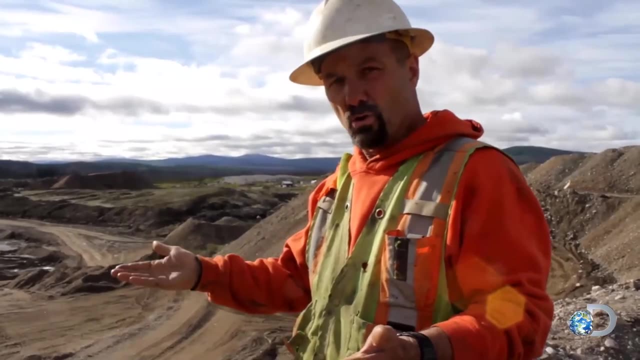 removed it from its natural state, put it up there and it's already growing. it looks looks bad now, but in uh, three years, you will never know that we mine here. they start with an end in mind, so when we started this, our end goal was to reclaim this site, so we mined it. 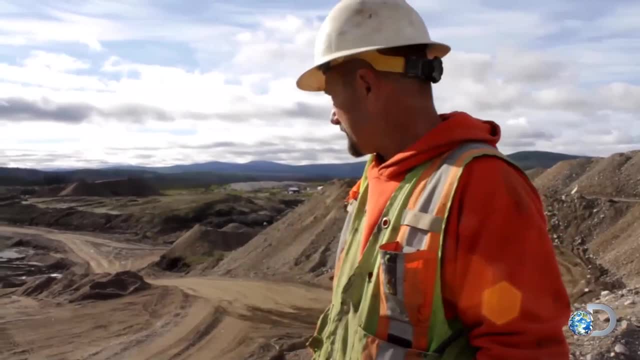 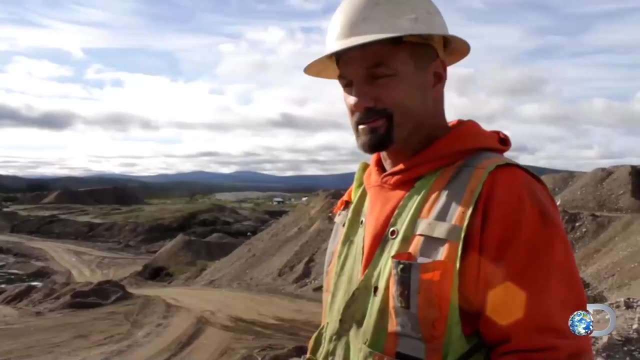 according to that plan, knowing that we're going to reclaim it. so, yeah, it's, it's true, and dear to my heart is the reclamation, so i'm glad to share it with you guys and, uh, hopefully we can see this in about three years. it'd be nice to come back, take some pictures and see what it looks like.